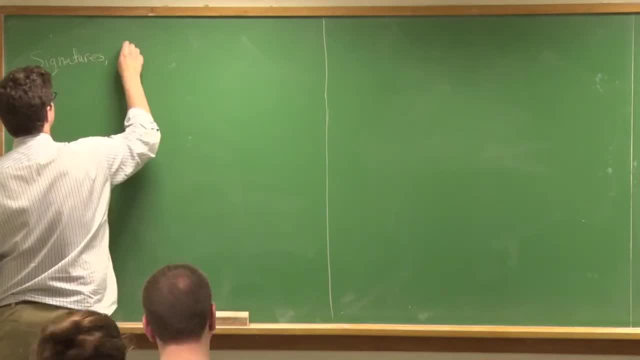 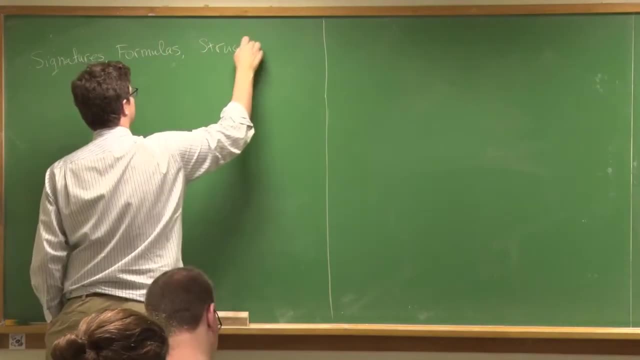 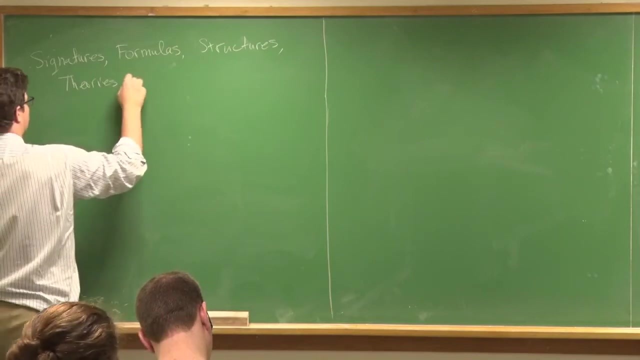 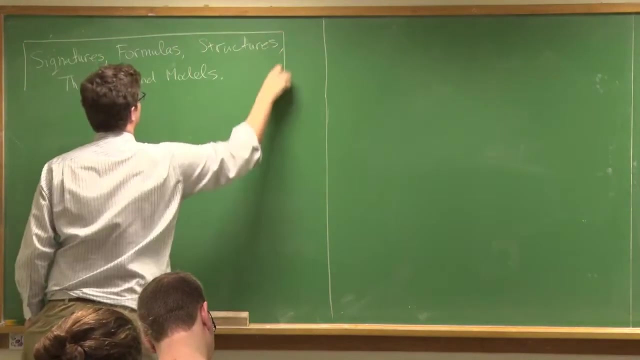 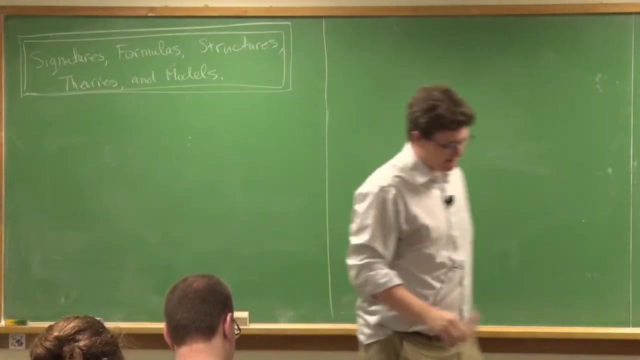 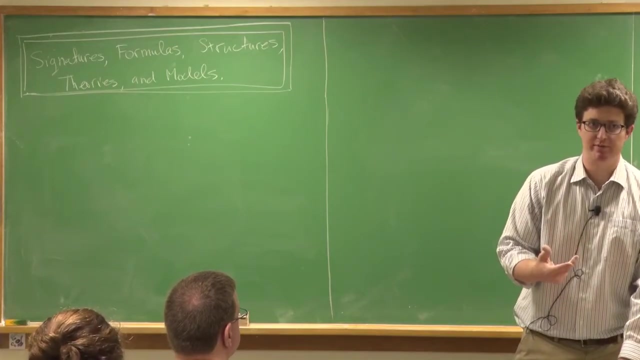 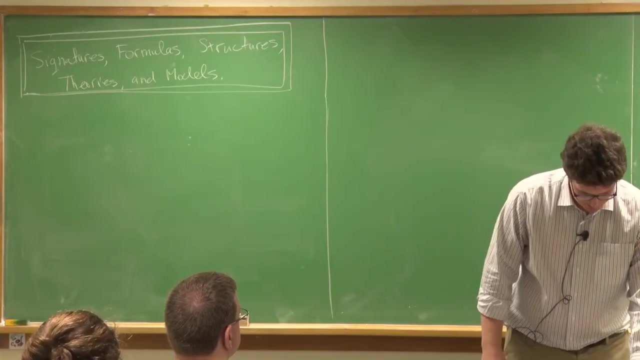 Structures, Well, signatures, formulas, structures, theories and models, And so this is kind of how we build up logic formally, Okay. Okay, And I'm using this because I want to talk about the difference between having a less than or equal to sign, with the axioms and the actual numbers, and not having a less than or equal to sign, and what this difference is technically Okay, So, so a signature. so let's start with signatures. 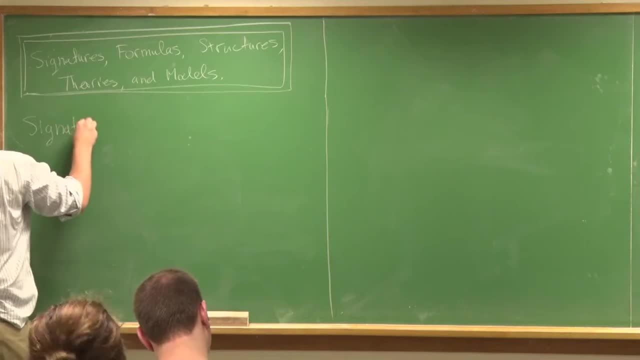 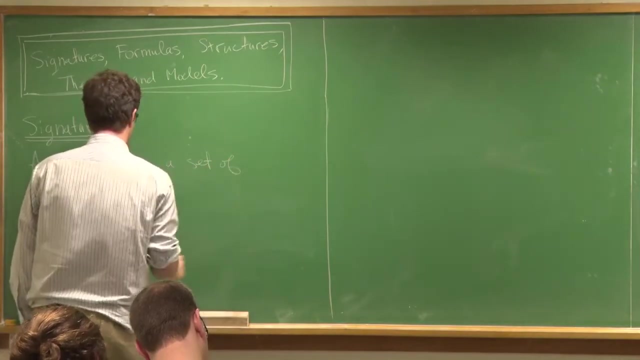 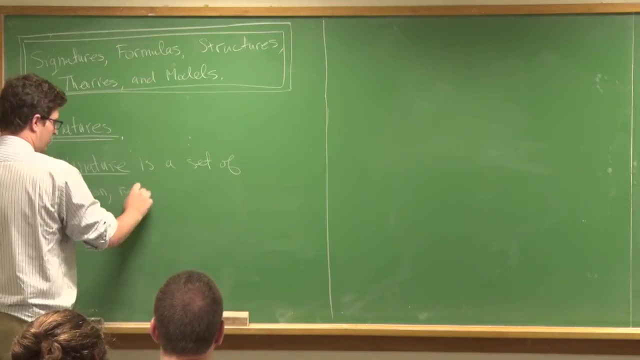 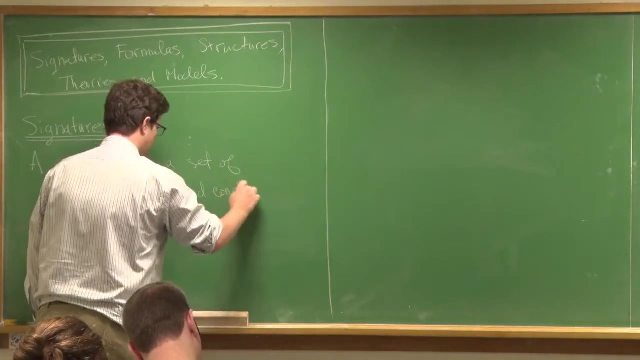 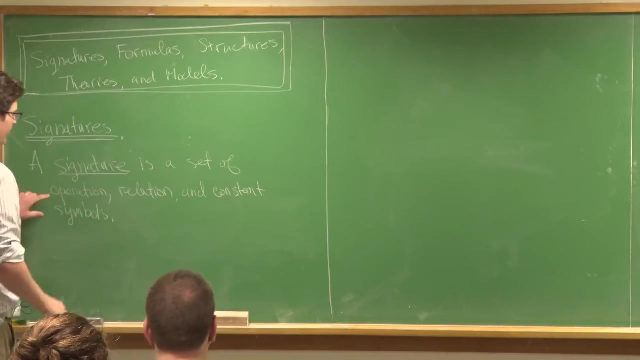 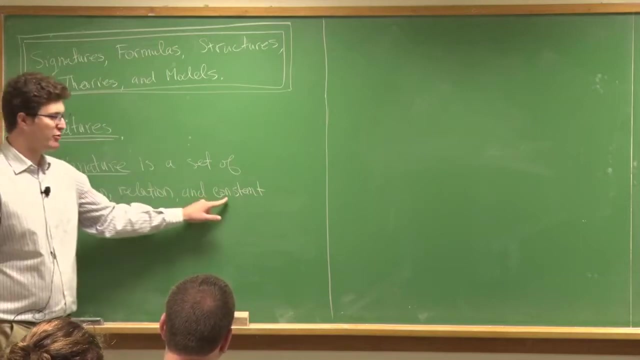 Okay, Okay So, and I'm just going to go through this, This list of things: Okay So, a signature is a set of operation symbols, operation relation and constant symbols and constant symbols. Okay So, for example, for they could be a multiplication here, or they could be like an inequality, or they could be like the group identity or the you know the identity for for multiplication in a ring. 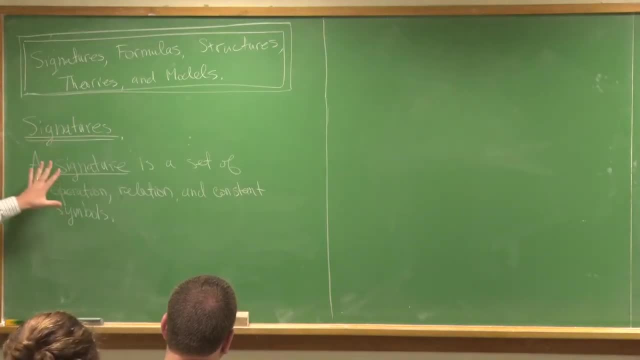 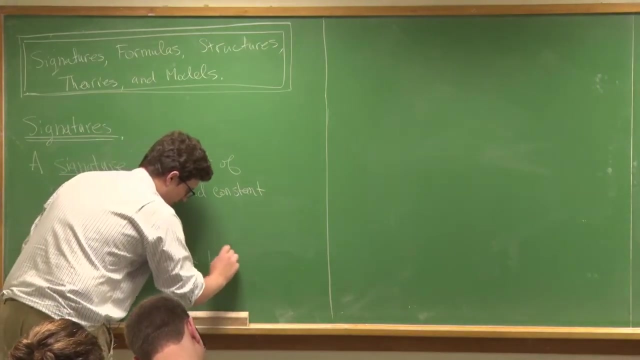 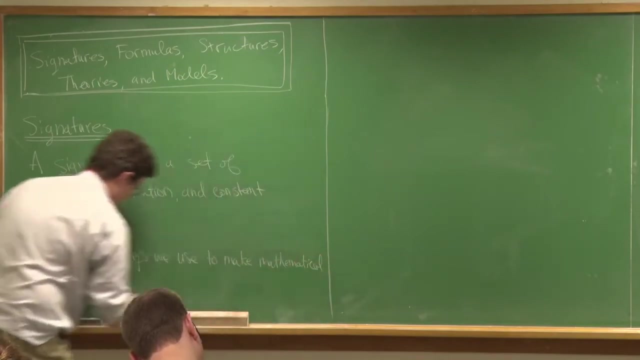 So it's the. it's the collection of things that we use to build the formulas for the formulas that we're going to use, that you know the mathematical formulas that we're going to use. So these are the collection of things we use to make mathematical formulas. 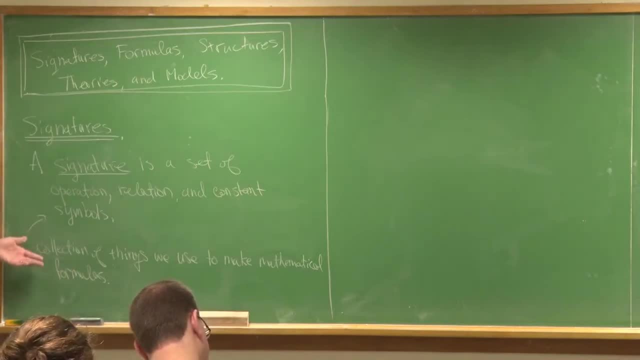 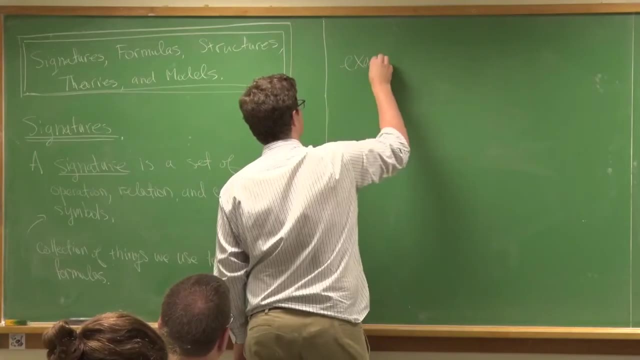 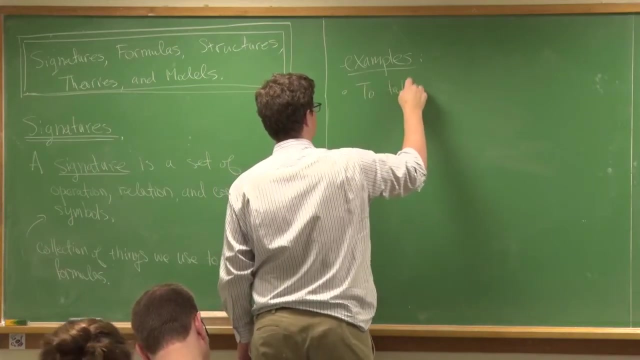 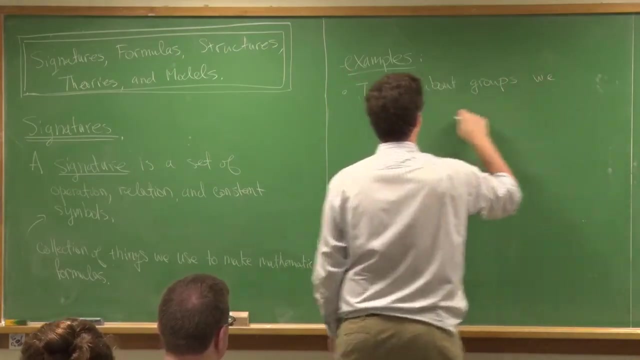 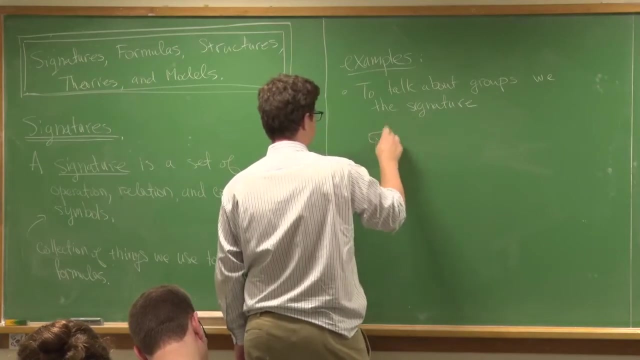 Okay, Not including the quantifiers. So the quantifiers, parentheses and equal signs will be given. Let me give you some examples. So, to talk about groups, we use the signature And I'm going to use, I'm going to call this sigma. 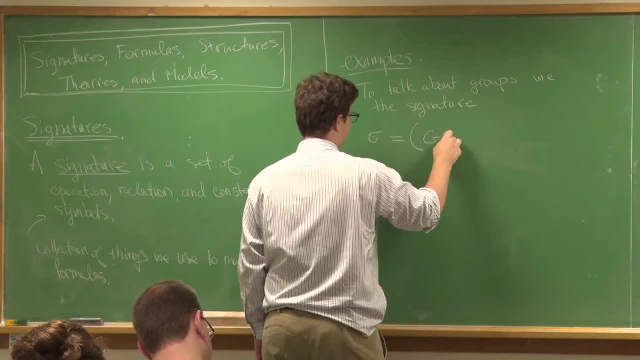 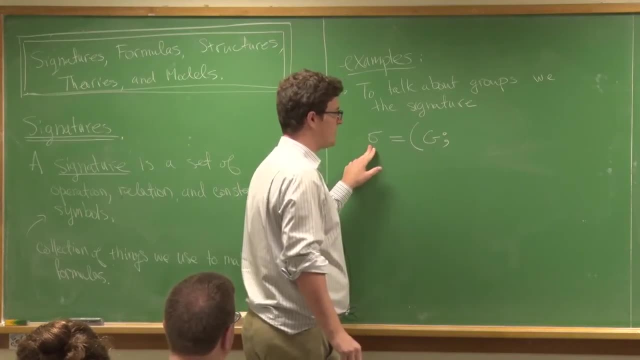 And then I'm going to use the underlying thing here. So sometimes this is called a sort, but I'm going to include this in here. So groups: we just have two symbols that we really use. We have a multiplication symbol, so that's our binary operation. 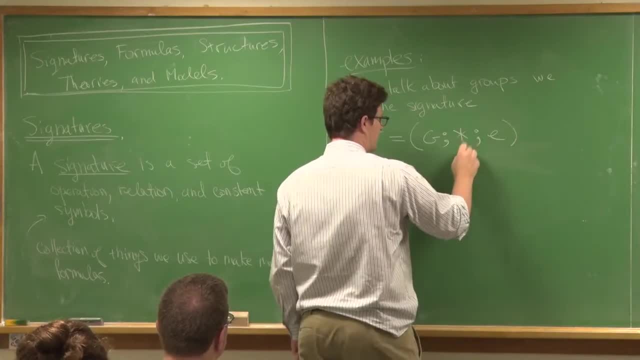 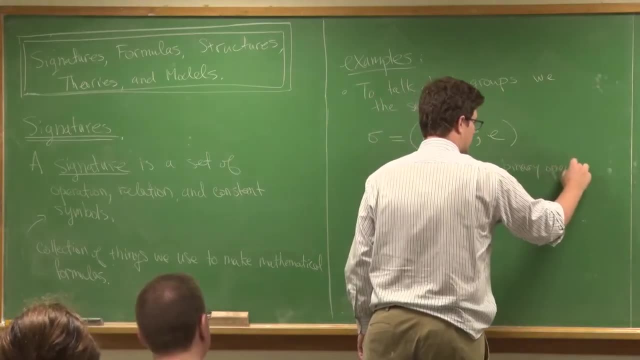 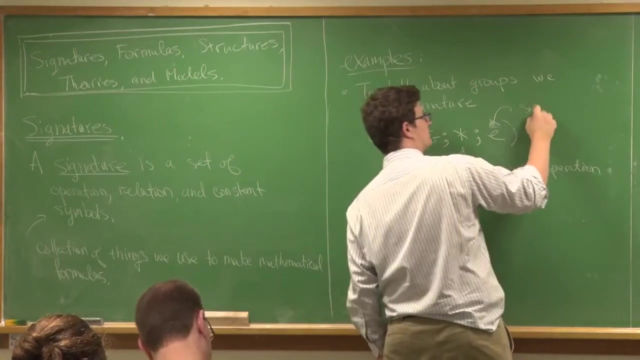 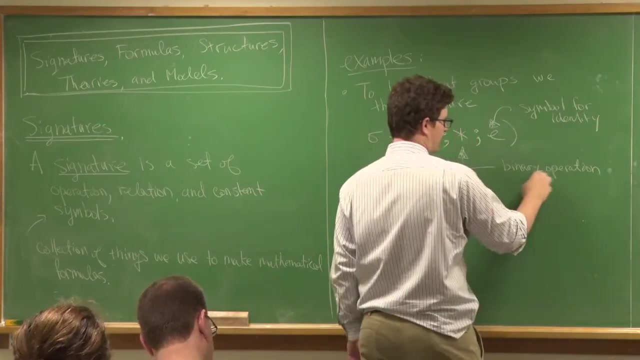 and then we have our constant symbol. There's no relations in this one. So this thing here is our operation, This is the binary operation, our symbol for the binary operation, And this is the symbol for the identity. So this is an operation symbol and this is a constant symbol. 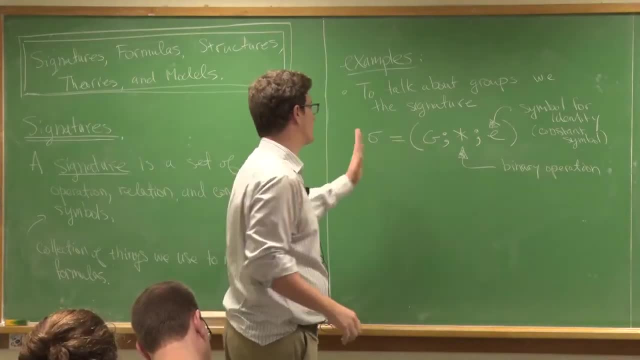 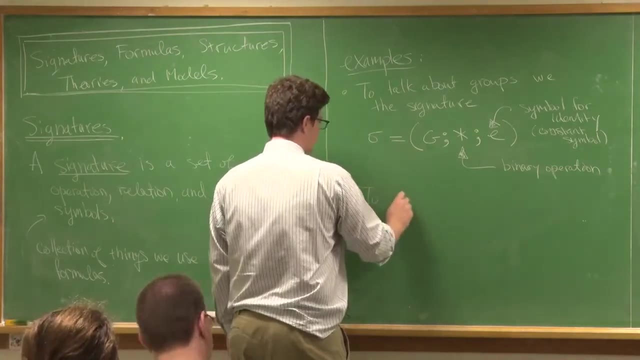 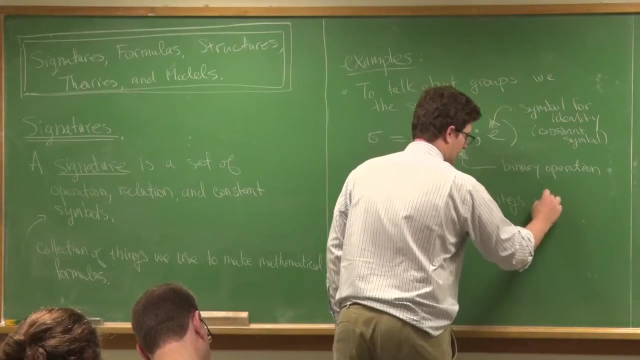 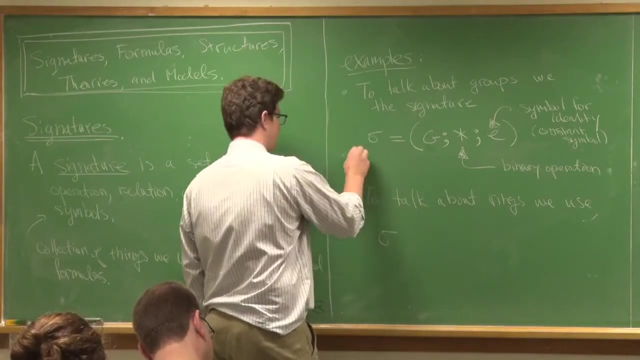 Okay. and then this is just an underlying set or sort Okay, so it's like a symbol we use for the thing. So let me give you another example. To talk about rings, we use the following: this signature: This is the Greek letter sigma. by the way, 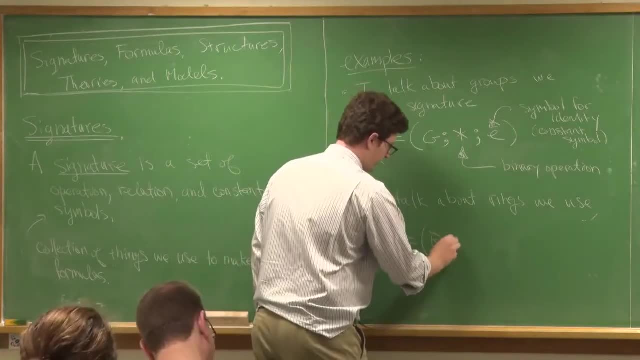 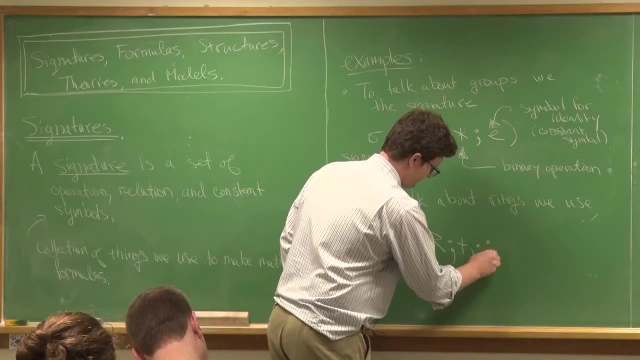 So we use the signature where we have this ring, the ring sort, and then we have an operation of addition, We have the operation of multiplication. There's no relation symbols, There's nothing like less than or equal to. We have a ring and we have a ring. 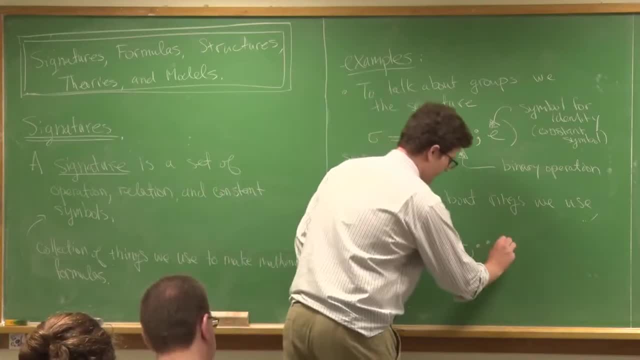 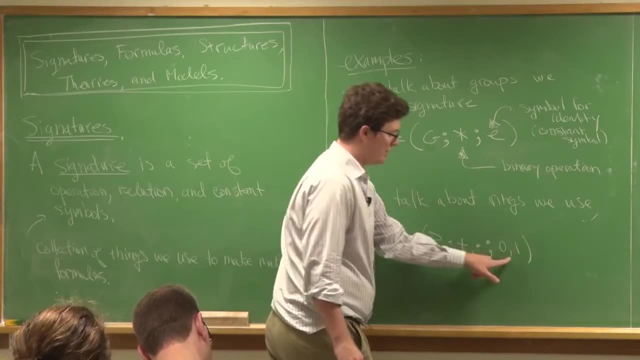 We have the free relation symbol, equal sign, but we don't write that one down right. And then we have zero and one. okay, So here are our function symbols, our operation symbols, and then here are our constant symbols. all right, 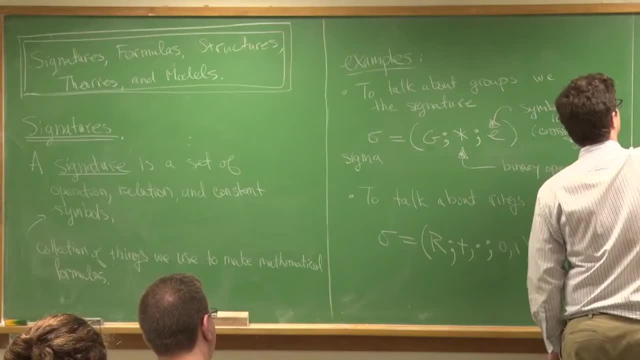 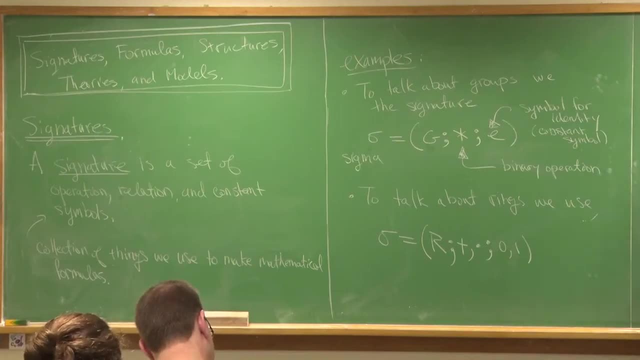 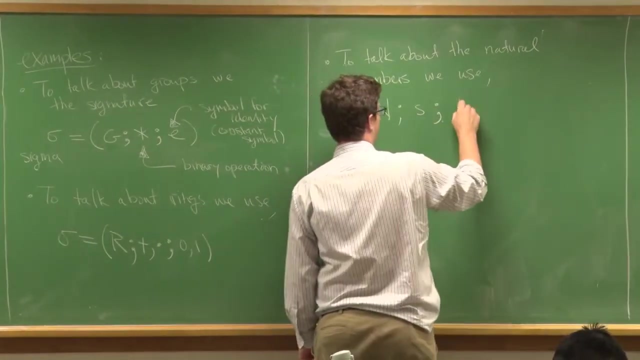 So to talk about the natural numbers, here are the natural numbers. So in the Datakn-Piano, for the Datakn-Piano we use this natural numbers here. and then we had this function. This was our successor function and then we had either one or zero. 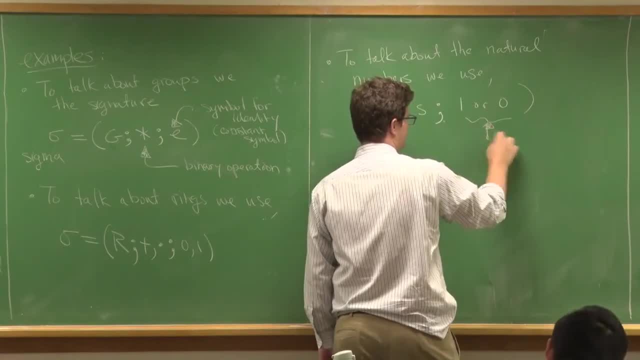 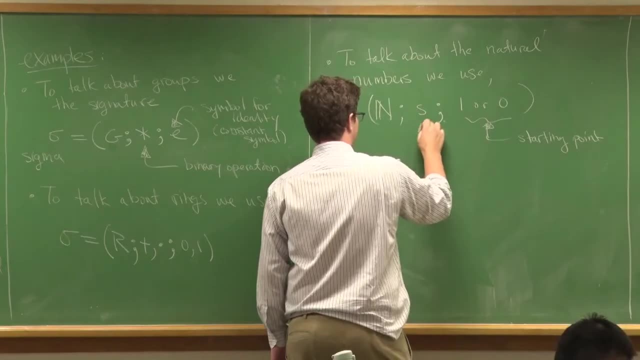 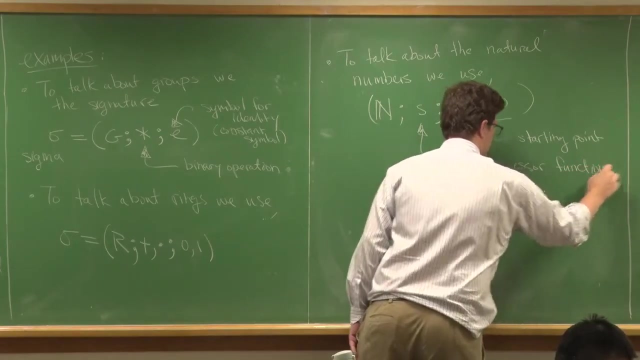 and so this thing here was our starting place. So this is the constant symbol which is our starting point. All right, and then this was the successor function. Okay, and so this was a function which takes the natural number and it returns a natural number. 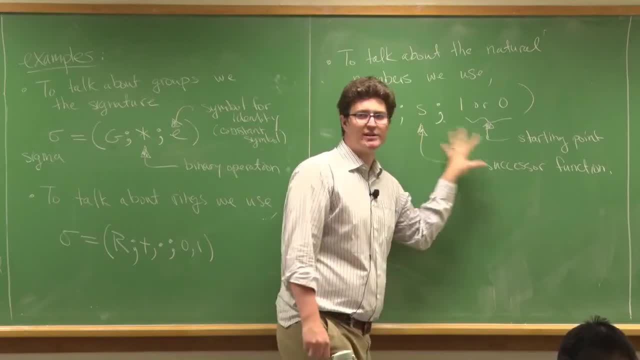 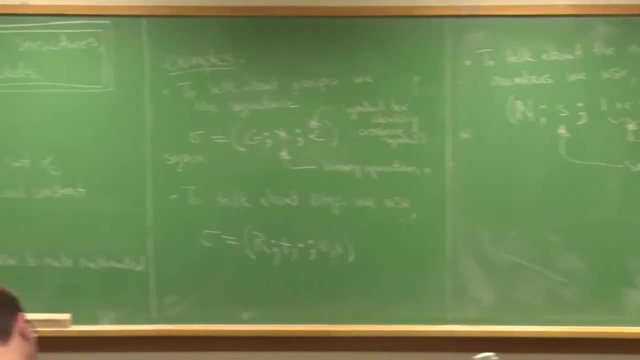 and the idea was that it would return n plus one, But right now we're not assigning the meaning, We're just making symbols for them. okay, So these were the signatures. okay, So let me talk about formulas. So let's talk about formulas now. 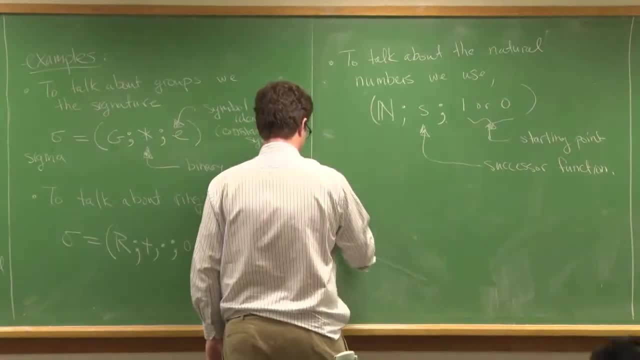 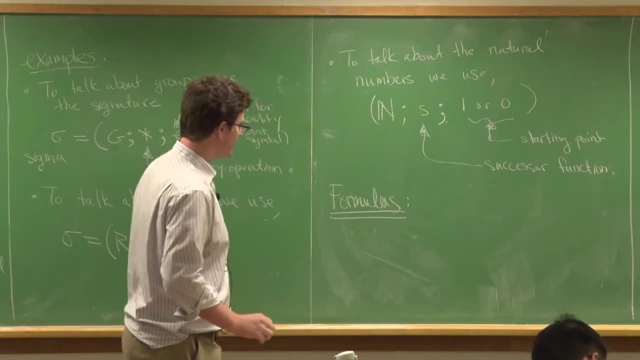 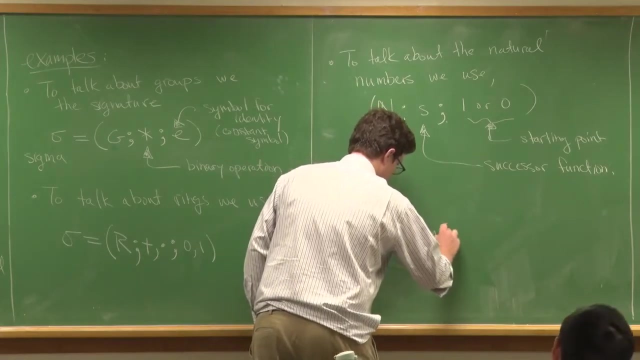 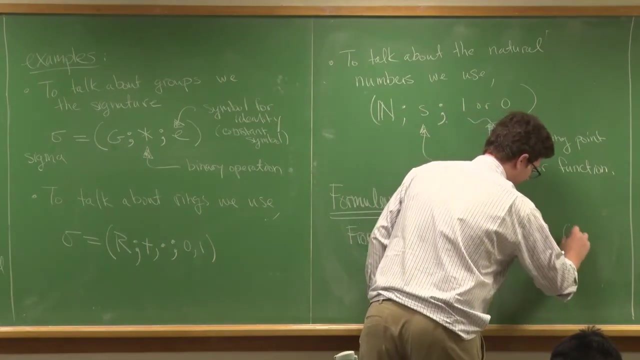 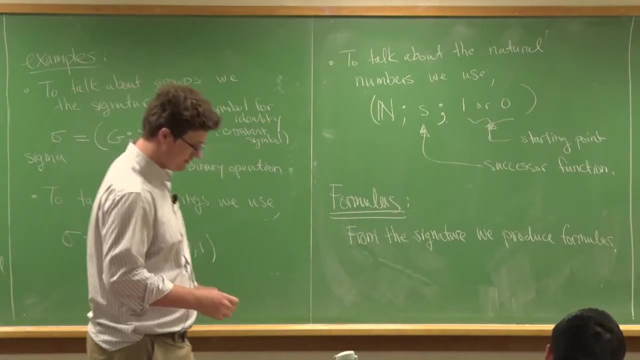 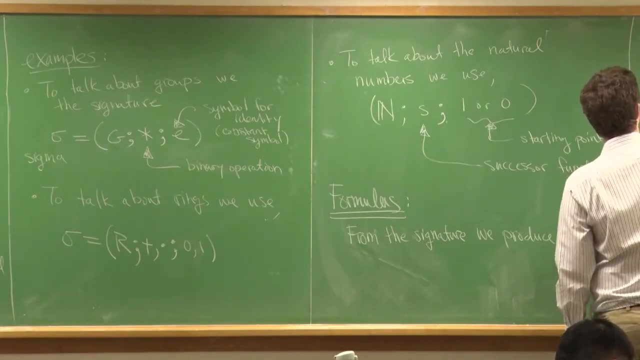 So for formulas, Okay, so for formulas. so from the signature we produce formulas, Okay, And the formulas are Okay. so let me just give you the idea. So the signature, We have formulas here. okay, So in the signature, right. 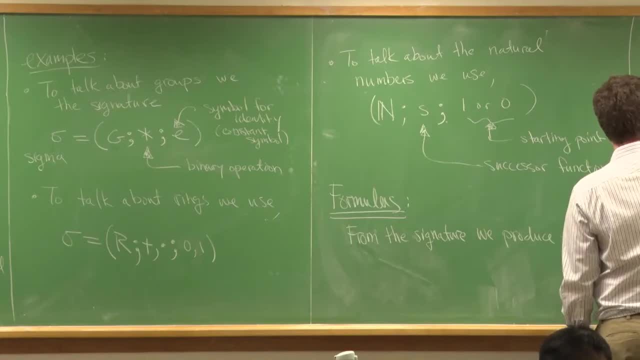 we could have something like the group multiplication, multiplication and then the identity axiom, and then from that we could produce formulas. So formulas, they have variables in them for all x, y. Let me just start one. This is like: x is equal to y times z. 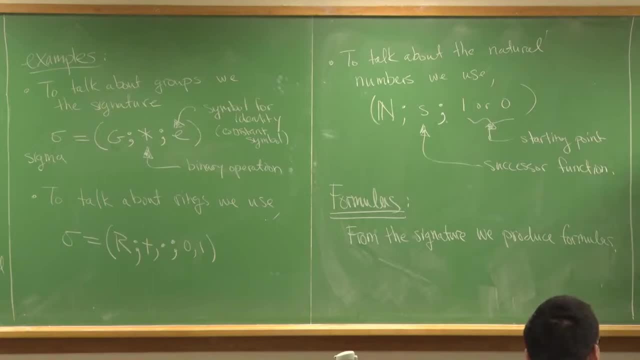 So these are with free variables. This is an example of one. Or you could have something like: for all x there exists a y, such that x times y is equal to e. Or you could have something like. that doesn't necessarily have to be true. 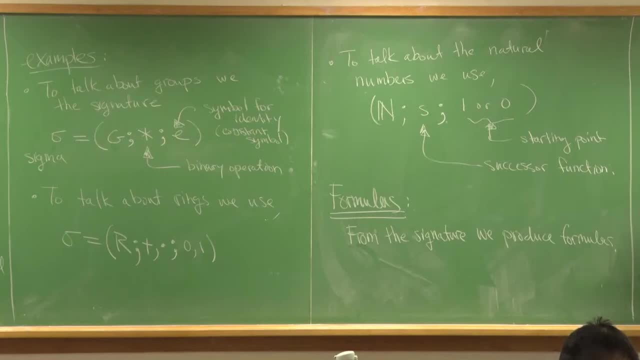 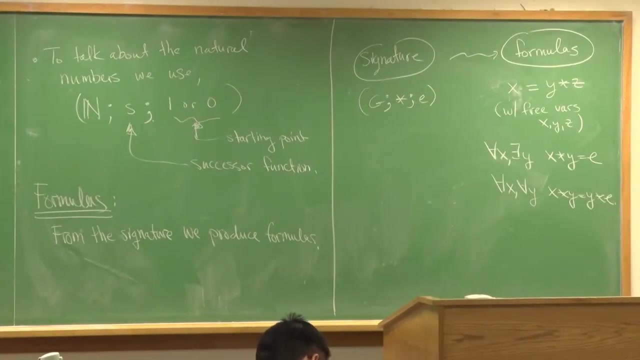 for all x and all y. x times y is equal to y times e. Okay, So these are some examples of formulas that we have. They don't necessarily have to be true for groups or anything. They're just things, right, Okay. 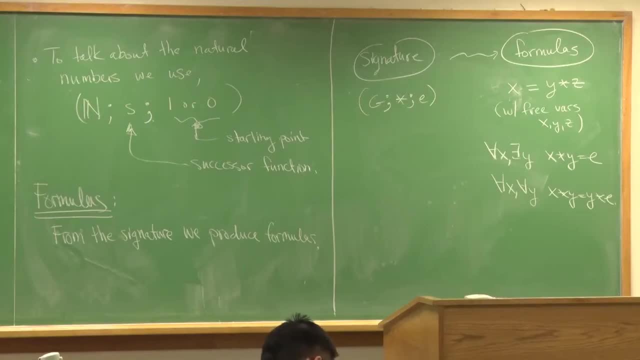 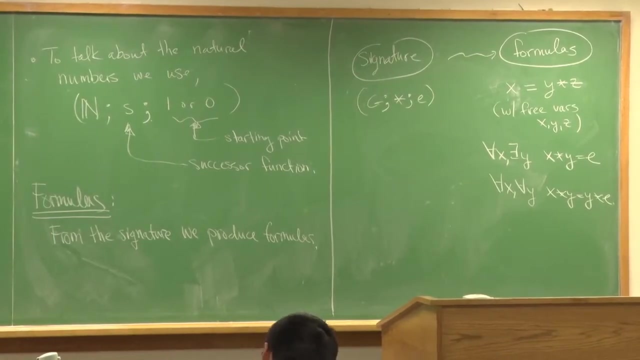 So Okay, And so we're. like I said, we're allowed to use equal signs and parentheses how we want, So I'm not going to include those in the signature of the things that we're allowed to say. So, but the basic idea right, is that for to build formulas, how formulas are built. 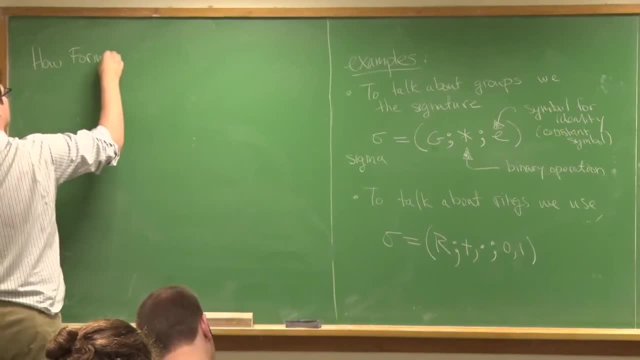 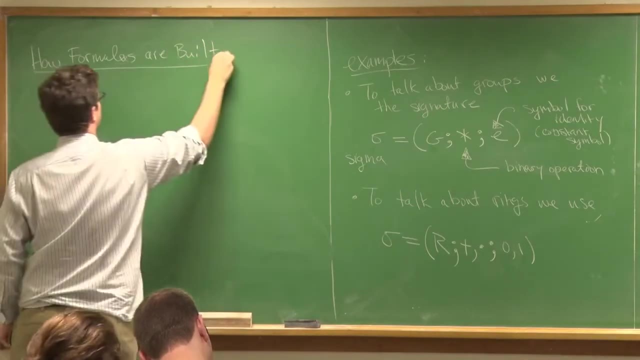 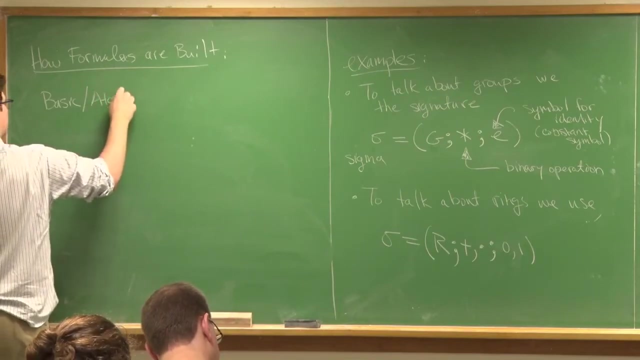 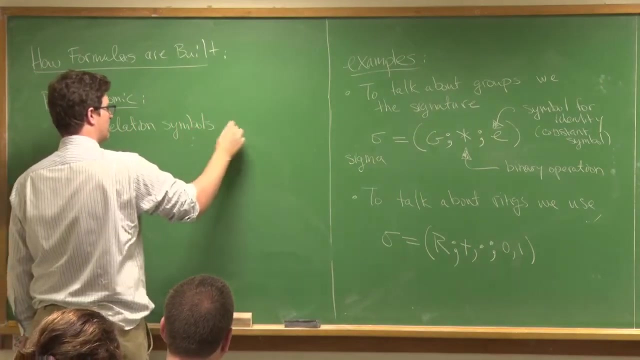 So how are built? Right, So you start with basic formulas, basic or atomic formulas, right, So these are come from basic inequalities, you know? so relation symbols by themselves, like r of x, y or x is equal to y, right? 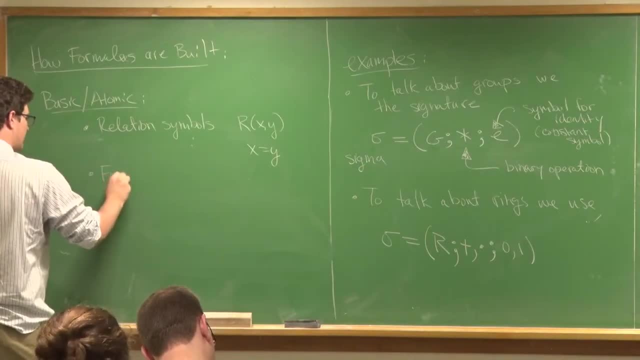 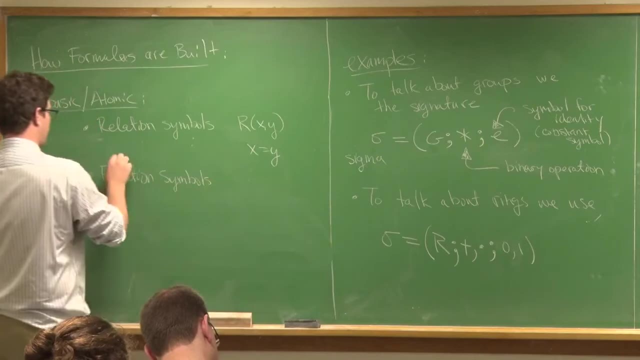 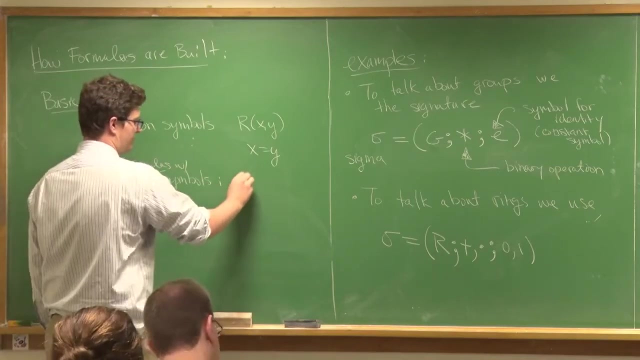 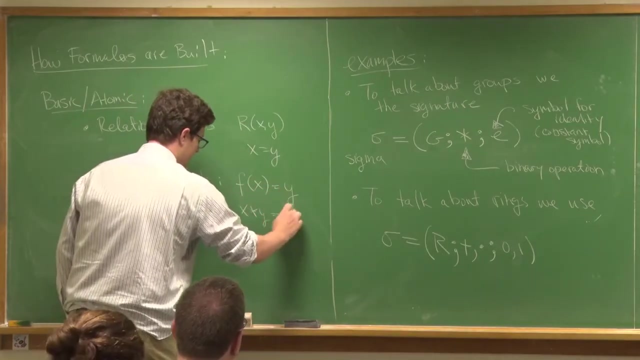 Or function symbols, with you know formulas with basic functions, The function symbols. so you could have something like: if so, here f of x is equal to y, or x times y is equal to z. So here I should mention that you know r, f. 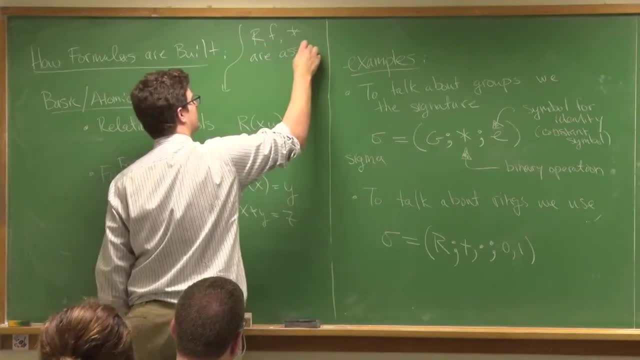 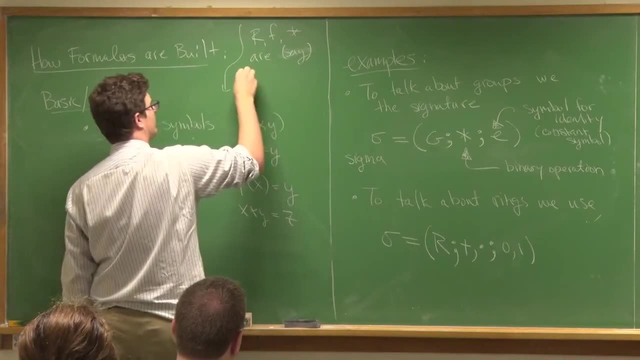 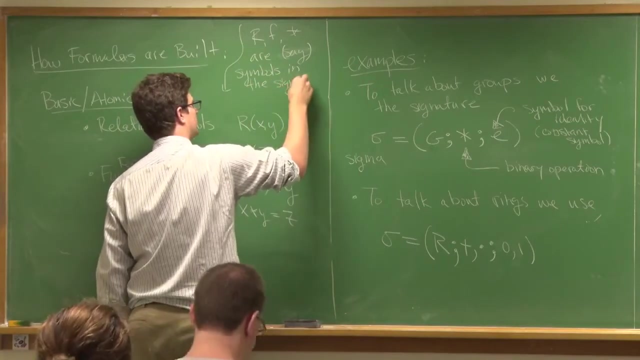 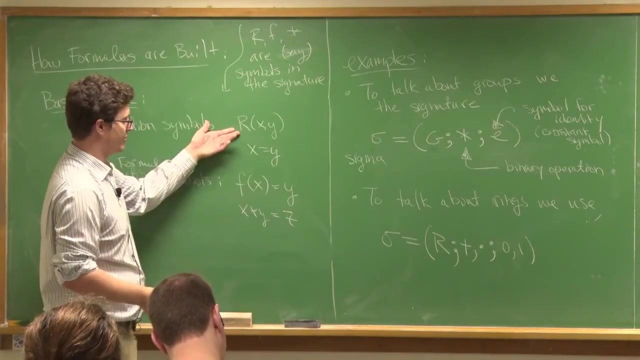 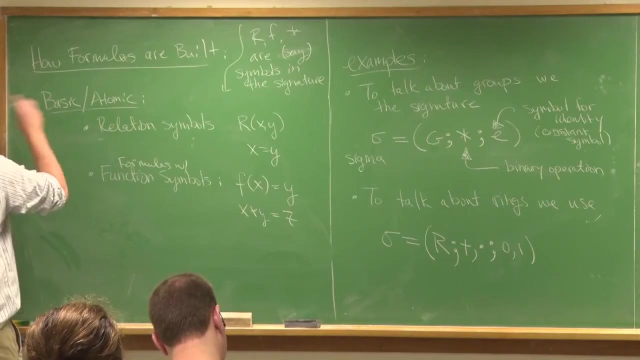 times are assumed or say, symbols in the signature. So we can start with a basic relationship. If we have a relation in our signature, we can start with a basic formula like this, And then you go from this, from basic ones, to more complicated ones. 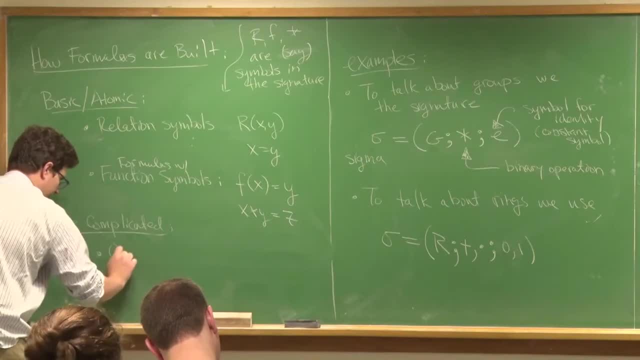 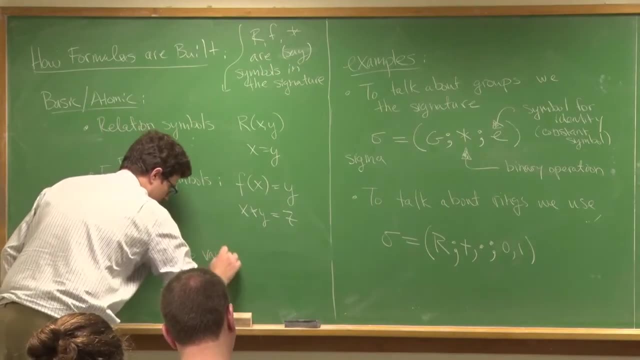 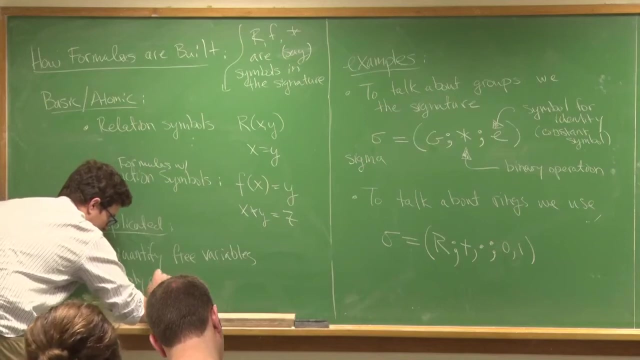 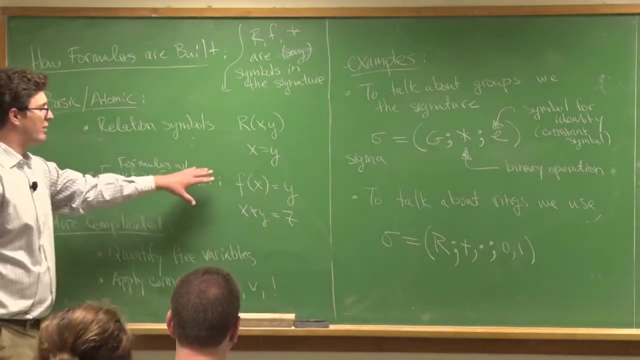 So taking basic ones, and then you can quantify free variables or you can apply connectives. So connectives are the things like and or and not. So if I have a basic one like this one or this one or things like this, I could take this and this. 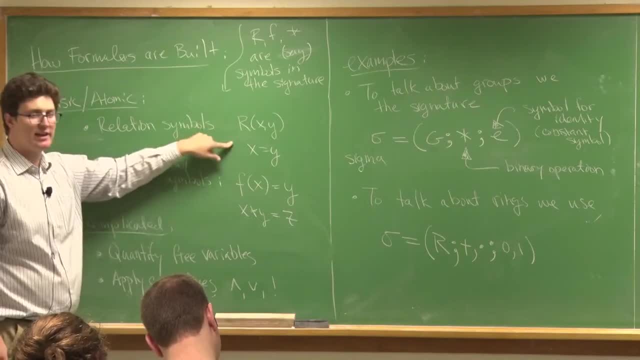 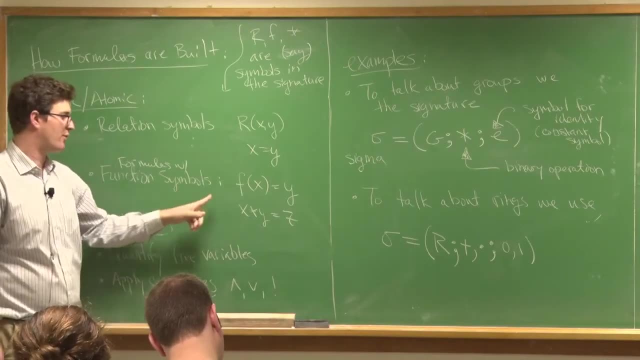 or I could take this and this or this, or this or not, this and this, Or I could say: for all x, y there is y times. for all x, x times, y, y is equal to z, things like that. 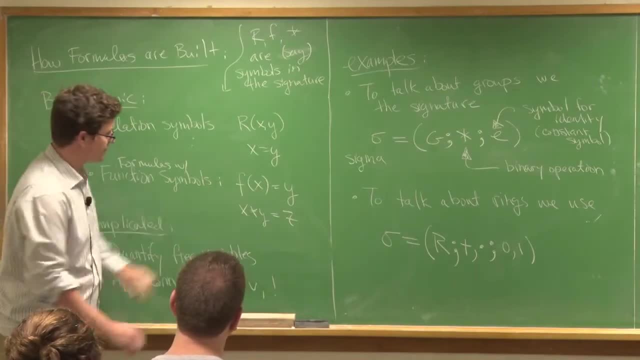 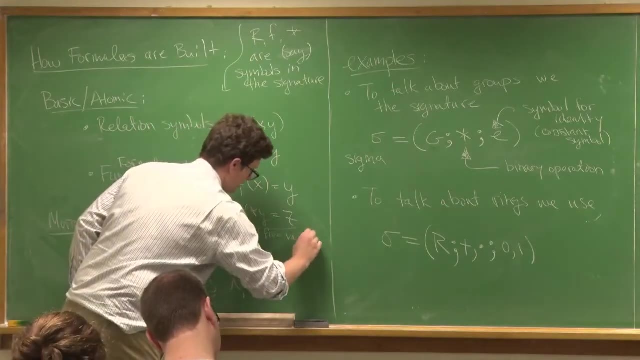 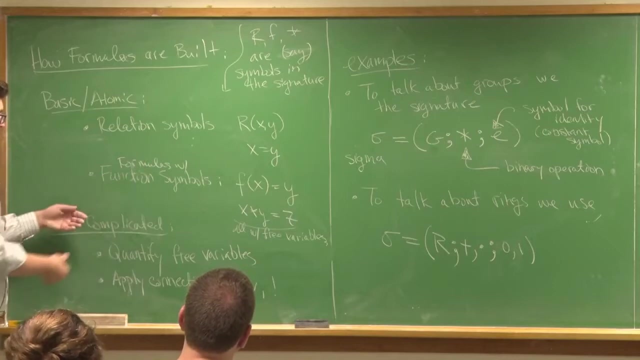 So I could these things have free variables here. These are all with free variables, free variables. So to build up all the possible formula, I start with these basic things and then I apply connectives and quantifiers to get all other formula. 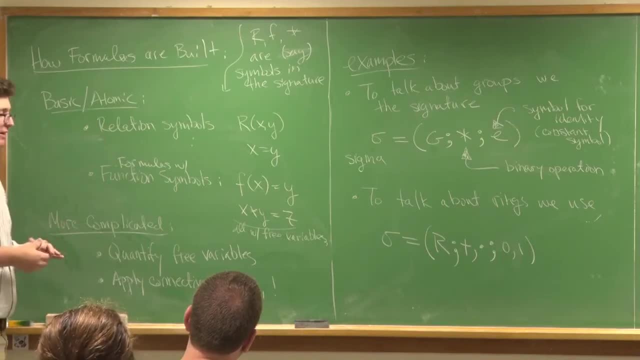 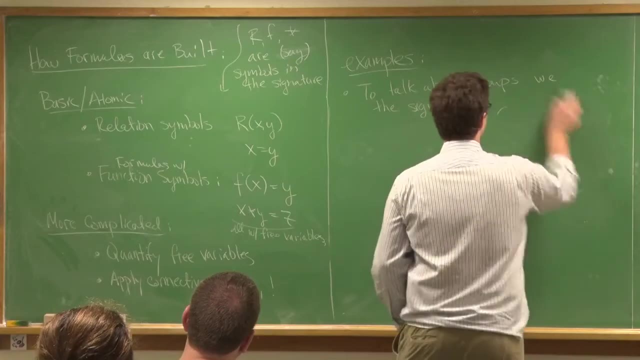 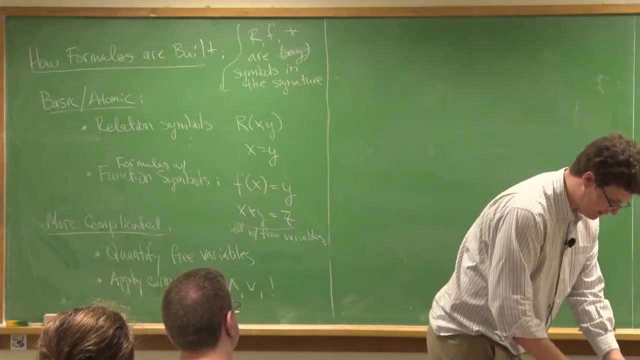 And so I generate all my formulas in this way. OK, So let me make a small distinction here. So sometimes we allow formulas which are first order and some formulas which are second order. OK, so let me just clarify what this means, Right. 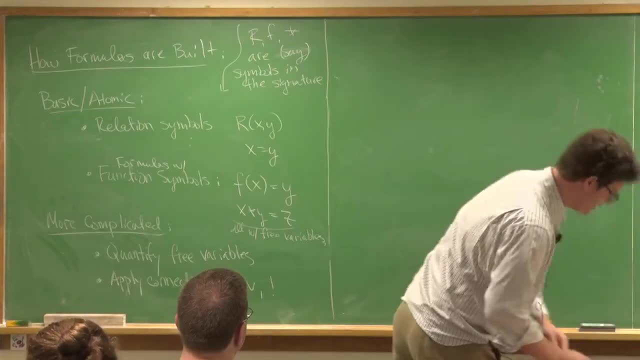 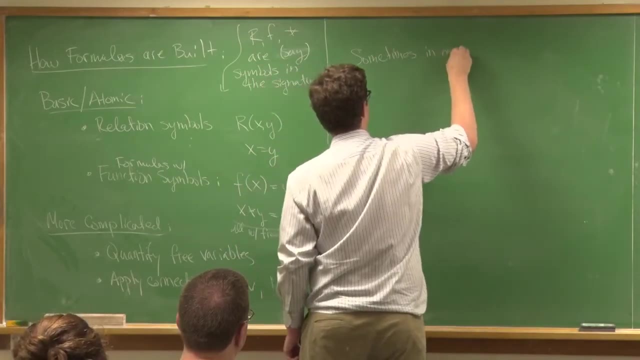 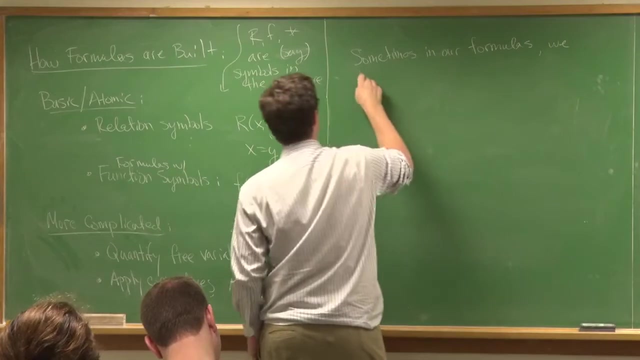 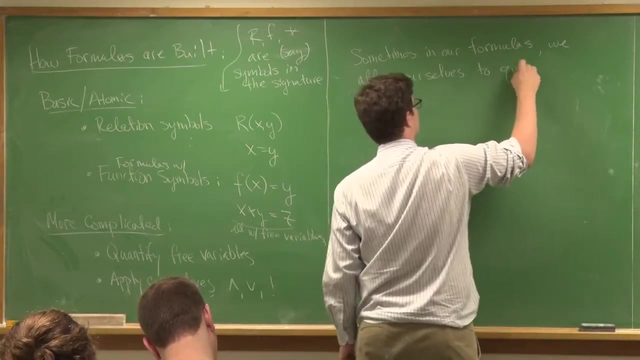 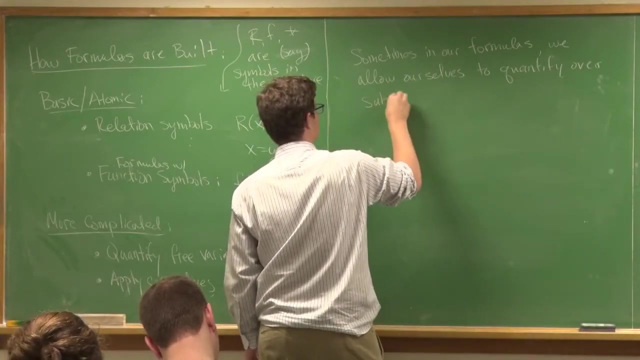 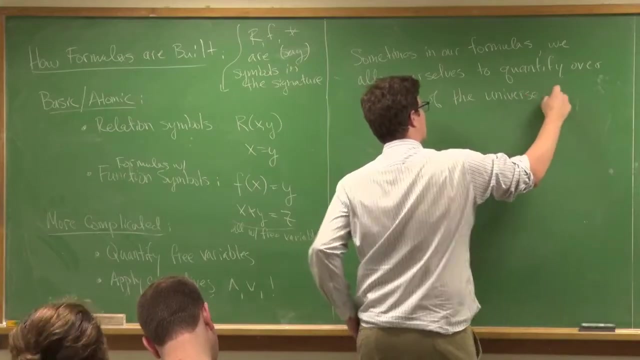 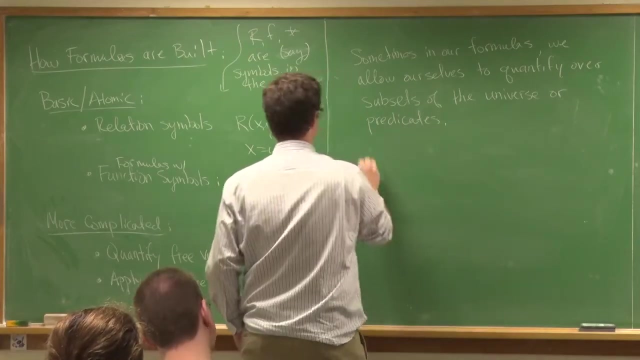 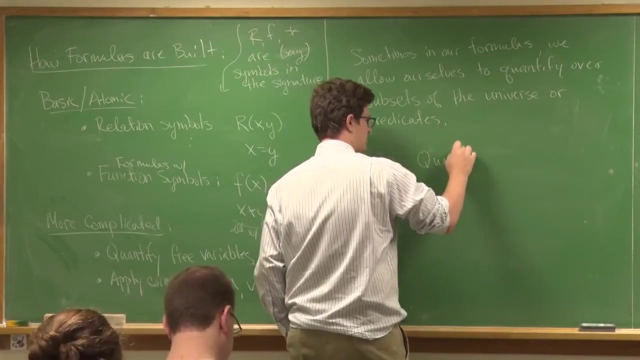 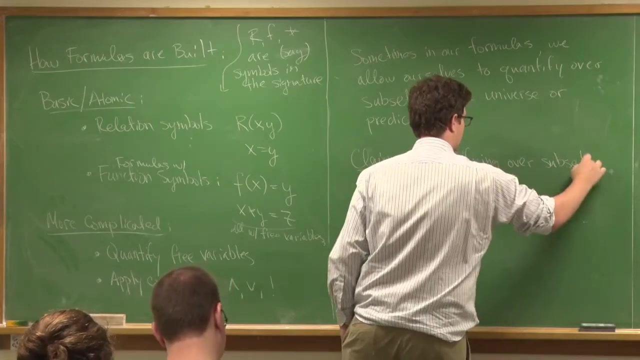 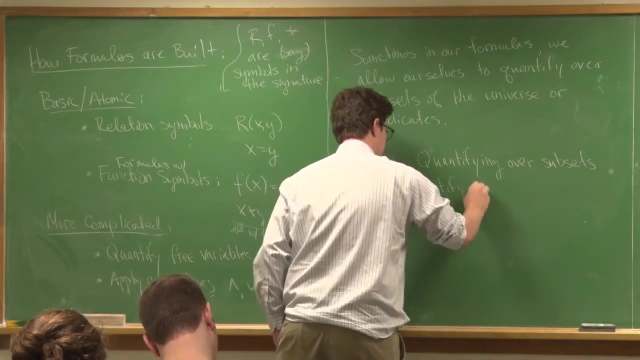 So OK. so sometimes our formulas, we allow ourselves to quantify over subsets of the universe or predicates, OK, So my claim is that quantifying over subsets and quantifying over predicates, OK. So my claim is that quantifying over subsets and quantifying. 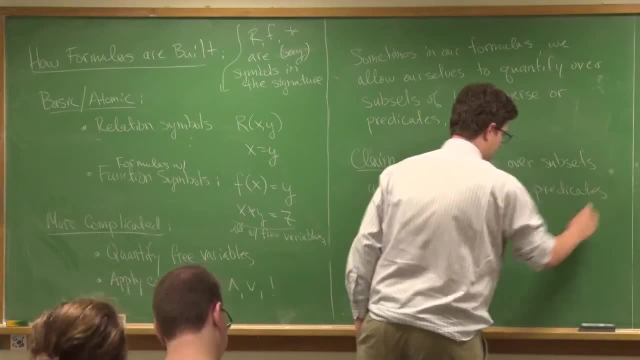 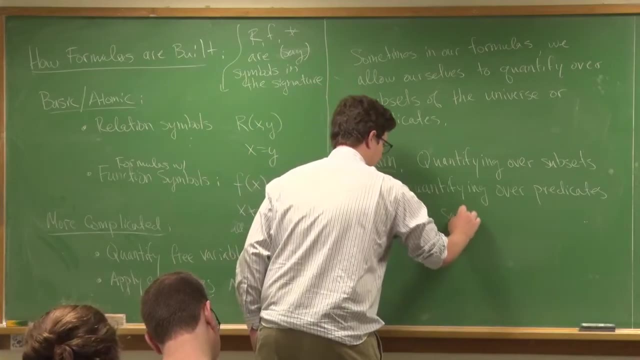 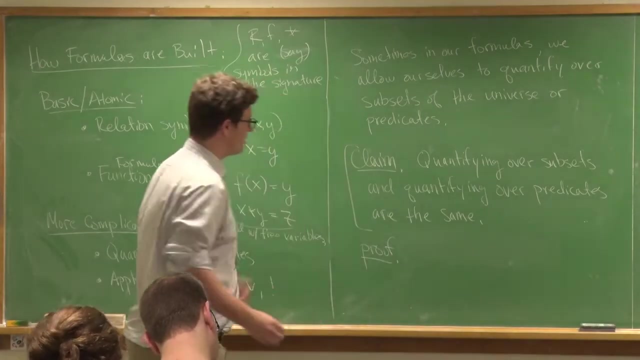 over predicates, OK. So my claim is that quantifying over predicates are really are the same thing. it's the same thing, are the same, OK. So let me give a proof of this. So if we quantify over predicates, so if we're given a predicate, so this is just. 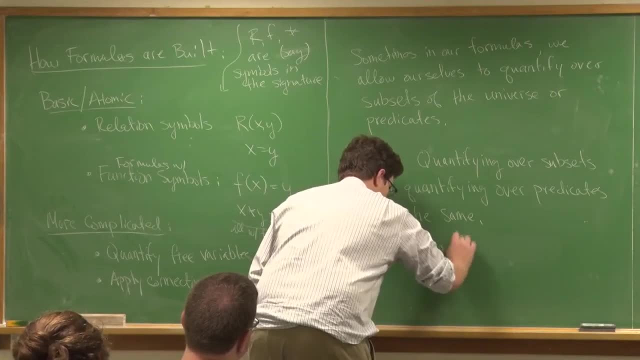 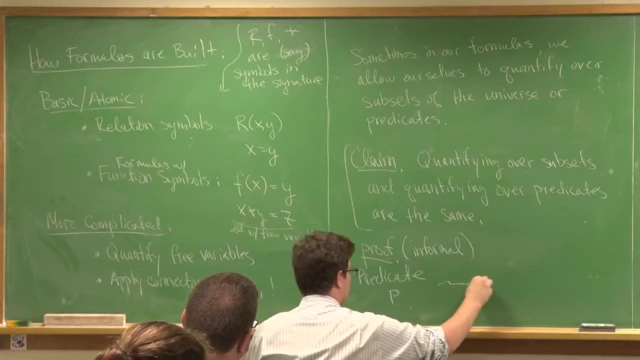 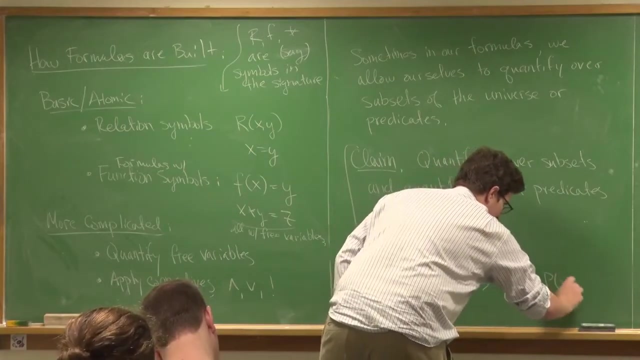 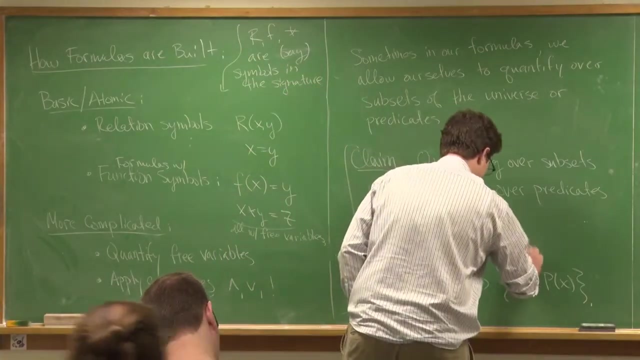 going to be like an informal proof, right? So, given a predicate, We can do P, right, We can do P of x. We can form the set of x such that P of x, OK. So from a predicate you can create a subset, OK. 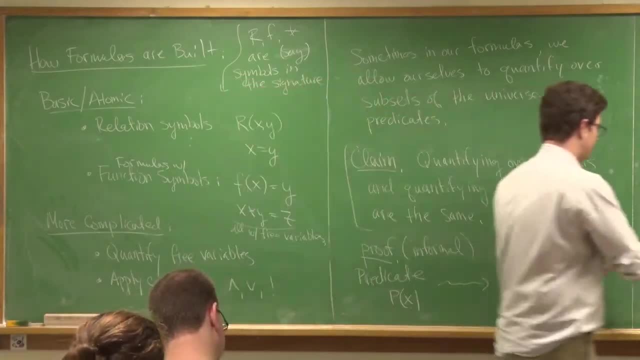 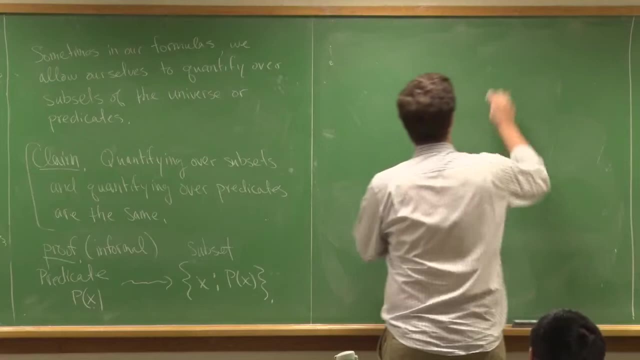 Subset of the universe, OK. Similarly, if you're given a subset, So if you have a subset, OK. So if you have a subset, OK. So if you have a subset, OK. So if you have a subset, So if you have a subset. 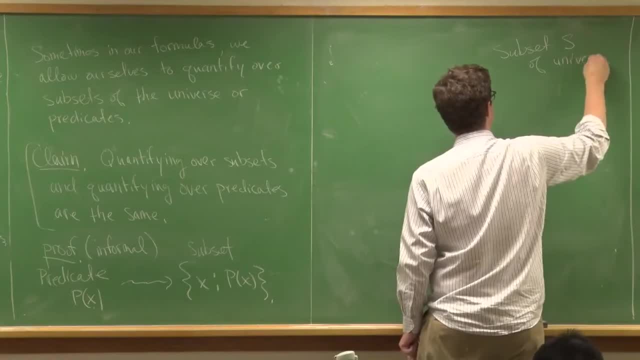 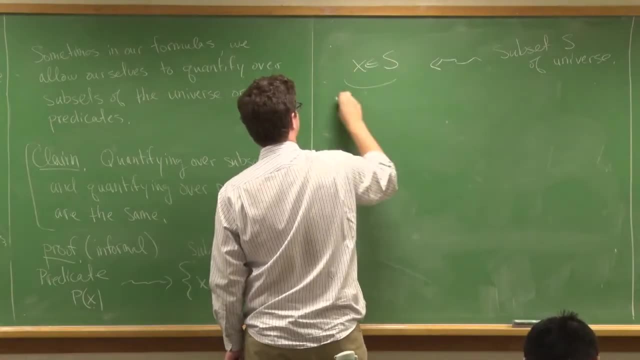 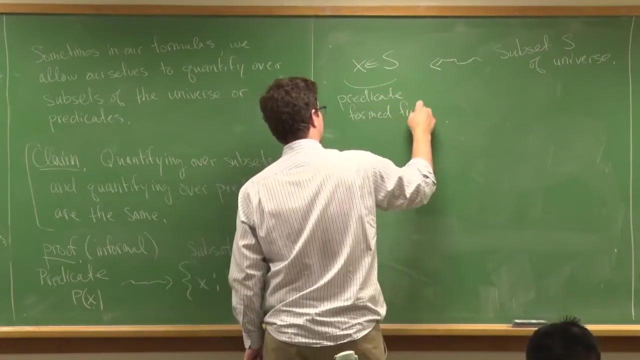 And you take a predicate, X is an element of the universe. So you can go this way. When we take a predicate, X is an element of s, So this is a predicate Formed from the subset OK, So these are really the same thing. 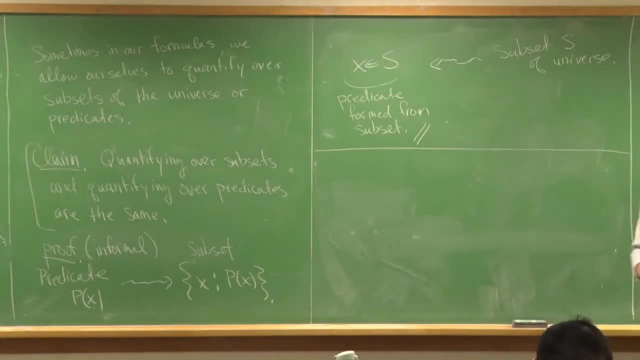 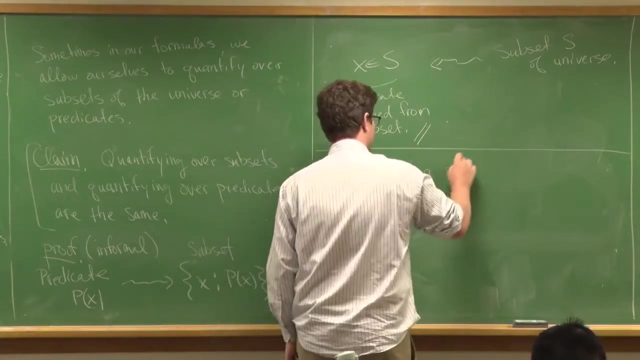 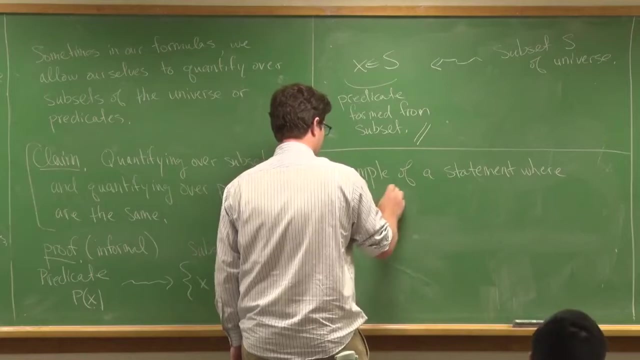 OK, Do you guys see what I mean by this now That quantifying over predicates and quantifying over subsets the same thing. and let me give you an example of where we quantified over predicates or subsets. so an example of a statement where we quantified over: 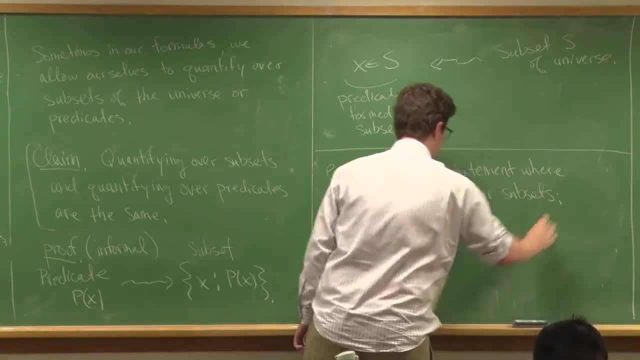 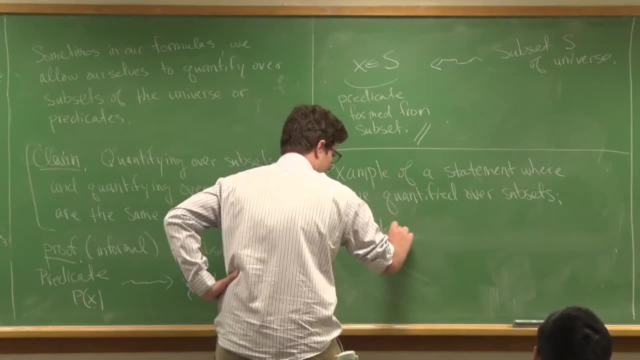 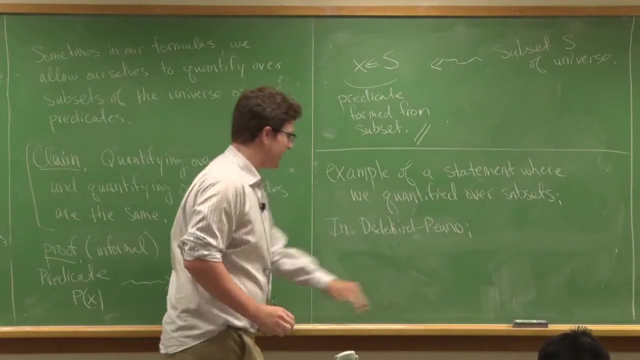 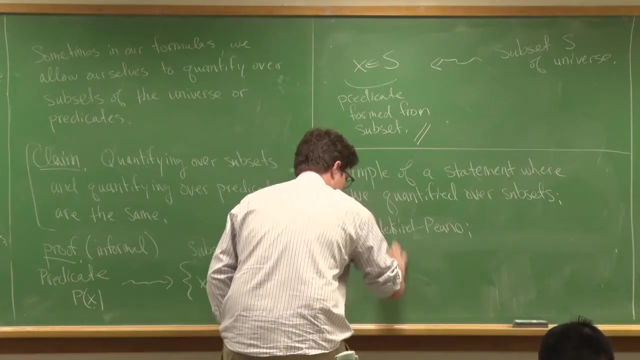 subsets. okay, so in. so. so in the didache and piano axioms did a kind piano right. we had this induction: axiom right said that for all, for all s the subset of the natural numbers. so this is a quantifier over subsets, you see. so this is a 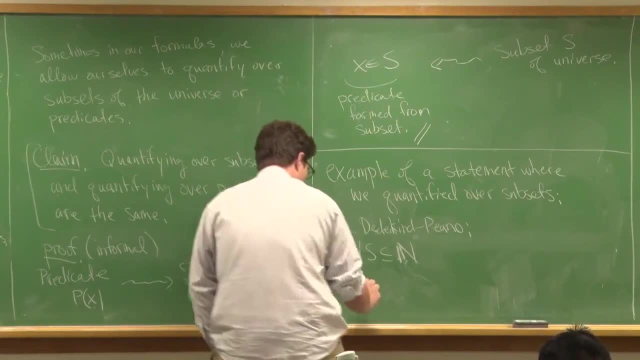 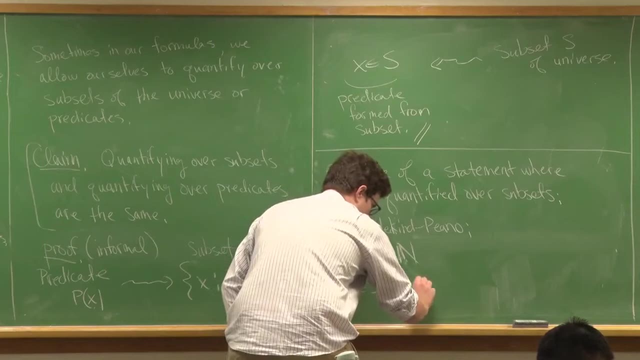 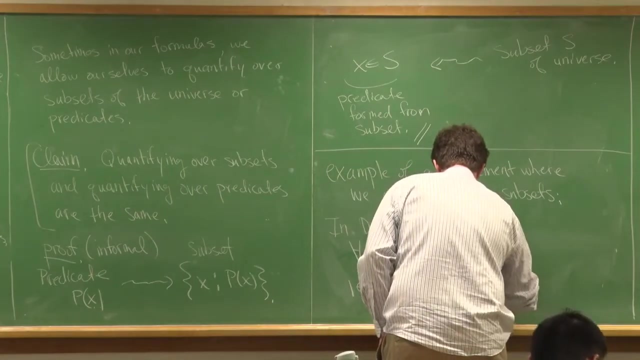 quantifier over subsets. you see so this is a quantifier over subsets. you see, so this is a for all set subsets of the natural numbers, if one was an element of s, and and for all n in the natural numbers if n was an s. this implied, and then we had 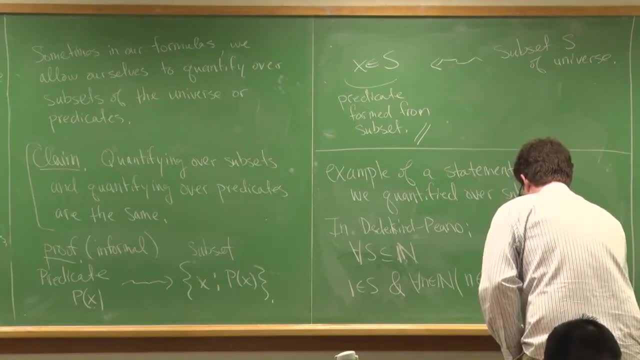 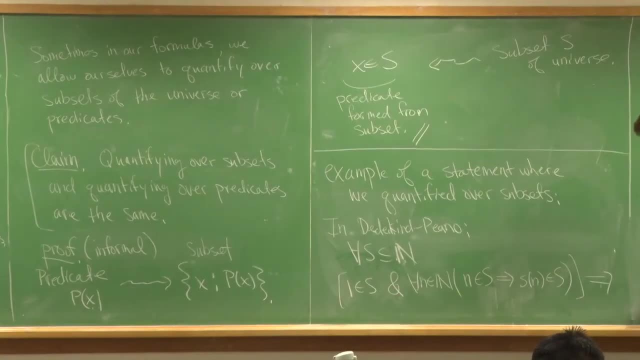 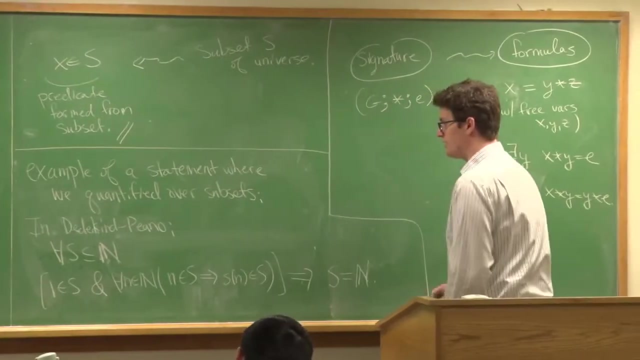 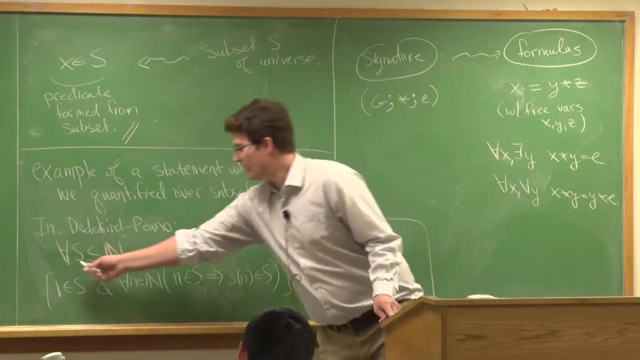 the successor function, so s of n was an NS. then these two things, these these two things implied that the following was true: that s was equal to the natural numbers. okay, so here was this: induction axiom right, and the induction axiom said for all subsets, blah, blah, blah, right. and I mentioned that we could have formulated it as for: 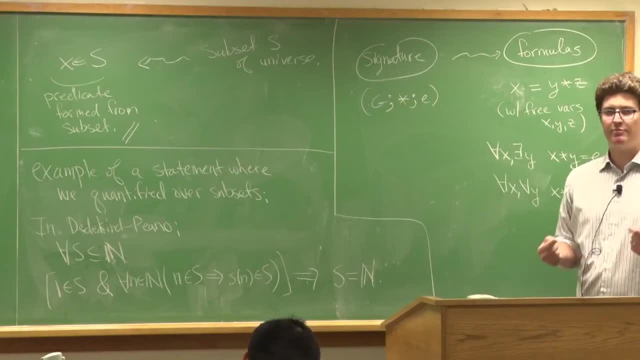 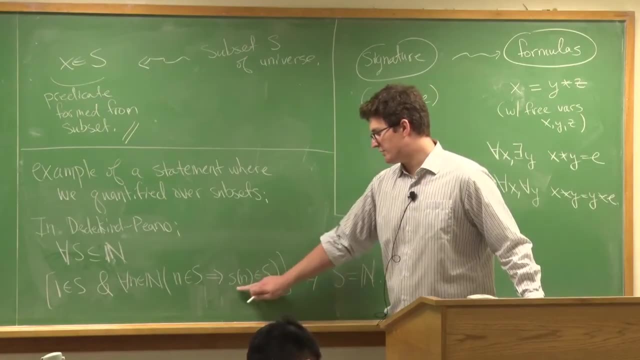 all you know, propositions, if P of 1 is true, and P of what? P of n implies P of n plus 1 and so there, okay, so let me tell you that there's two, there's two. there's these kind of a poor choice of letters here. this is a. 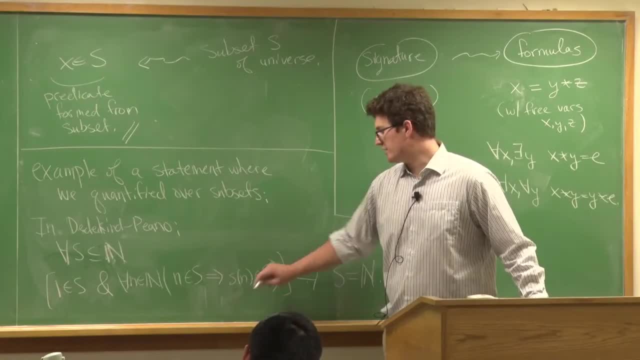 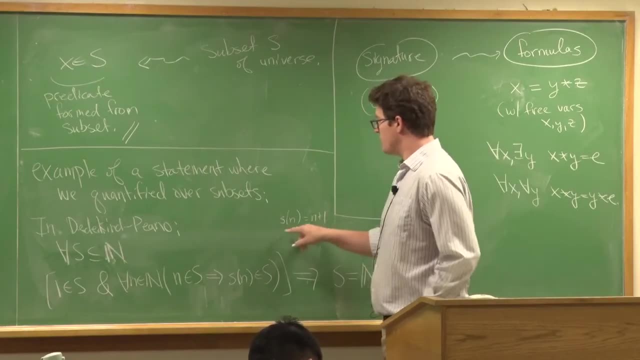 this is kind of a poor choice of letters here. this is a lowercase s. this lowercase s. this lowercase s is really represents lowercase s. S of N is n plus 1 right is n plus 1 right. it's the successor function, but I'm trying to be careful. 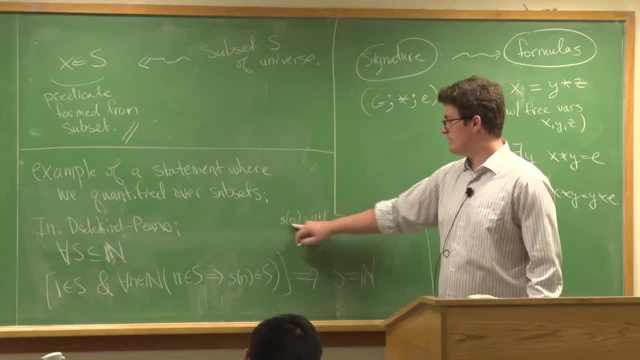 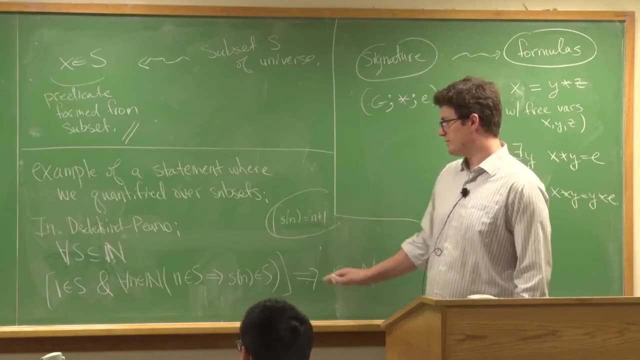 about what symbols I use today. okay, so we use n plus 1 before. okay, this is like. this is how we're supposed to think about it. okay, so this is the axiom of induction. okay, and so formulas say: let's think real hard. this is long and short. 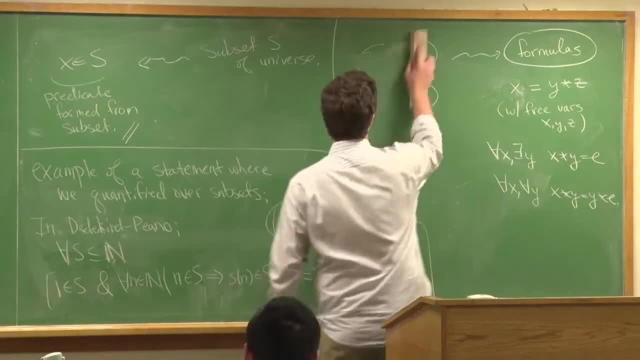 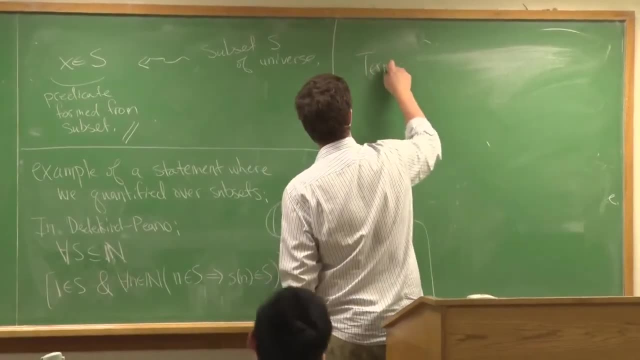 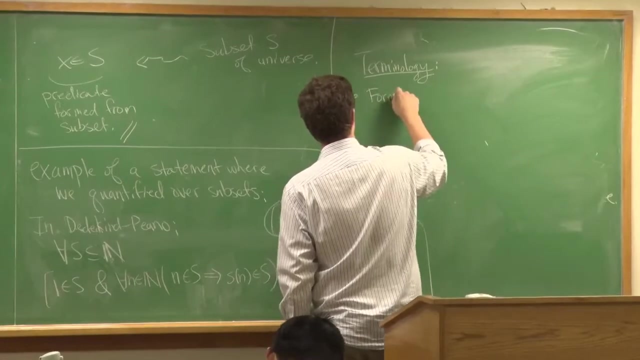 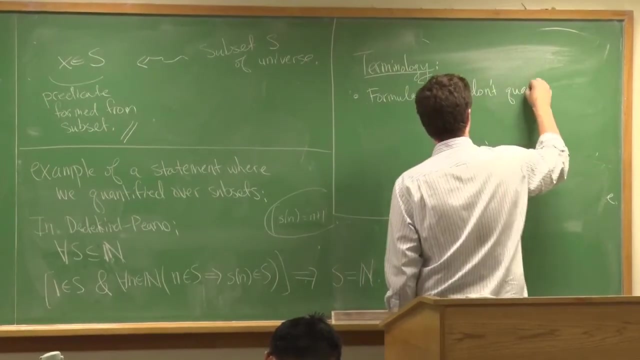 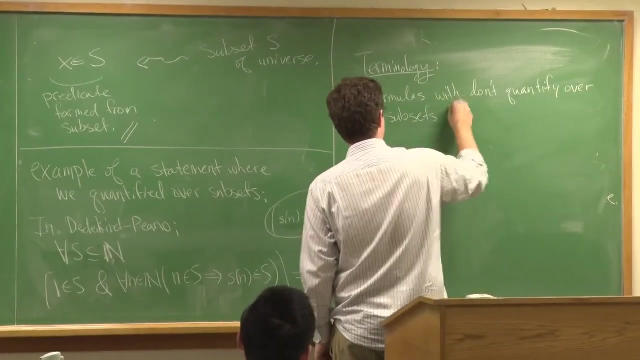 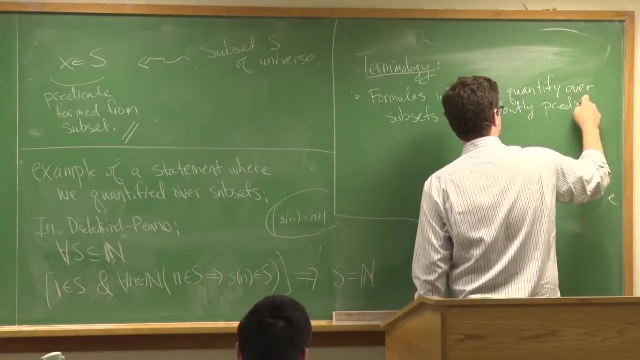 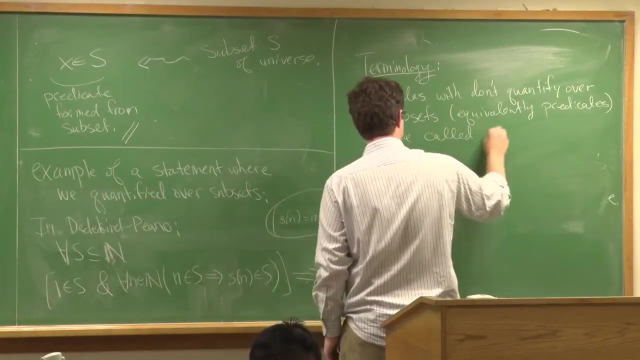 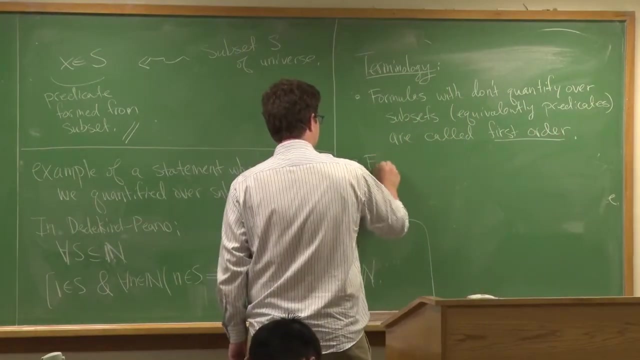 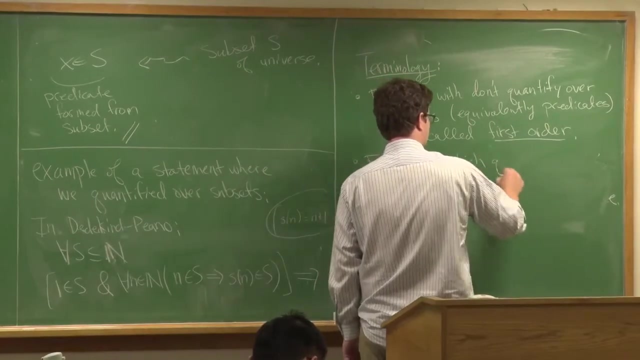 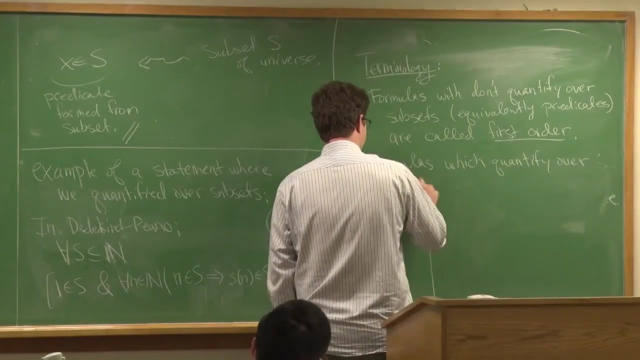 Okay, so now. so let me say, let me give you some terminology, okay. So formulas which don't quantify over subsets, equivalently predicates are called, are called first order Okay, and formulas which quantify over subsets, subsets of the universe- are called 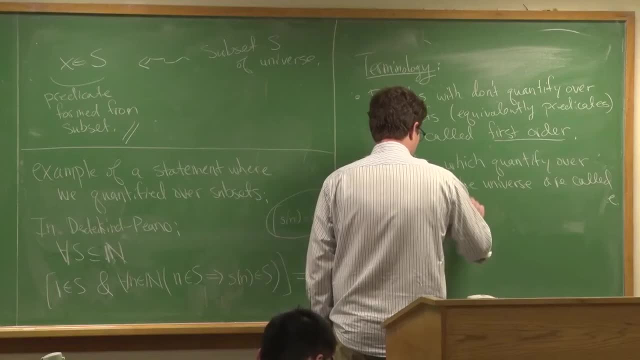 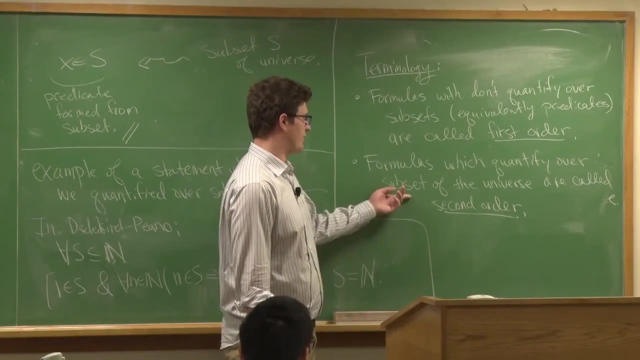 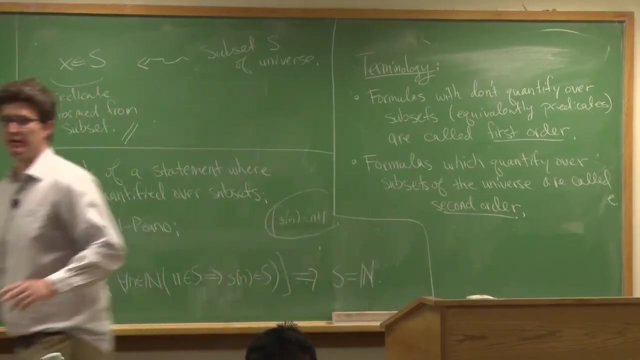 second order. In the second statement I didn't say. I didn't say subsets of the universe. quantify over subsets of the universe, right, And I could have written equivalently: predicates: if you quantify over predicates, it's also second order, okay. 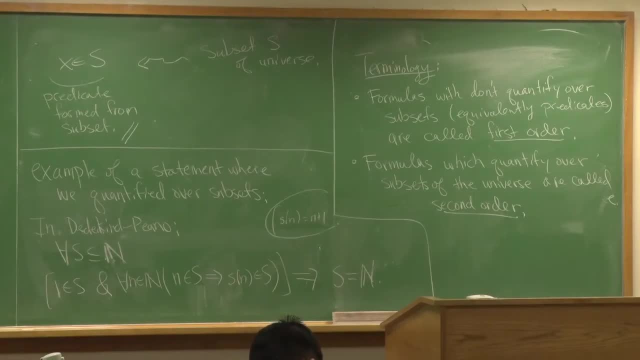 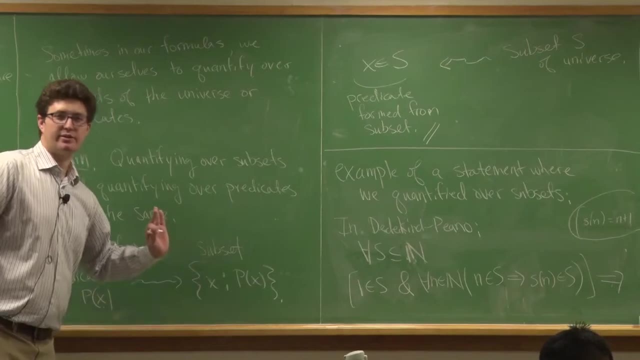 But there, you can always convert between the two very easily, okay, And using this thing. so, if you have a predicate, you form the set of X such that P of X is true. okay, And if you have a subset, you form the predicate that X is an element of S, okay. 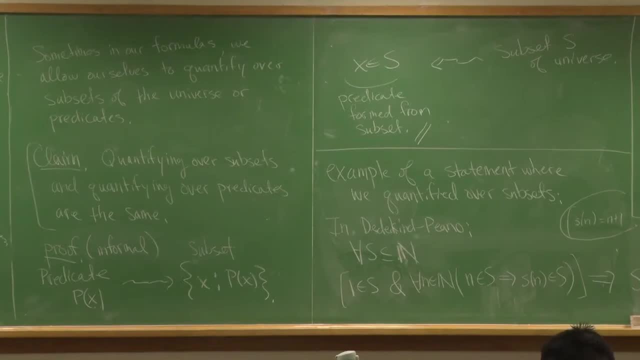 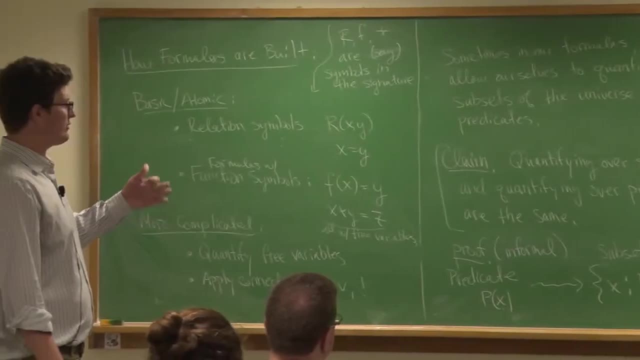 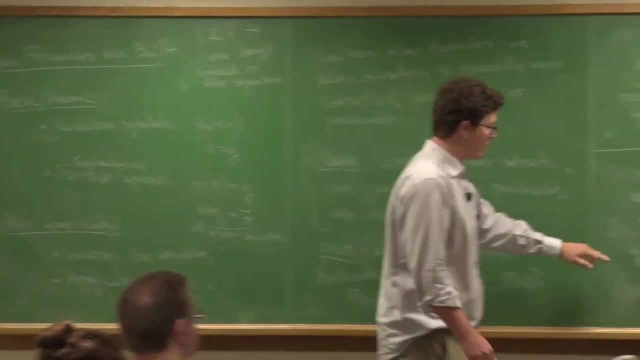 So yeah, so okay. so those are second order things. so we have a notion of first order and second order formulas. Formulas are built from the signatures right, And sometimes we allow for them to quantify over subsets of the universe, okay. 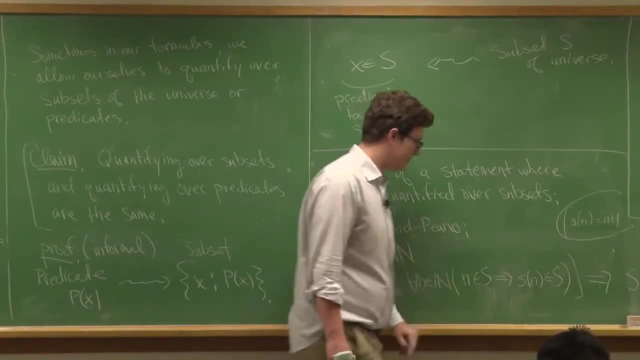 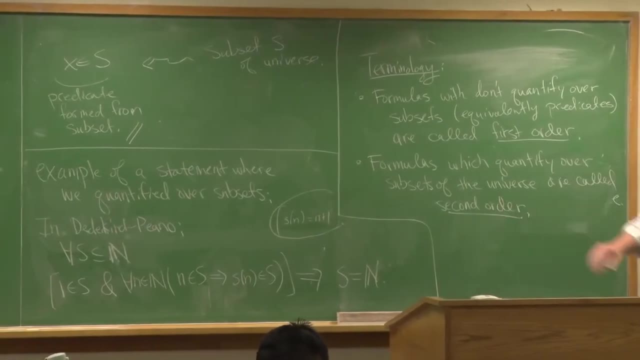 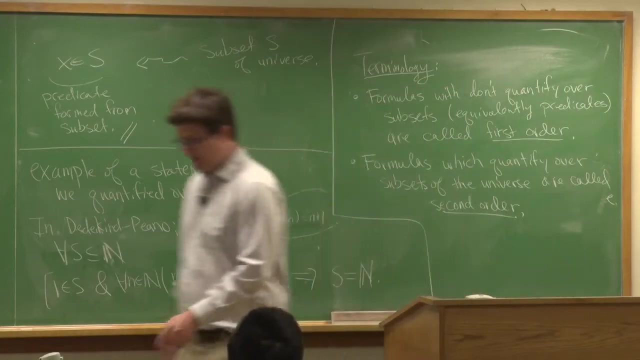 And with this element symbol, okay, And like we did for the div, which was different, right There was, and it was okay, the data can piano axioms. so we call that a second order thing, a second order formula, okay, okay. so there's a list, a lot of words, okay, all right, so we've. 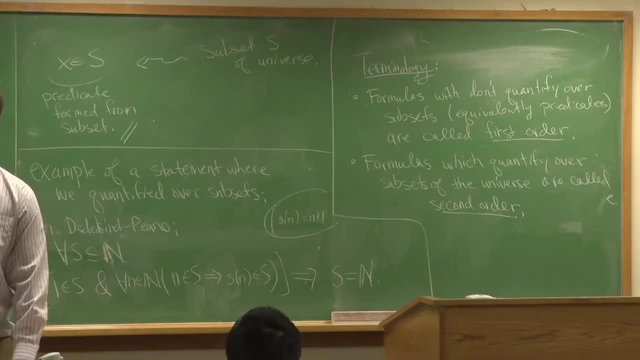 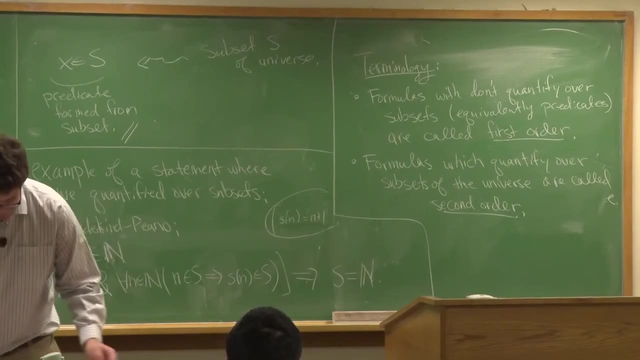 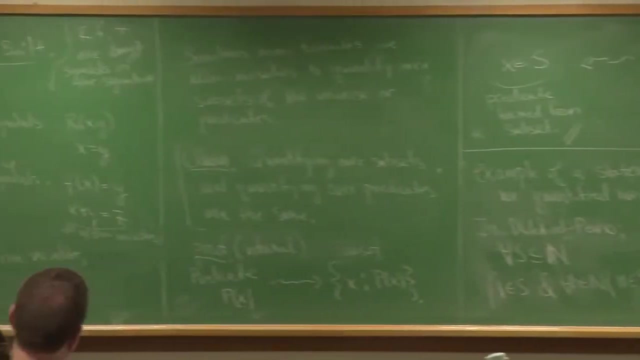 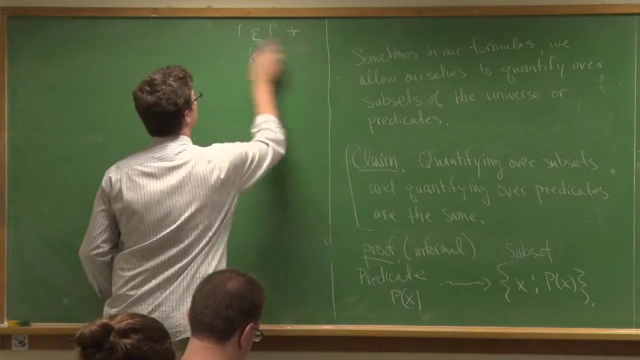 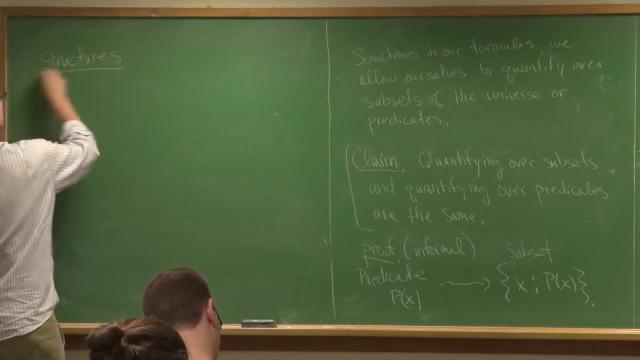 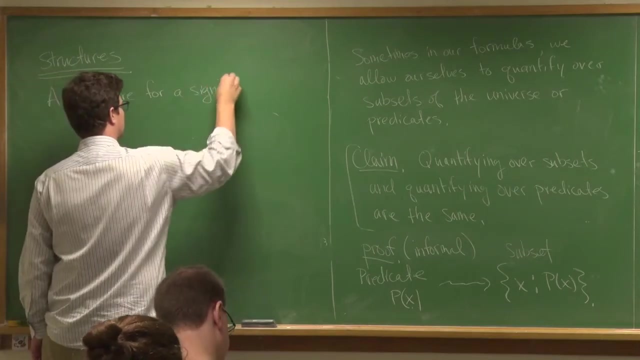 talked about signatures, signatures where the symbols were allowed to use. from the signatures we get the formulas. the formulas, are you the first order or second order? okay, and they're just things that we can say okay. so now let me just say something about structures. okay, structures, okay, so structures, so a structure for a signature, so a 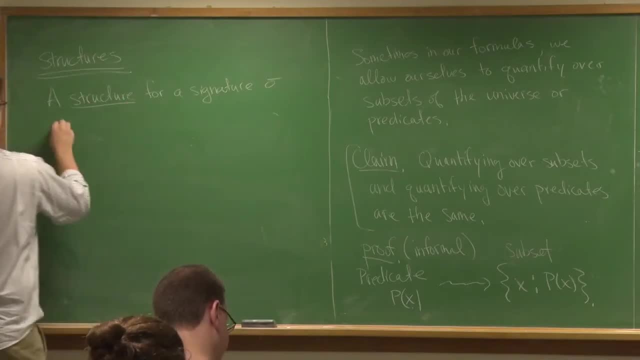 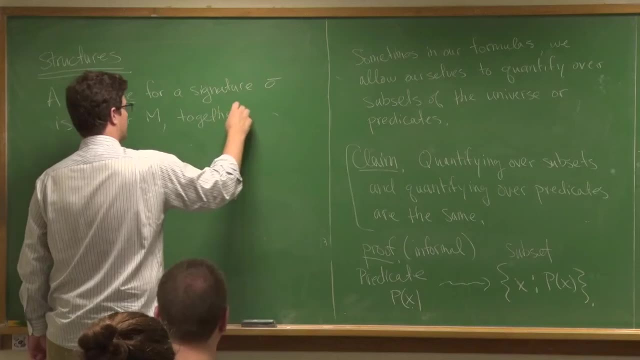 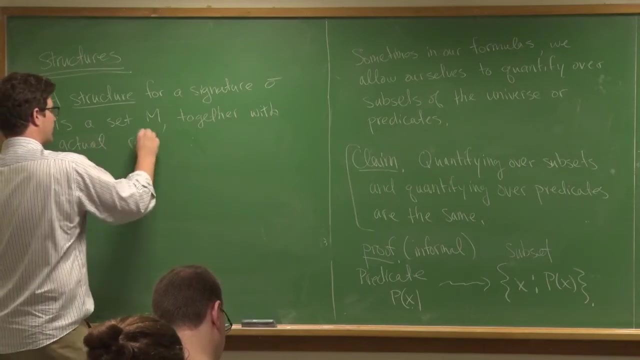 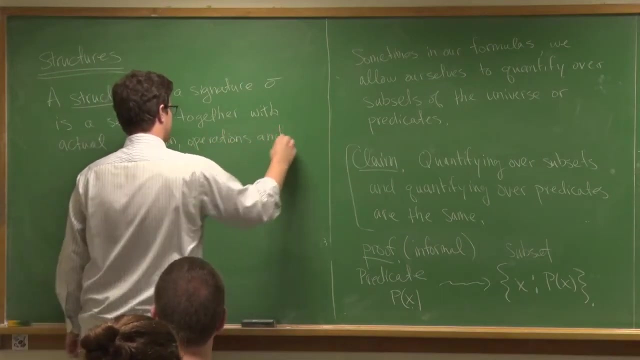 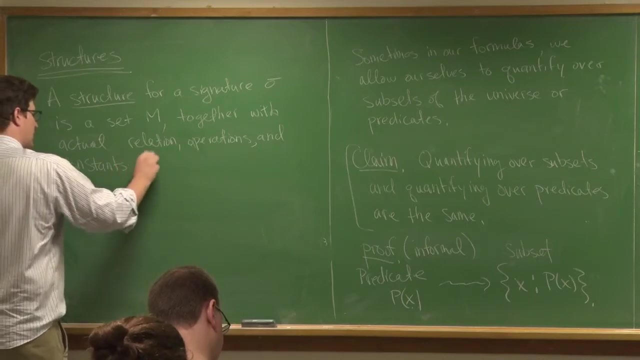 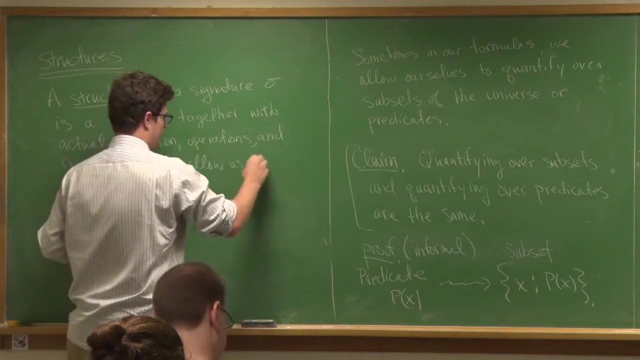 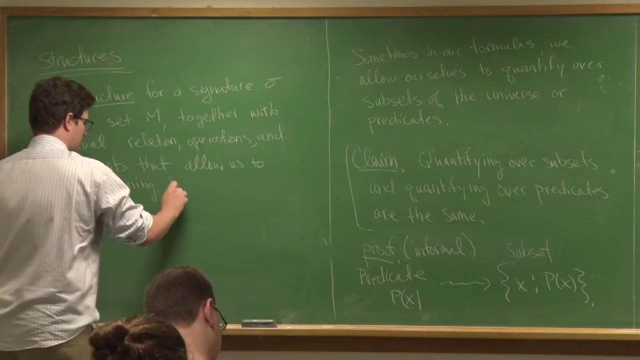 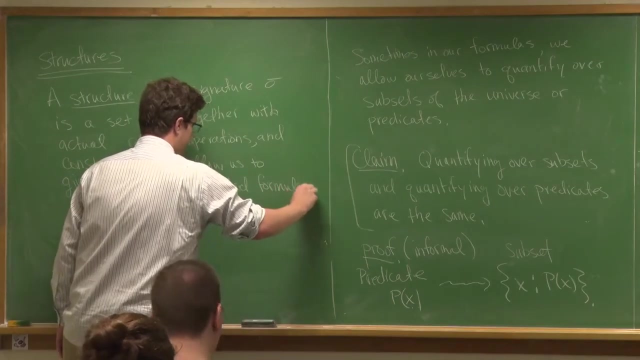 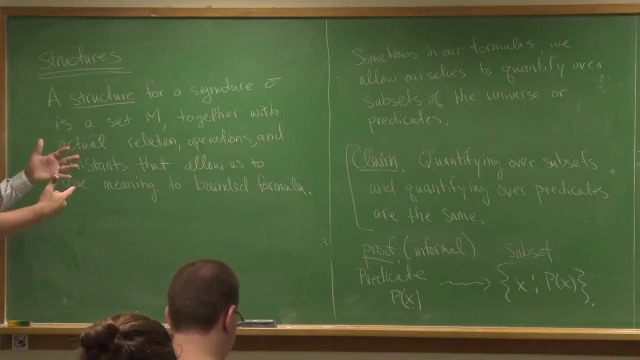 structure for a signature. Sigma is a set M, together with with actual relations, actual relations, operations, and constants, and constants that allow us to give meaning to formulas, to give meaning to bounded formulas. so so this means that when we have a structure right, we we get to interpret the symbols. so this means that when we have a structure right, we we get. 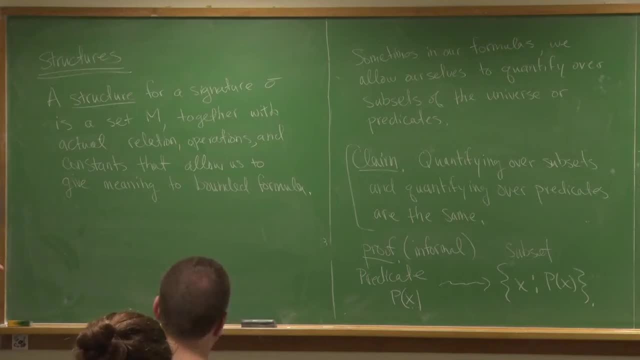 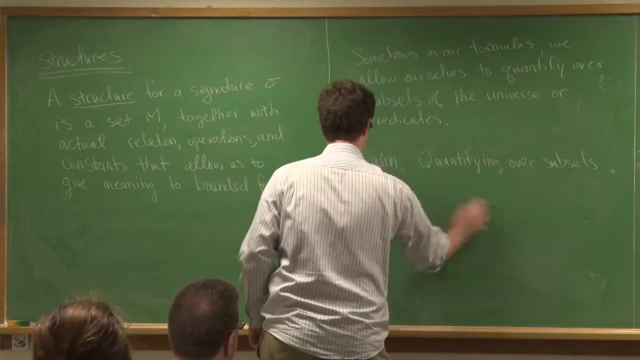 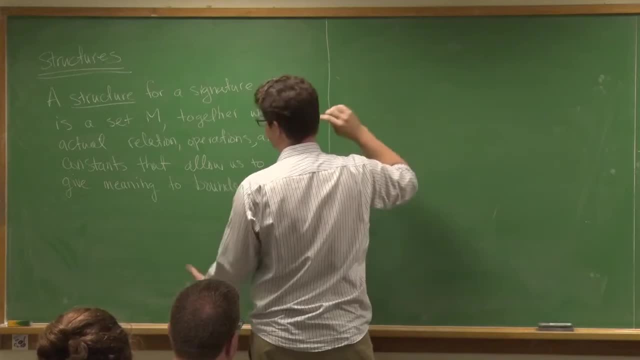 and they don't need necessarily need to be. so let me give you an example: the. and they don't need necessarily need to be. so let me give you an example: the. and they don't need necessarily need to be. so let me give you an example: the formulas don't necessarily need to be. 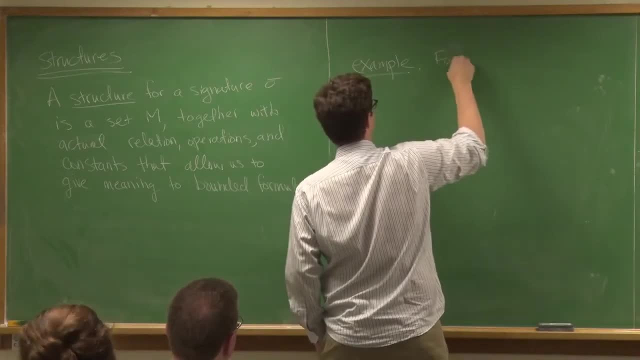 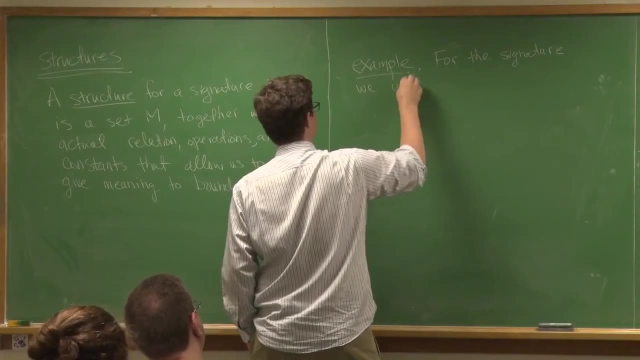 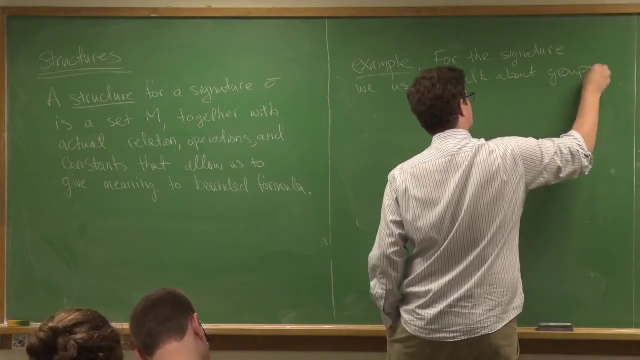 formulas don't necessarily need to be formulas, don't necessarily need to be true. okay. so for the signature we use to true, okay. so for the signature, we use to true, okay. so for the signature we use to talk about groups. so this is the talk about groups. so this is the. 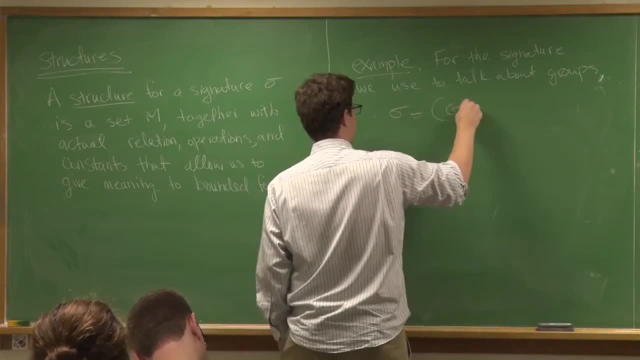 talk about groups. so this is the signature, signature, signature, Sigma, Sigma, Sigma. we'll call it G. we have our multiplication, we'll call it G. we have our multiplication, we'll call it G. we have our multiplication. symbol, then we have our identity here. symbol, then we have our identity here. 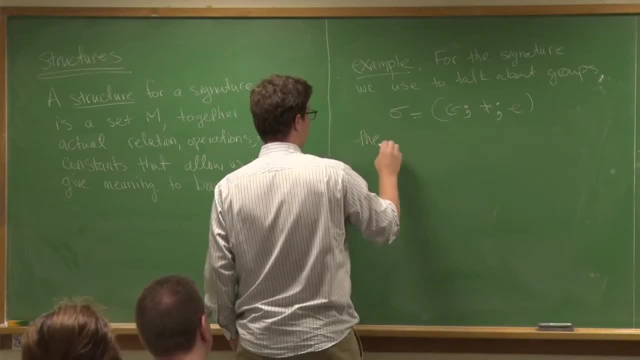 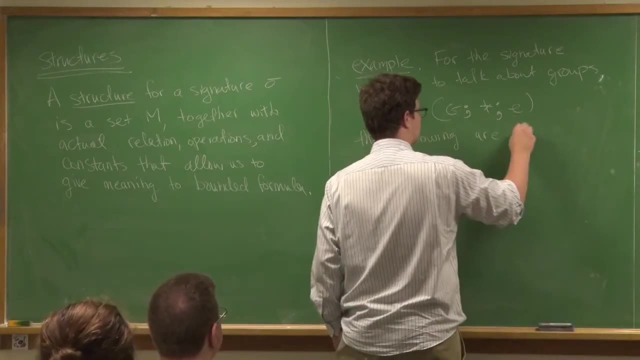 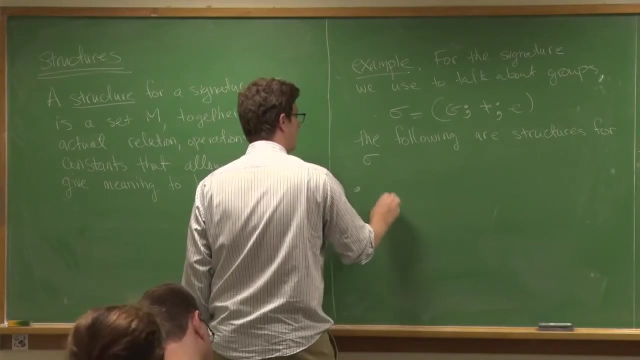 symbol, then we have our identity here: the. the. the following are following our the. the. the following are following our the. the. the following are following our structures for Sigma: okay, so we'll do structures for Sigma. okay, so we'll do structures for Sigma. okay, so we'll do the natural numbers and then we'll. 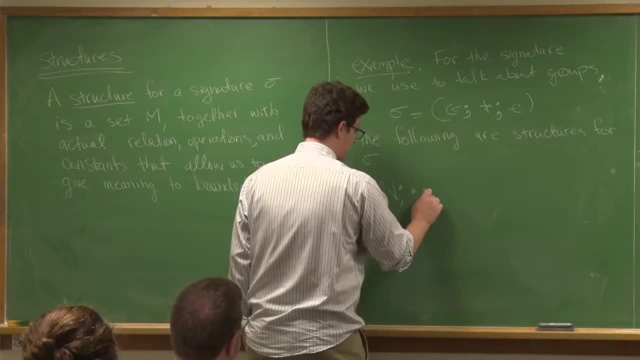 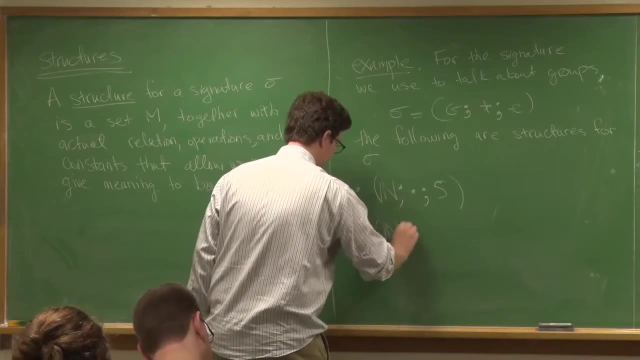 do the natural numbers, and then we'll do the natural numbers, and then we'll do it with multiplication, and we'll do five. do it with multiplication and we'll do five, do it with multiplication and we'll do five. okay, we could do the natural numbers. okay, we could do the natural numbers. 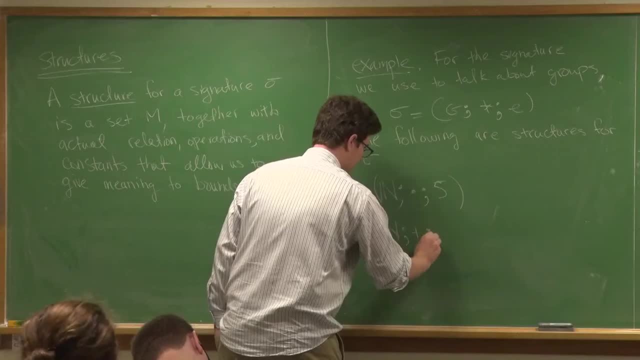 okay, we could do the natural numbers with addition, and we could do say five as with addition, and we could do say five as with addition, and we could do say five as well. or we could do I don't pick well, or we could do I don't pick. 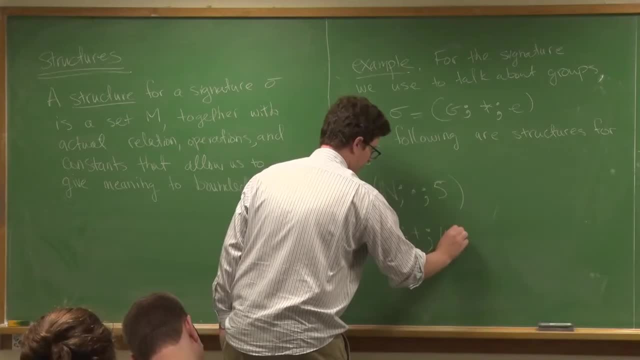 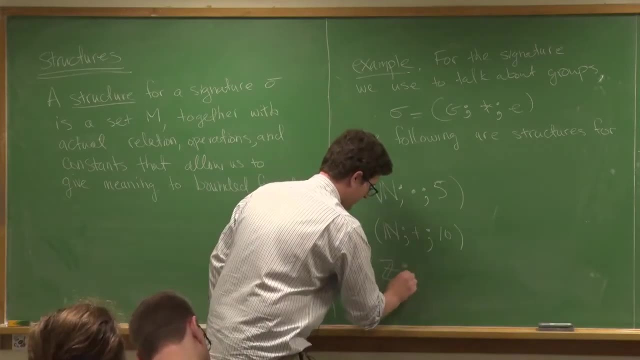 well, or we could do. I don't pick another 100 10, that's that's fine, right. another 100 10, that's that's fine, right. another 100 10, that's that's fine, right. or we could do Z here we could do. 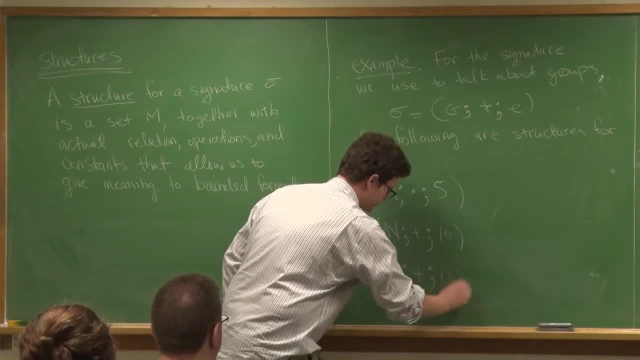 or we could do Z here, we could do Z here, we could do. or we could do Z here, we could do Z plus and zero. okay, so these are all plus and zero. okay, so these are all plus and zero. okay, so these are all structures here. okay, these ones are this. 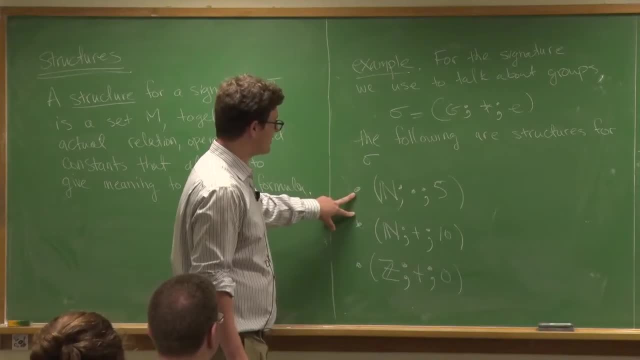 structures here: okay, these ones are this. structures here: okay, these ones are: this is not actually a group right. it just is not actually a group right. it just is not actually a group right. it just means that I can take a formula so for means that I can take a formula so for. 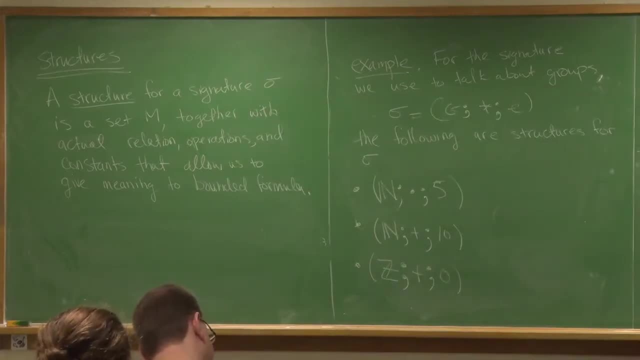 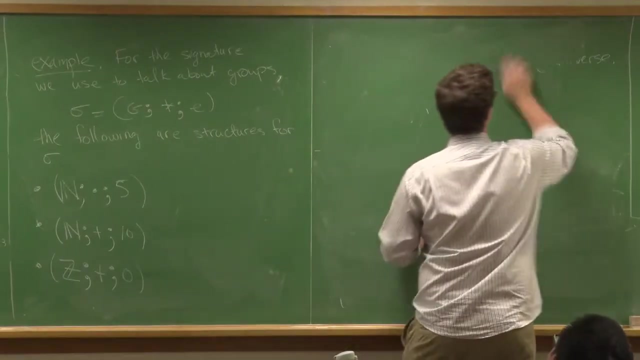 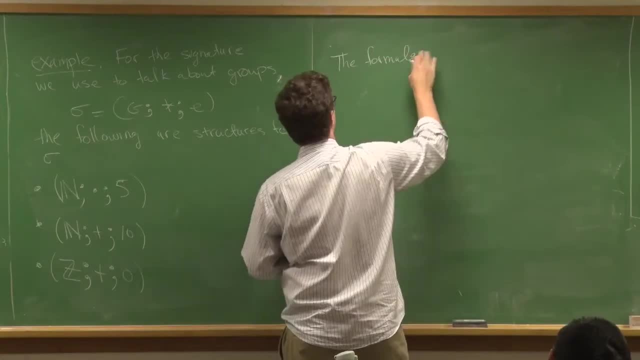 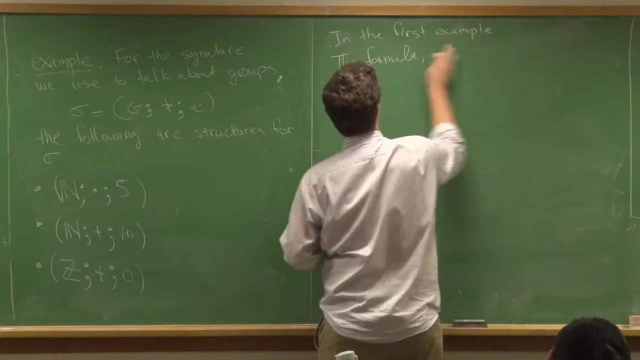 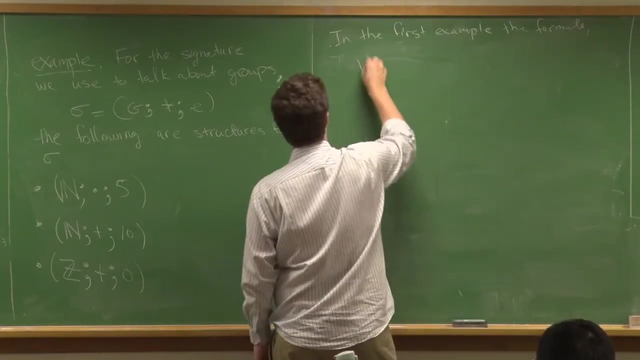 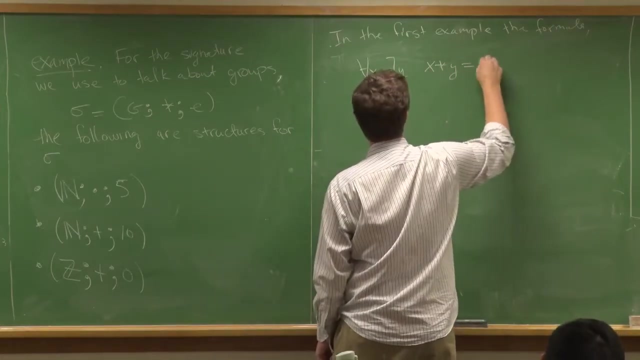 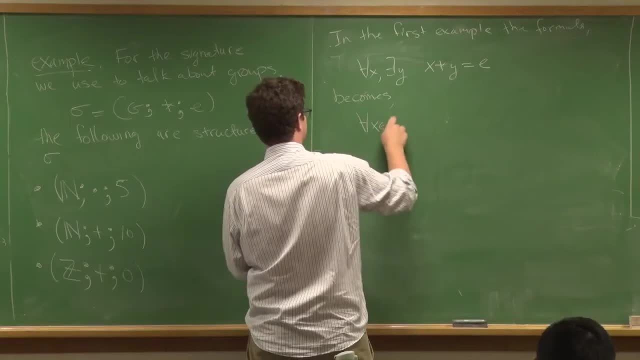 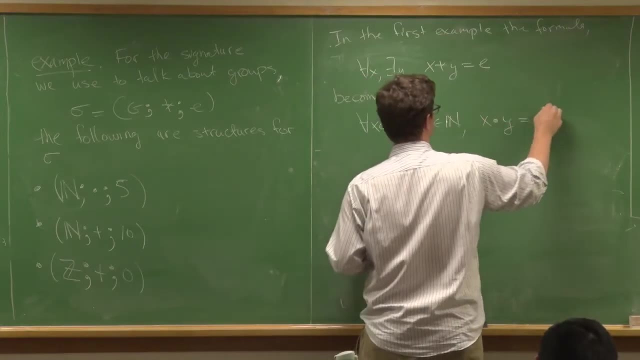 times Y is equal to 2e, right becomes times Y is equal to 2e, right becomes okay. so an actual okay, so an actual okay, so an actual thing. X dotted with Y is equal to 5, right? so thing X dotted with Y is equal to 5, right? so? 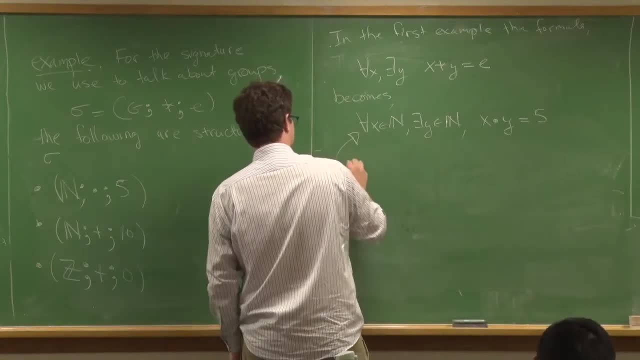 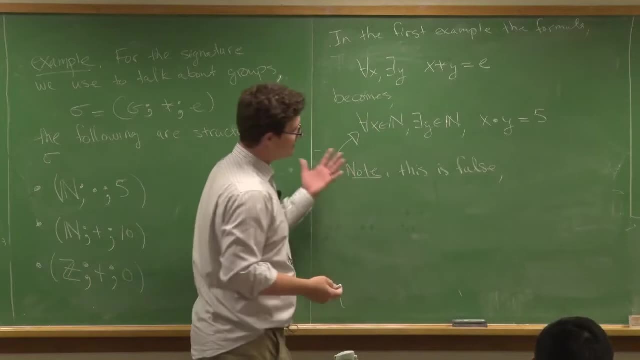 thing: X dotted with Y is equal to 5, right? so this thing is false, right? no, this thing is false right. no, this thing is false right. no, this is false right. we just care that it. this is false right. we just care that it. this is false right. we just care that it returns, that we have something that 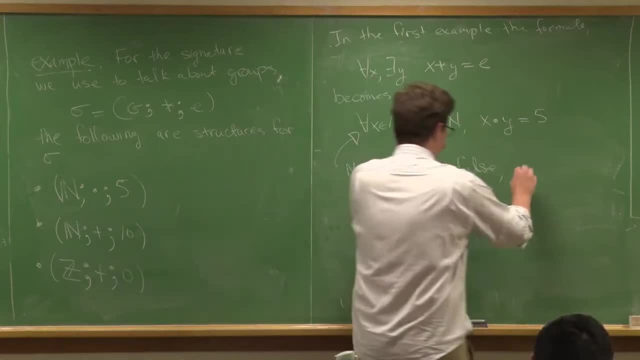 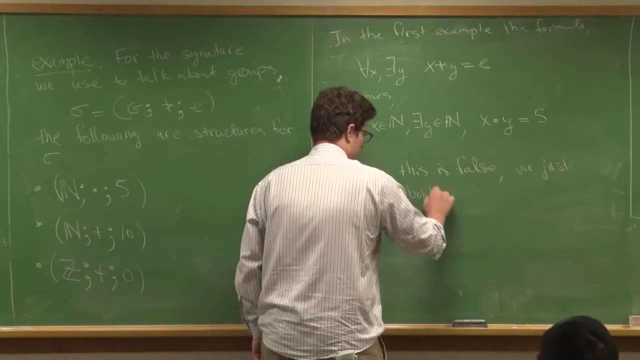 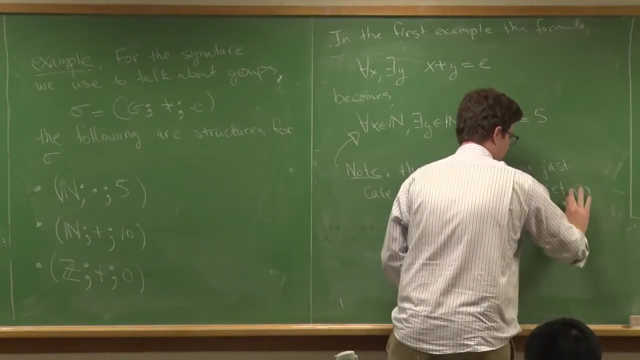 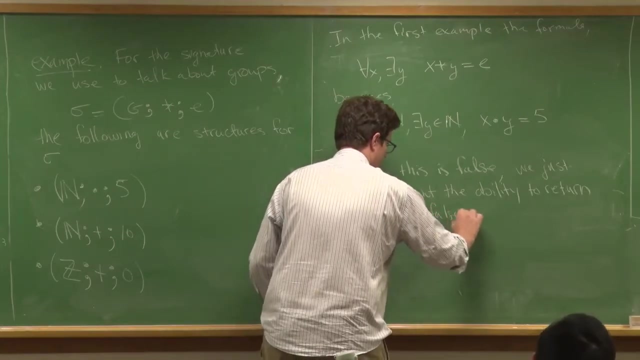 returns, that we have something that returns. that we have something that allows us to return a true or false, allows us to return a true or false. allows us to return a true or false value, right value, right value, right, the ability to return, you know- or false. and so this is a. 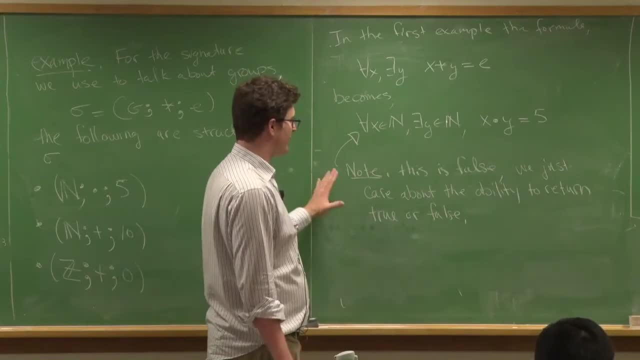 notice that there's no free variables. X is quantified and Y is quantified, and so quantified, and Y is quantified and so quantified and Y is quantified, and so we only care about like whether or not. we only care about like whether or not. 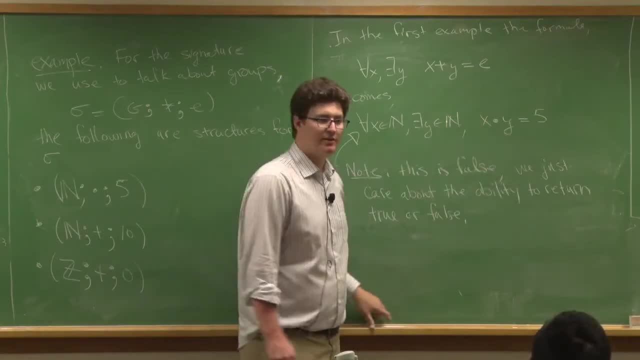 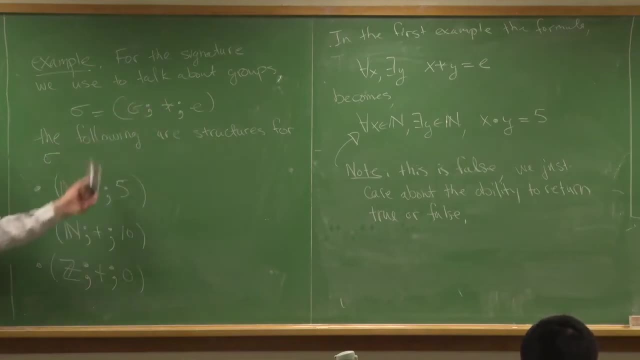 we only care about, like, whether or not this formula makes sense, right, okay, so this formula makes sense, right, okay so, and this is a structure for this, for the signature, do you guys make sense? so it doesn't matter. if we do multiplication, we can interpret this operation as: 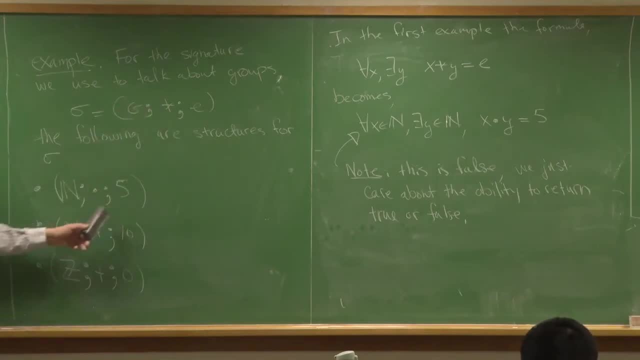 multiple, or addition as well or multiplication. this doesn't need to be one. the identity doesn't need to be the identity, it's just something. this is an example here where it actually happens to be a group, right, but we don't really care. we're not really care concerned about groups right now. we're just 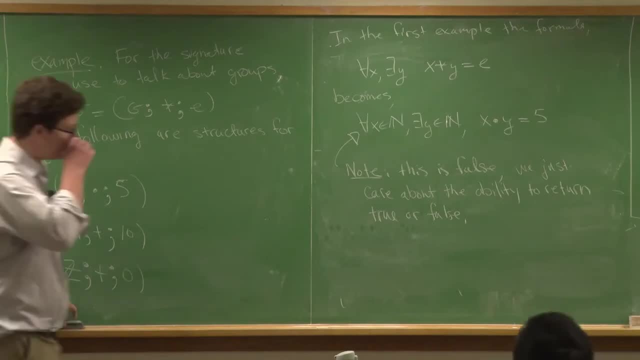 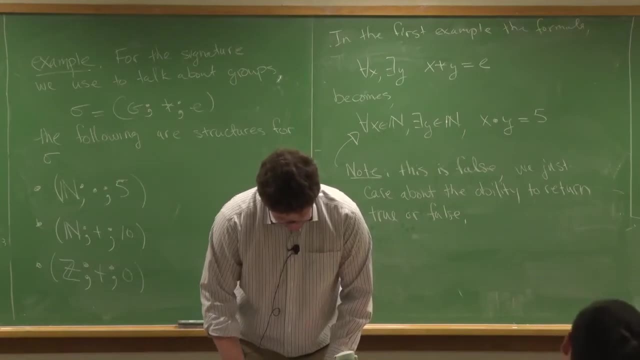 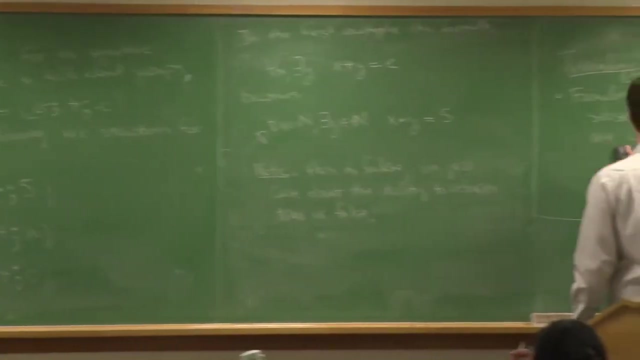 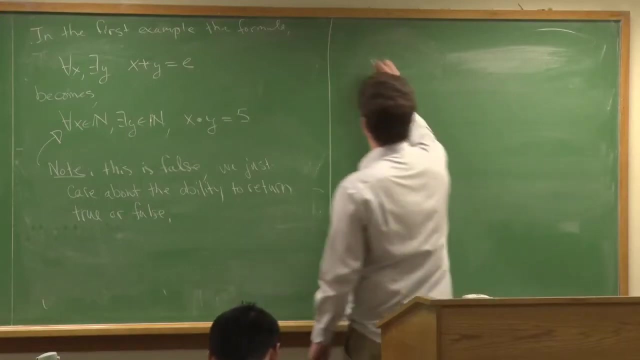 concerned about structures. okay, so that's what a structure is. yeah, oh, okay, okay. so now let me talk about theories. okay, so we've talked about signatures. from signatures come formulas, okay, and structures are things where we can interpret the formulas given the signature. okay, so theories. what's a? 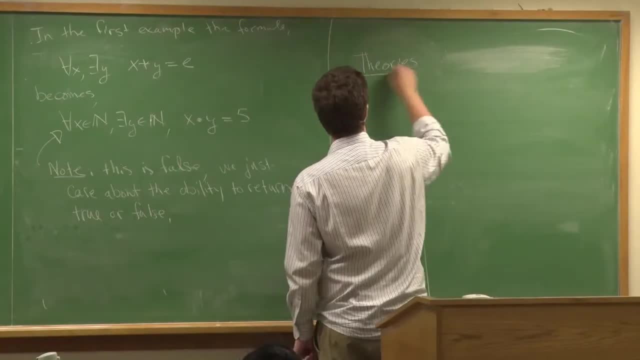 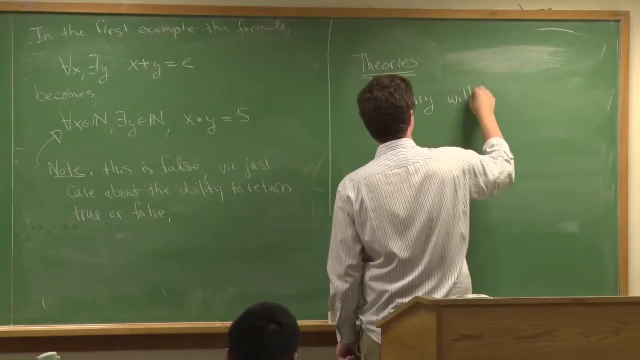 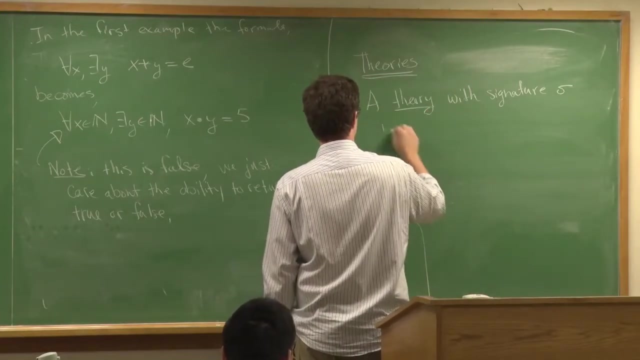 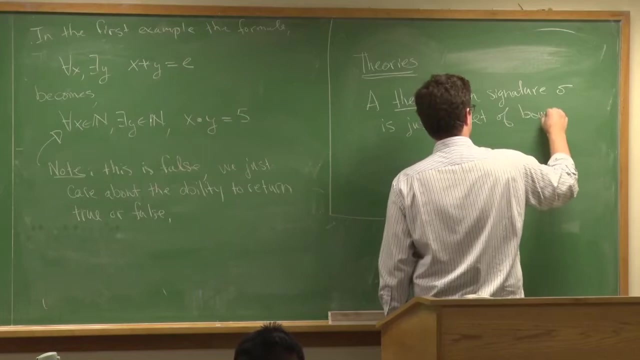 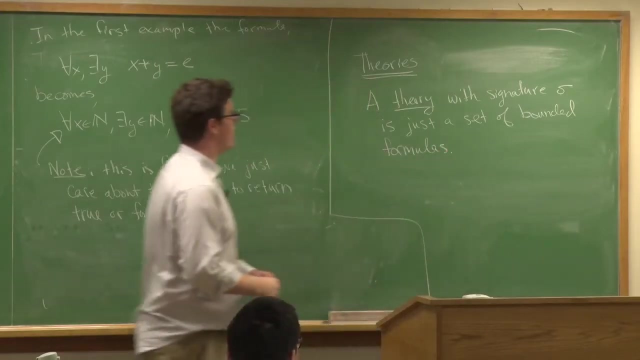 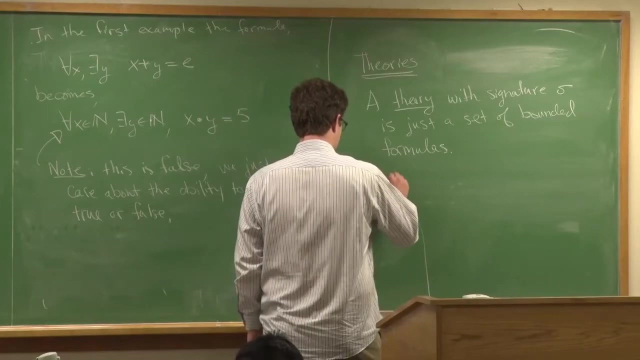 theory. so a theory is a with signature. Sigma is a collection, is just a set, a set of bounded formulas. it doesn't matter what the formulas are. I just take any collection of formulas and that makes a theory. it can be the stupidest theory in the world, right, but it's a theory. that's what we call it, okay. so for example, for: 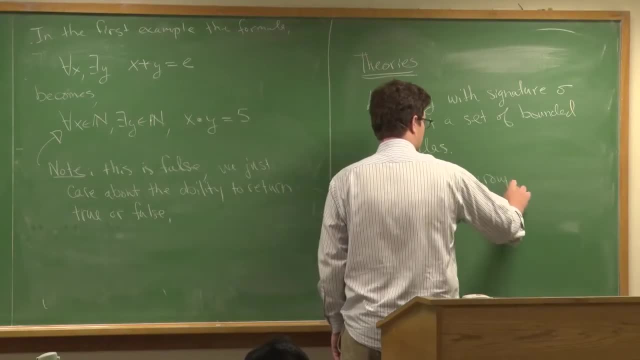 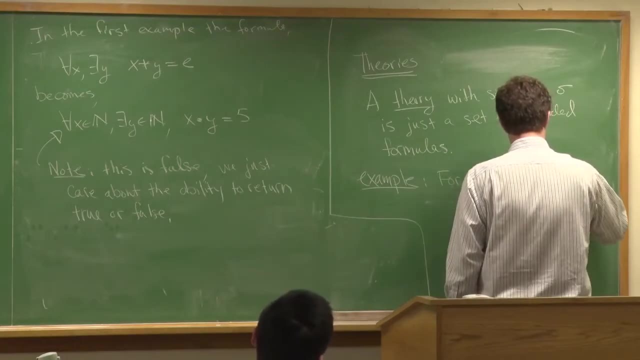 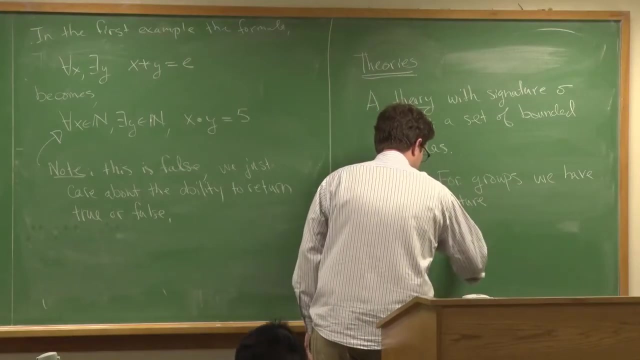 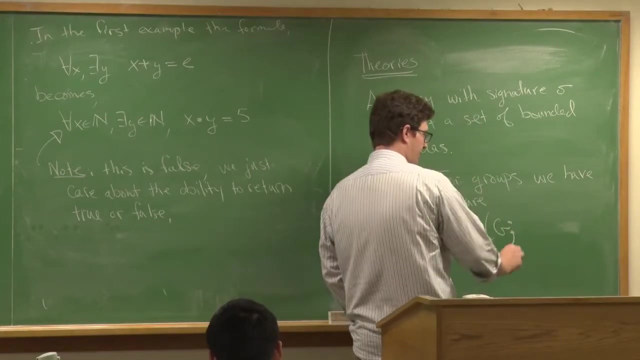 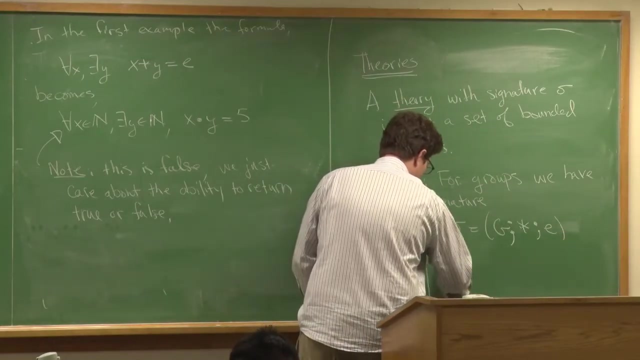 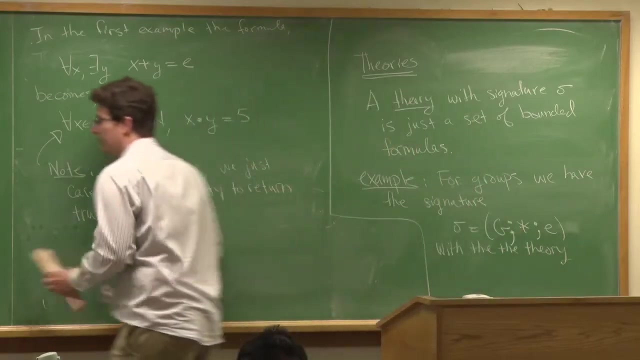 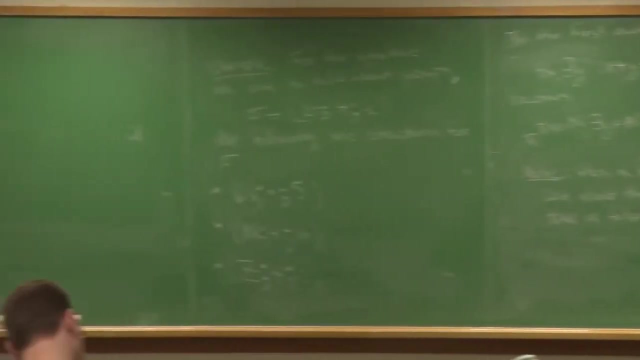 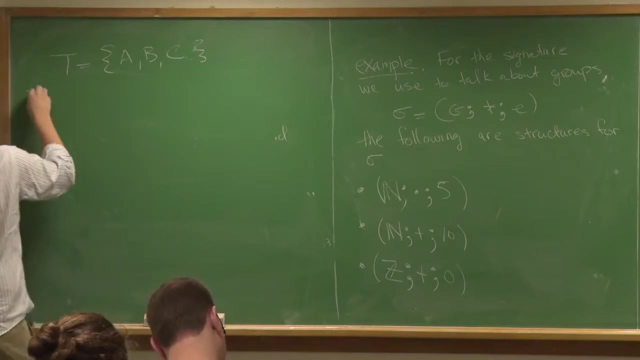 groups our theory, we have our signature. the signature here's Sigma and this is going to be so, this was so. we have this sort here, then we have the multiplication, and then we have the identity, we have the signature, this with the theory being so, T is the set of a, B, C, where a is equal to, here, a. 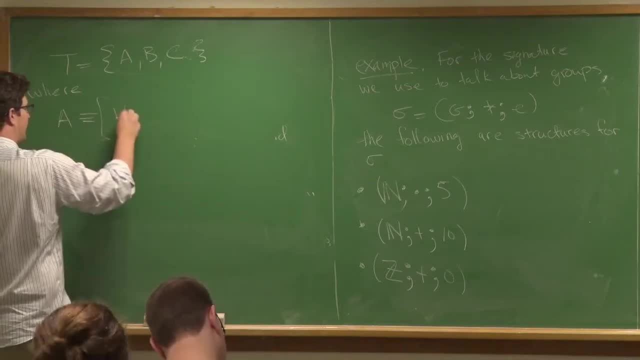 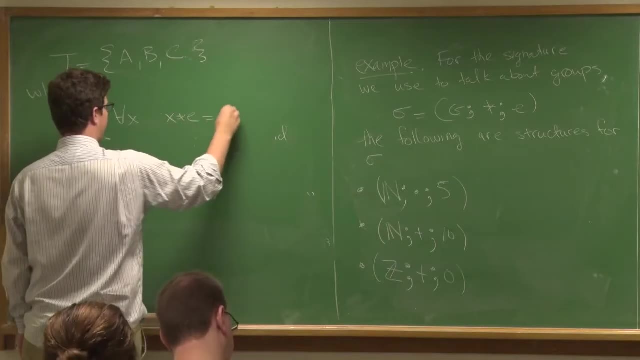 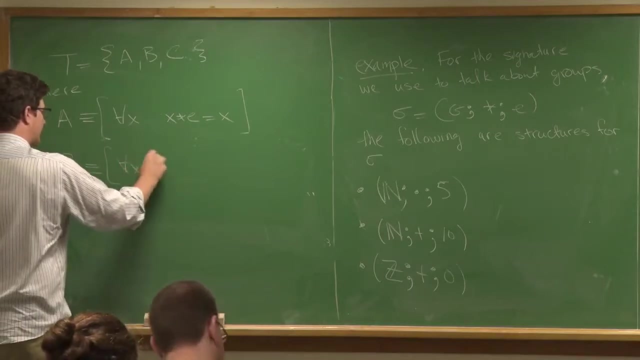 is equal to the following thing is that, for all x, x times e is equal to x. ok, B is the formula. for all x, there exists a y, such that x times y is equal to e, that there's a right inverse. and see, you know, and I could strengthen this, 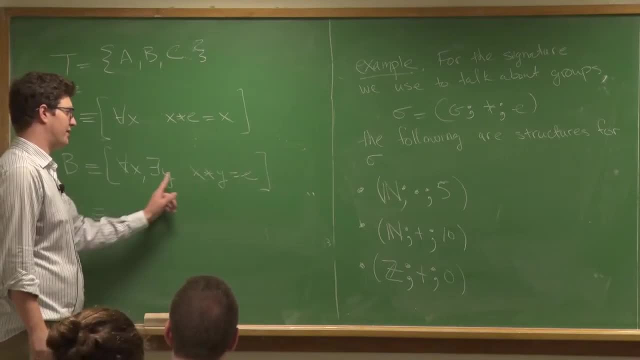 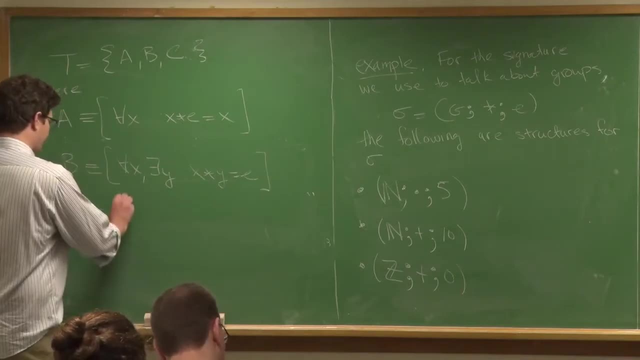 if I wanted to, I could add the that not only there's a left x, that this inverse is the, the right inverse, but it's also the left inverse as well. so I could add that as well, if I wanted to. right C could be for all x, all y and all. 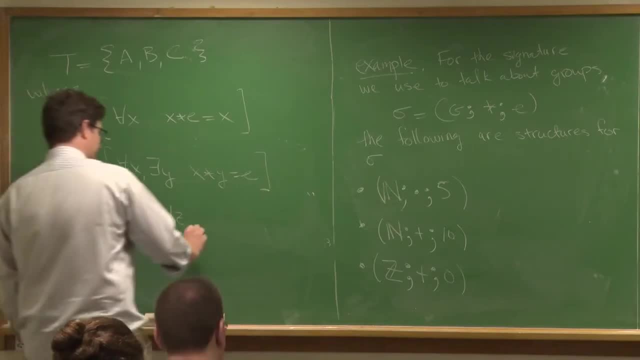 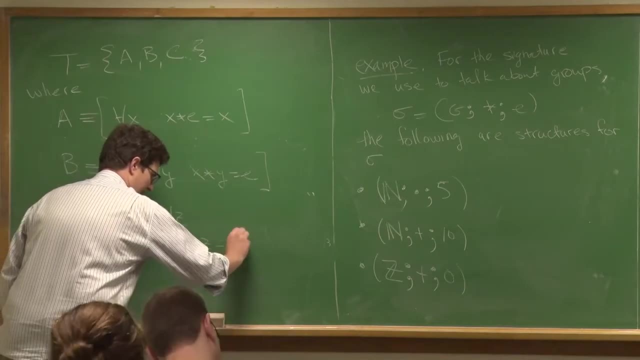 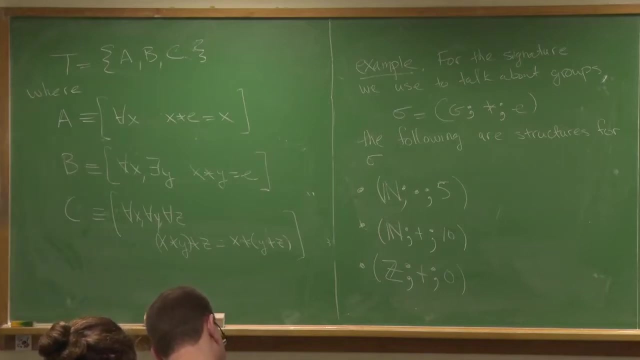 Z, that x times y times z is equal to x times y times z. ok, so this was, this was the formula for this is the. this is a theory of groups. it's this collection of, we could just say a subset of these things. ok, and so subset of formula. 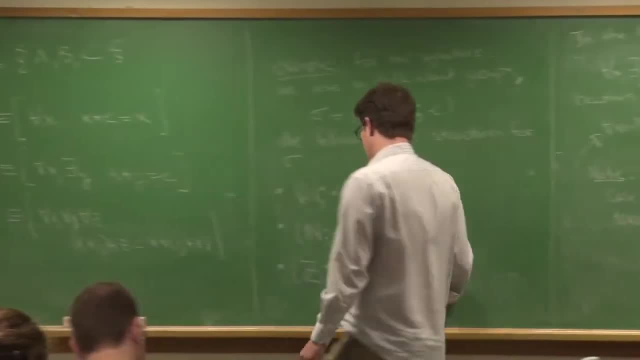 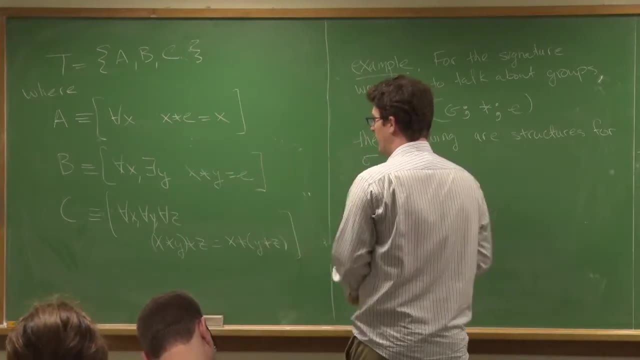 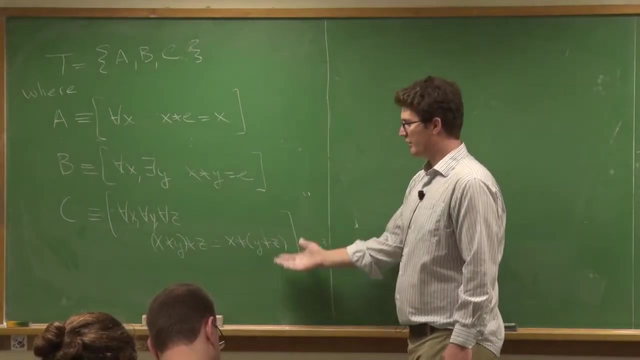 ok, so that's what it is, that make sense. so note that all these things are bounded and all these these formulas here their first order. so this is a first-order theory of groups. ok, there's no statement here about that. quantifies over sets. the data can piano axioms. on the other hand, they did quantify over subsets, so it 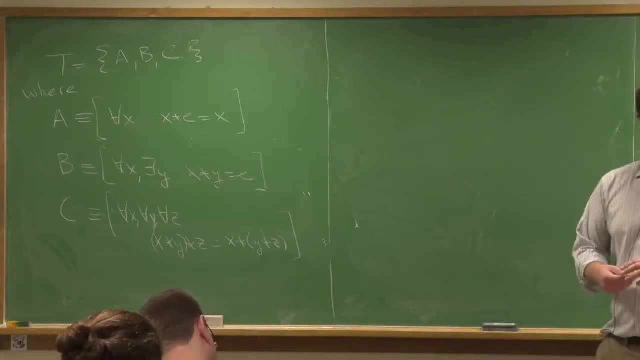 had that induction axiom. that said, you know well, for every proposition, if you have the first thing and then this idea where you can go P of n to P of n plus 1, then that implies for all n P of n. that's a second-order theory. ok, because 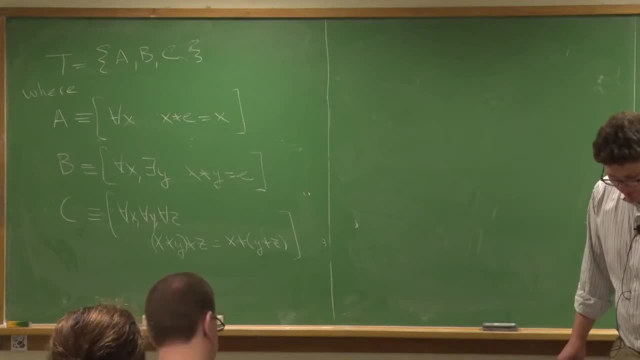 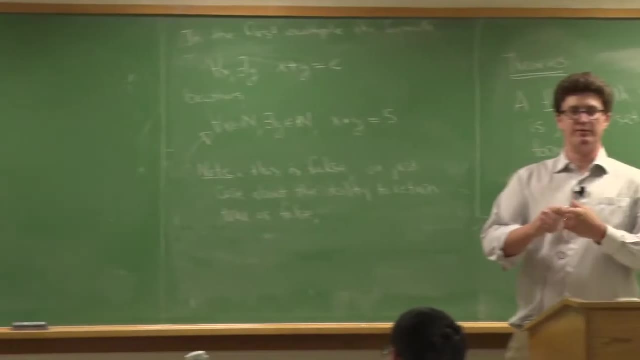 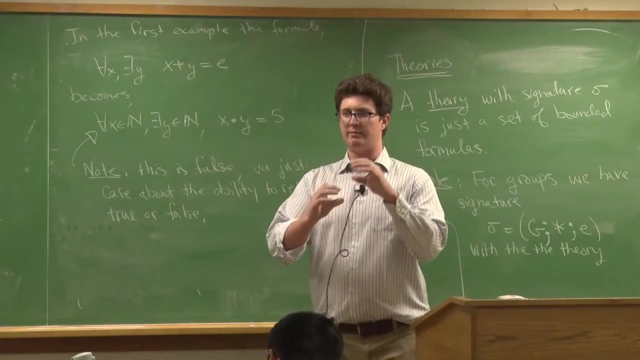 one of the formulas in there is a second-order thing, ok, ok. so let me recap again: ok, signatures, those are the symbols that you, you, you, use right to make up your, your, your formulas. ok, your formulas are built from the atomic things and we use connectives and 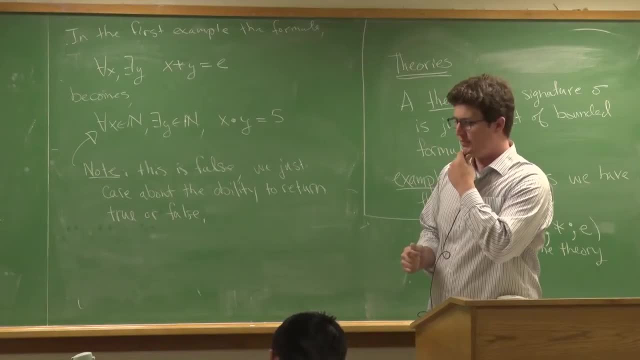 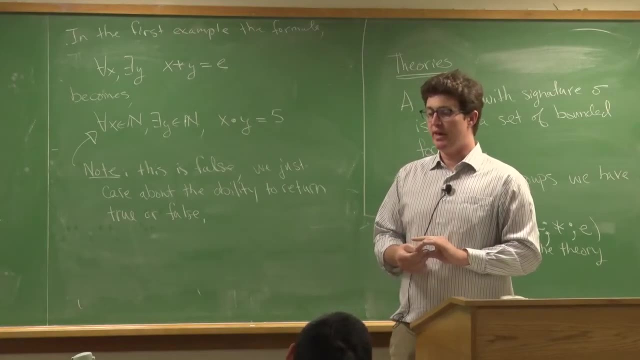 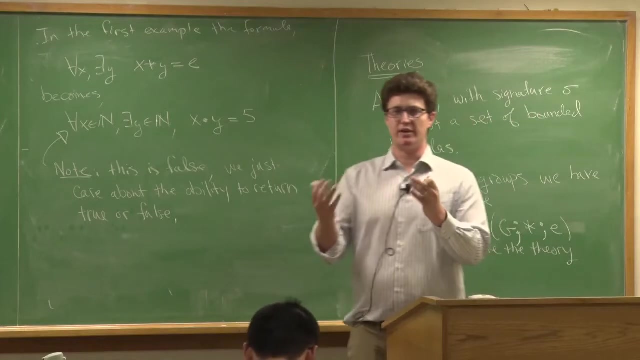 quantifiers to build up from there. ok, then after that they could be first order, second order, second order ones are where you quantify over sets. ok, then we had structures, structures or sets with relations and operations and constants that allow us to interpret the formulas. so, for example, 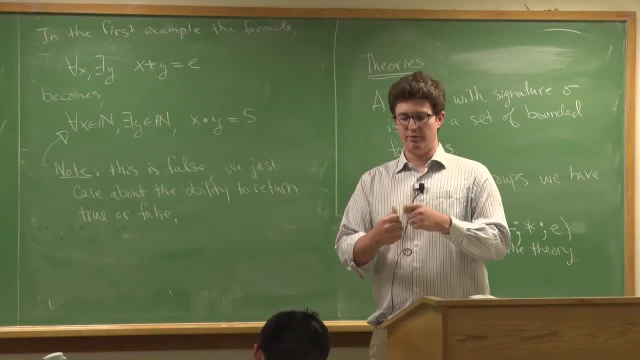 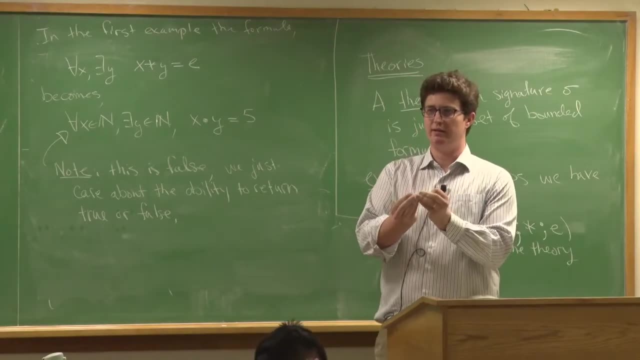 if we had the theory of groups, we and we, you know we are- we had the signature for groups. we need to and we had a set we needed. we could assign the multiplication meaning and for that particular set, now it would be a structure for the theory of groups or for the signature of groups. all right, 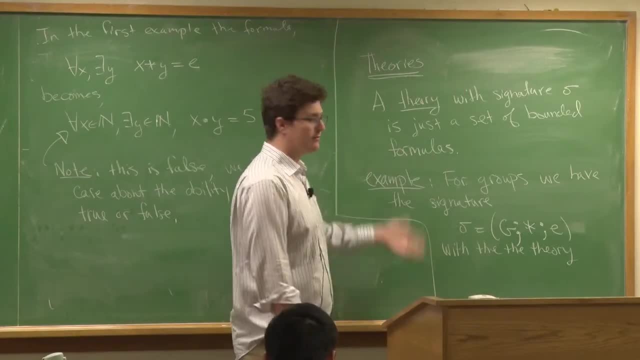 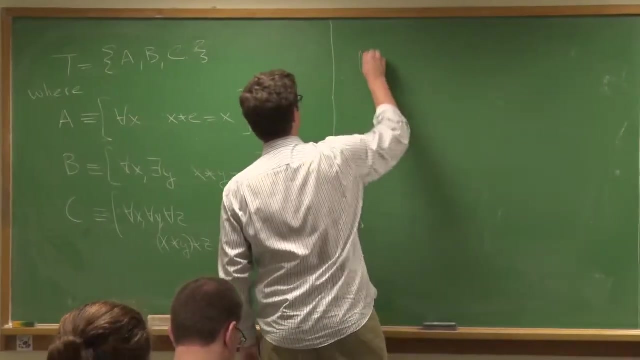 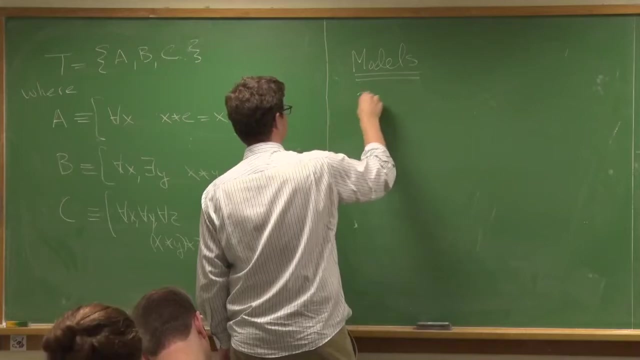 then we had theories. theories were just a subset of formulas that had nothing to do with structures or anything. it's just a collection of formulas that you can make. ok, now I'm going to tie theories into and structures together. ok, so these are called models. ok, so a model. so fix the signature. 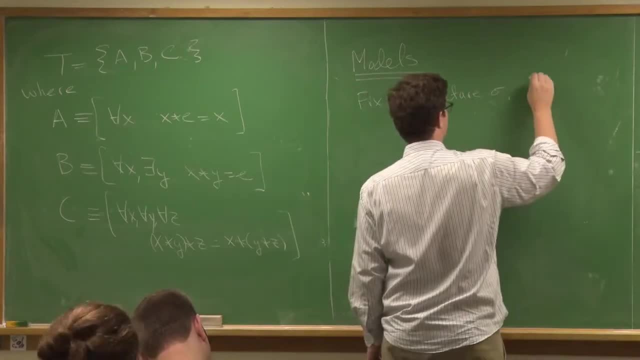 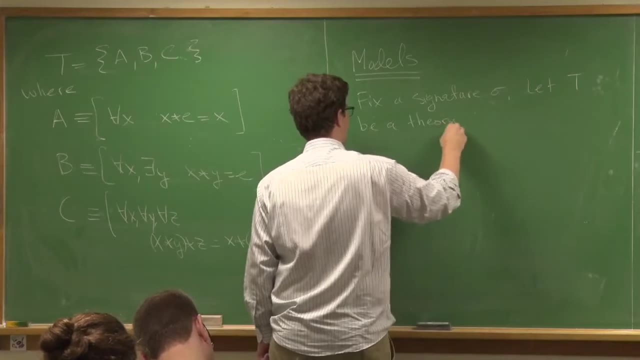 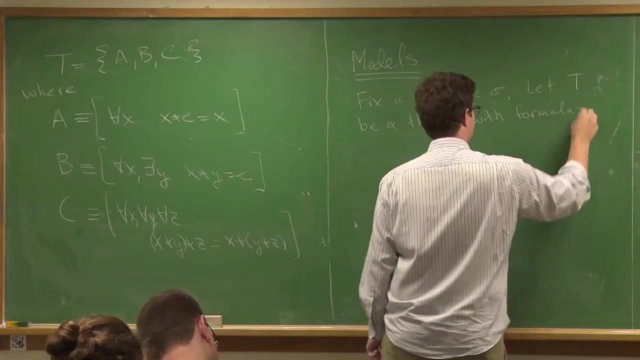 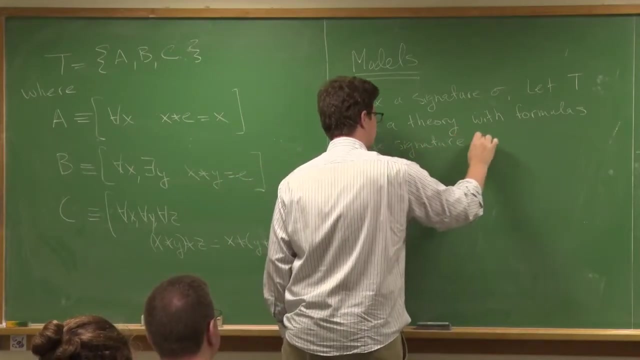 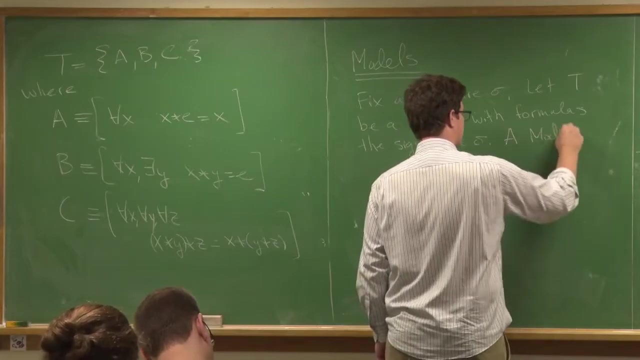 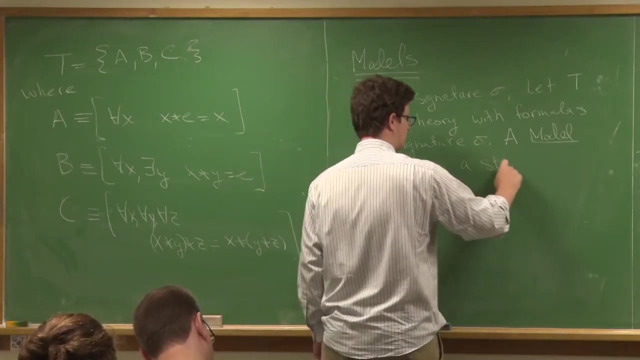 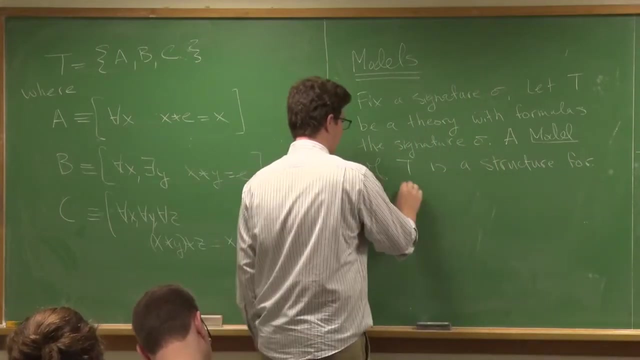 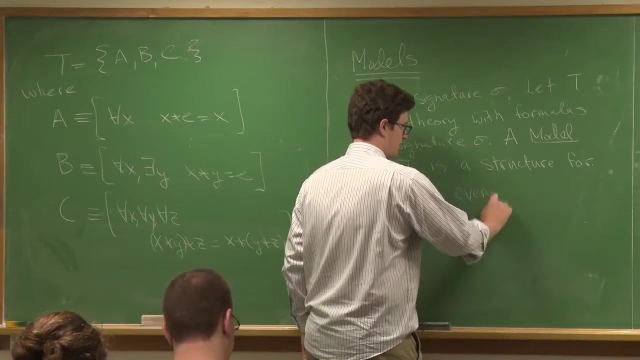 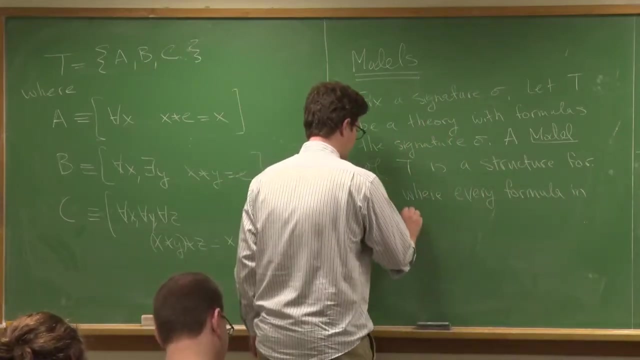 sure, Sigma. so a model, and let t. let t be a theory, theory with formulas. Similarly, u, the model is okay. so a model of t is a structure for Sigma, is a structure for Sigma. so all of our options are the same: s yes, where every formula in T is true in this structure. 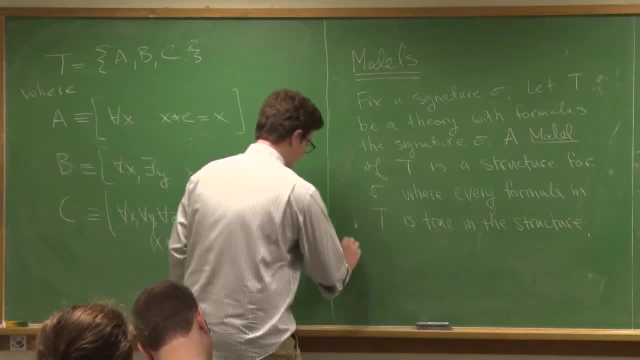 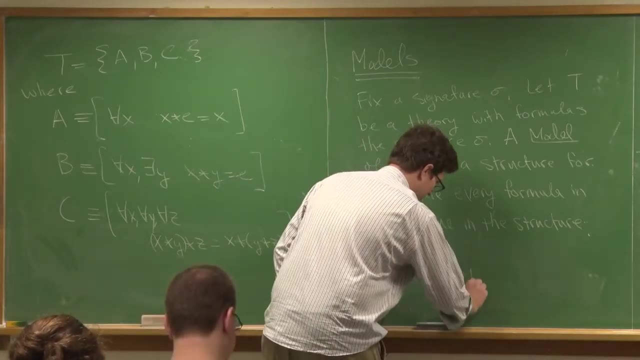 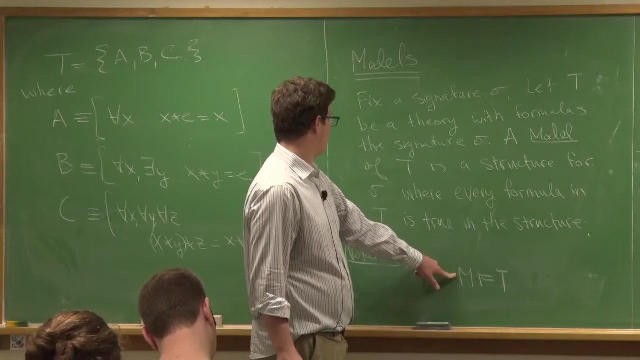 Okay. so there's a notation that we use for this, So this is a kind of a cool logic notation. So we say that M proves T, So it's not just M, right? So when I say as a structure, M, 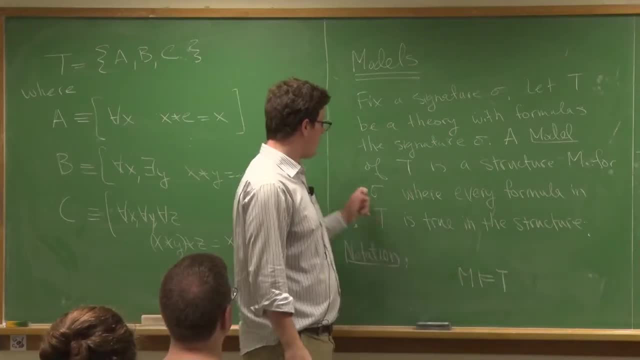 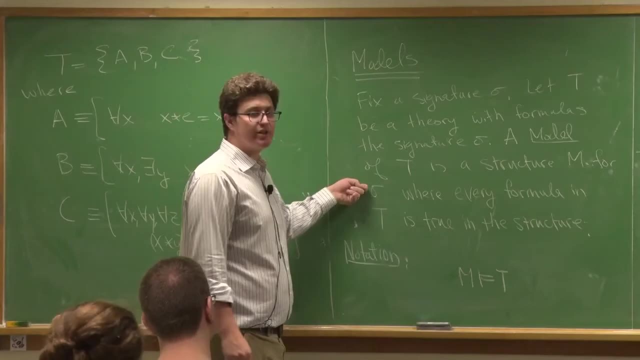 Okay. so when I say M, M really comes with all the data that comes in the signature. So if your signature has a binary operation, your M has a binary operation. If your signature has a constant, M has a special constant in it. okay, 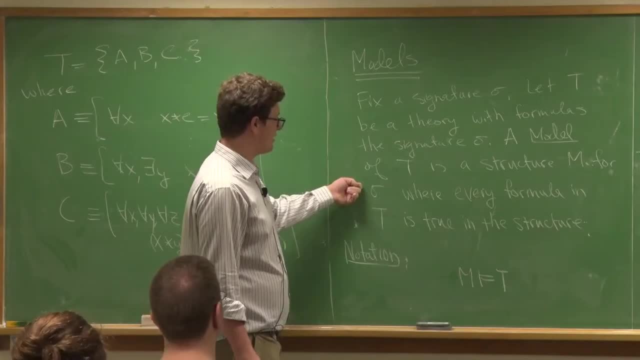 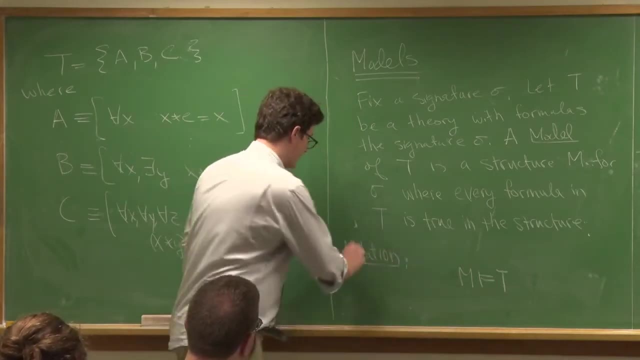 If your signature has a function or, you know, like a relation here, like less than or equal to sign, M comes with a relation or less than or equal to sign, okay, And so this notation is that M is a model of T. 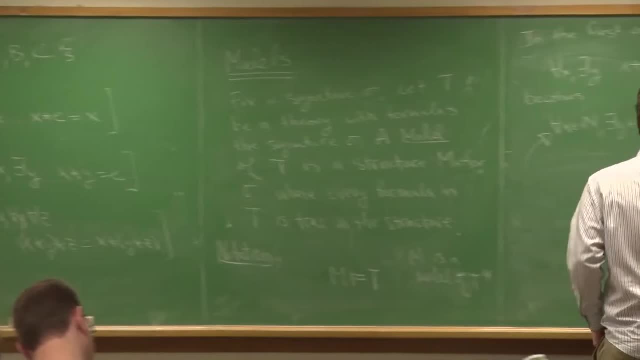 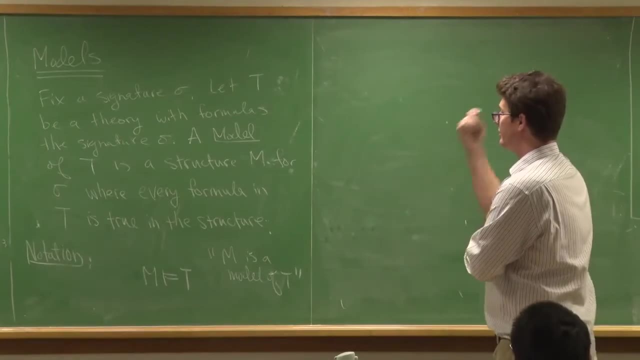 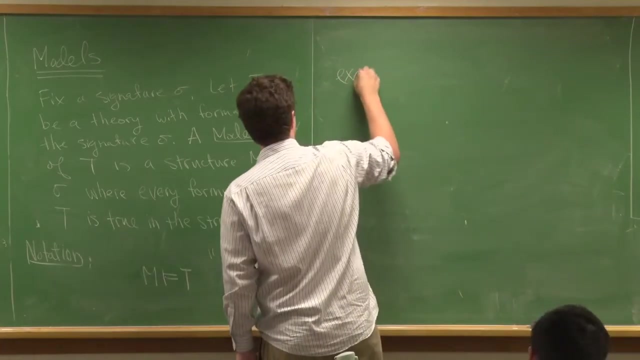 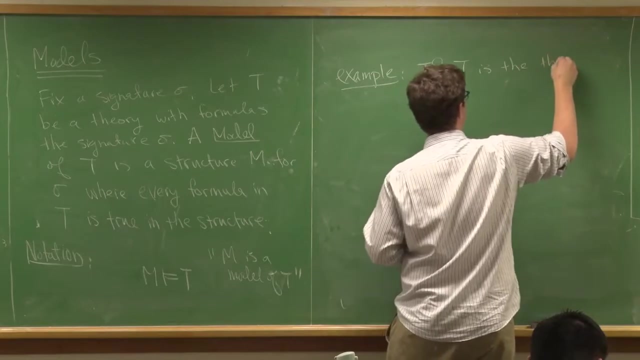 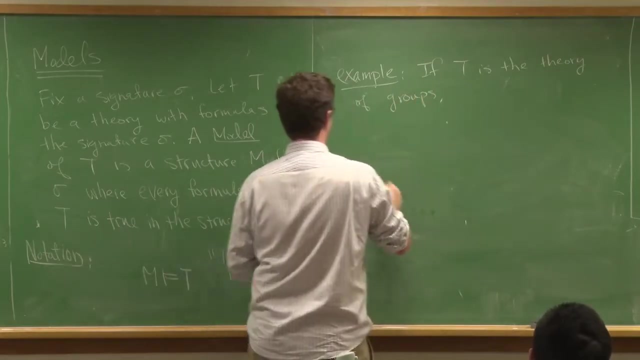 Okay, Okay. So that's what we call. That's What am I saying. So this is what a model is. So, for example, for the theory of groups, if T is the theory of groups, of groups, then these examples here: 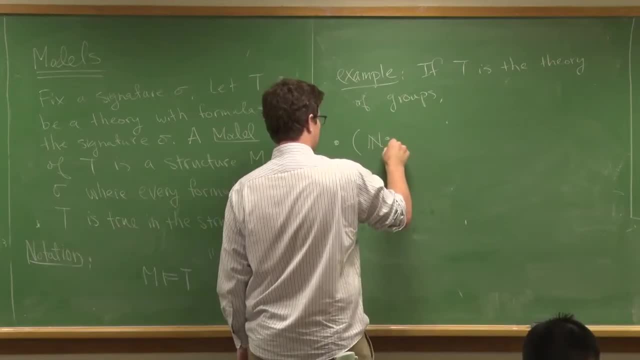 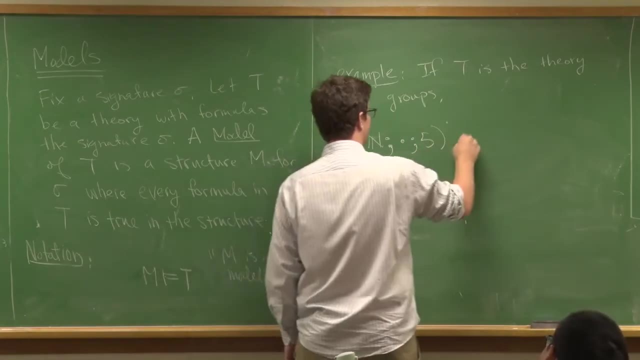 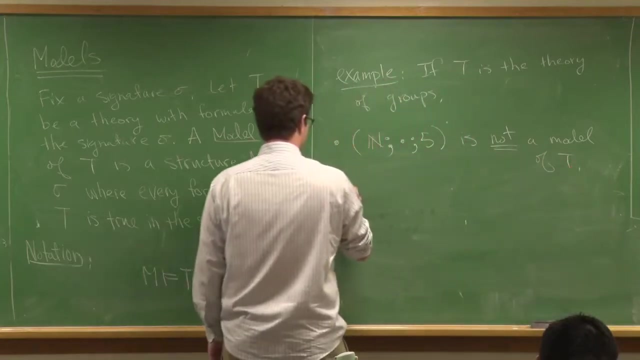 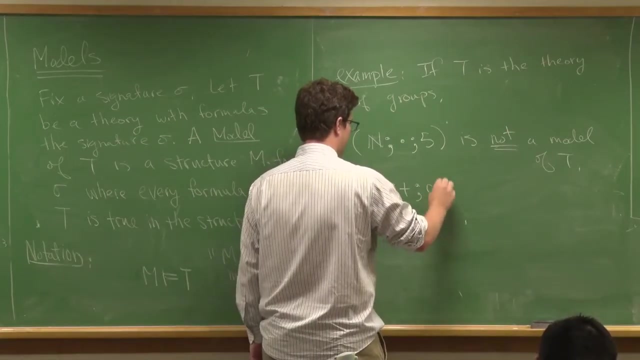 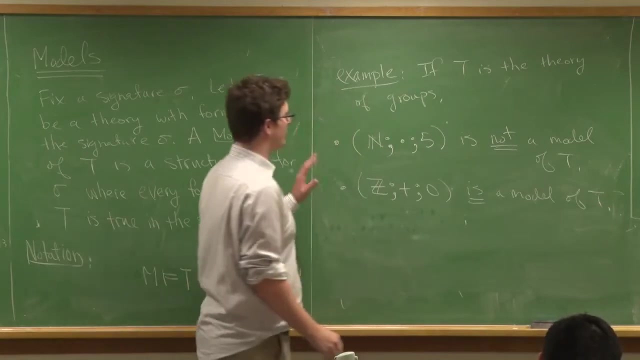 this thing. here we had the natural numbers. with The natural numbers, what did I say? Times and five is not a model of T, right, But this thing- Z plus and zero- is a model of T. okay, Is the model for. 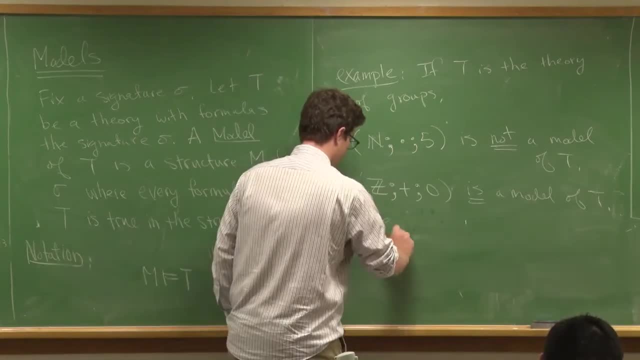 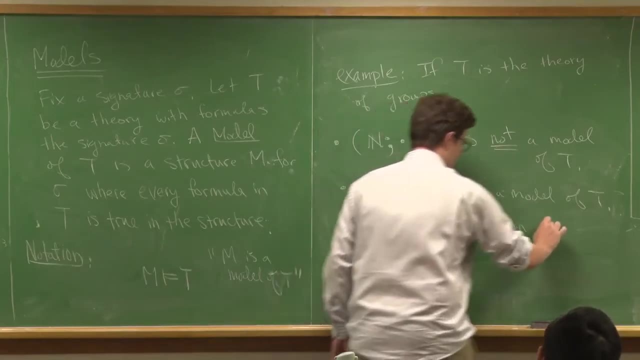 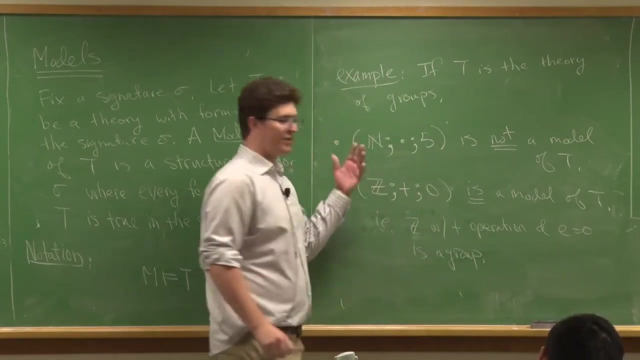 So this is an actual group. ie Z with the plus operation and E being zero is a group. So any model for the theory of groups is what we call a group. okay, That's all that I'm saying. Okay. 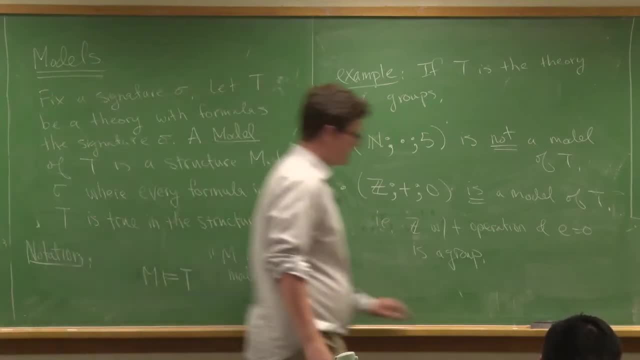 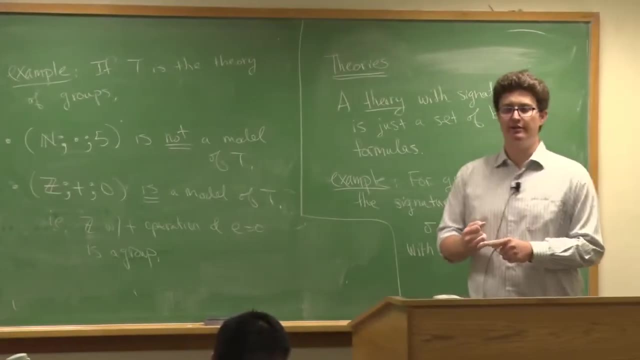 So now let me recap. Let's recap one more time. Okay, So we started with signatures. okay, Signatures are The collection of symbols that we're allowed to make our formulas from, So it's like plus times constant symbols, whatever. 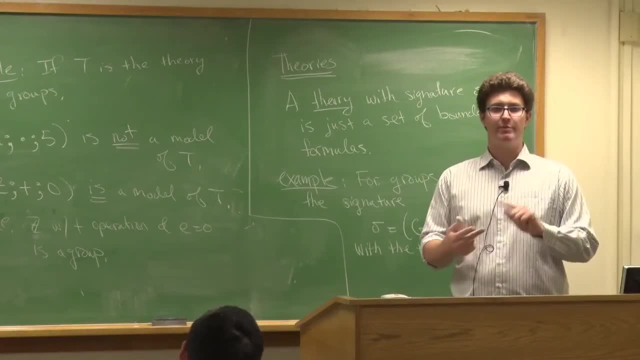 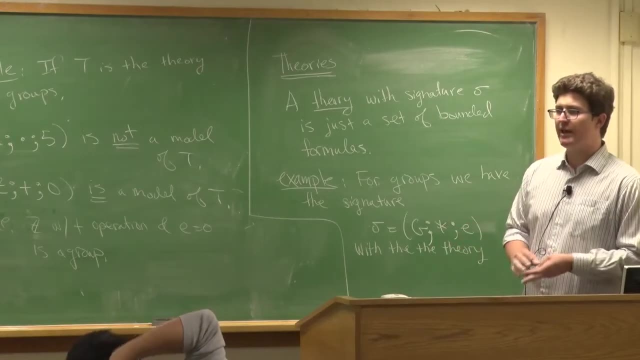 Our formulas are built from atomic formulas. From there we build more complicated formulas by using connectives and quantifiers. All right, Sometimes we allow quantification over subsets. You know, those are called second-order formulas. If we don't do that, then they're just called first-order. 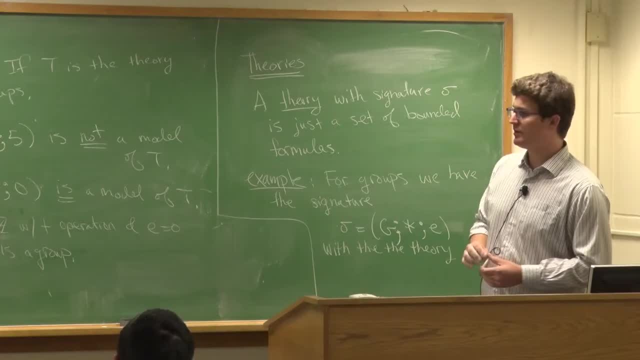 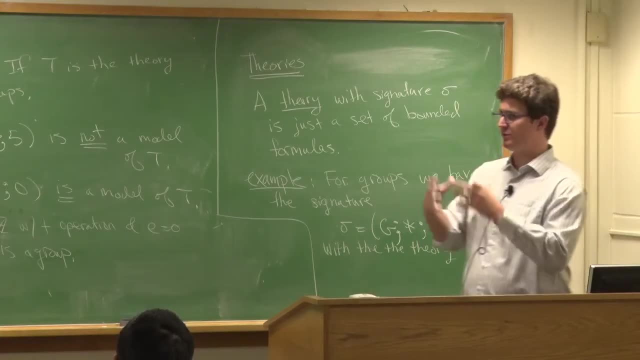 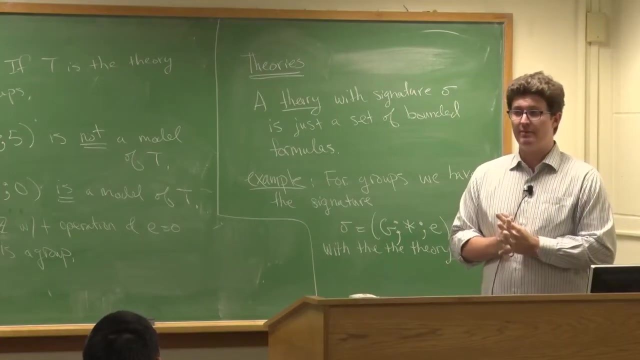 All right. So, given a signature, we have a notion of, We have a notion of a structure. A structure is just a set with some operations which allows us to interpret each of the formulas, The formulas, and it returns true or false. okay, 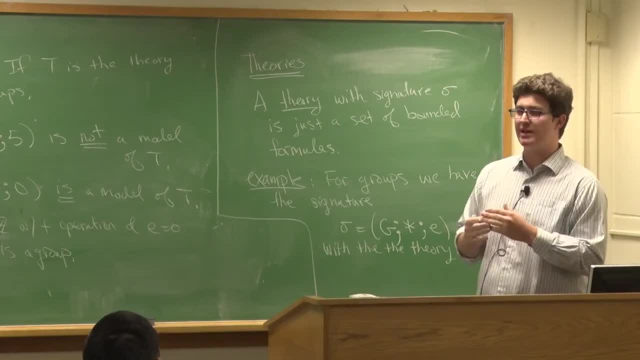 It doesn't matter, you know that they satisfy some axioms. It just means that we can make, We can assign meaning to the formulas. okay, So a theory is just a collection of formulas and a model is a structure where all the formulas 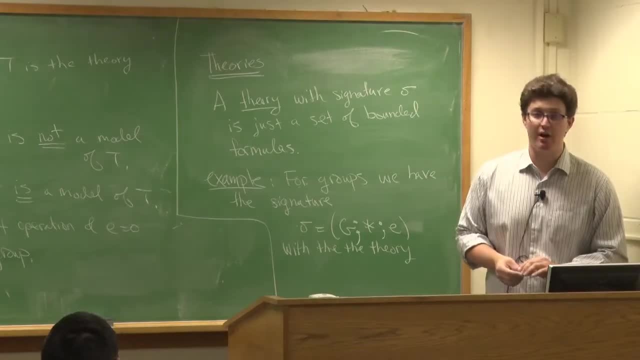 in the theory are true, Okay, That's it. So there's a lot of words, okay, And so in the homework I'm just going to have you guys like, I'm going to give you guys some examples, and you guys are going to say: 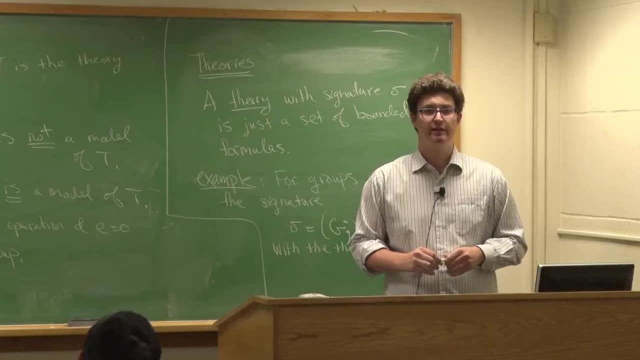 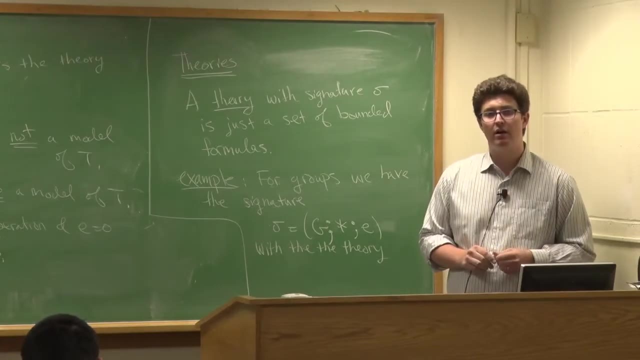 is it a structure, is it a model? right, Things like that? Yeah, So you can have structures that are. So. structures are true or false, right? Yeah? yeah, So you can take a formula and then you kind of plug. 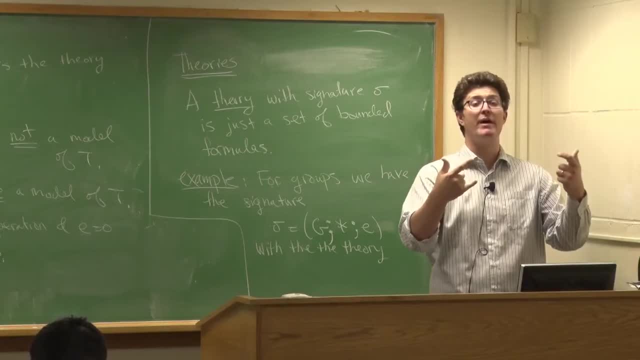 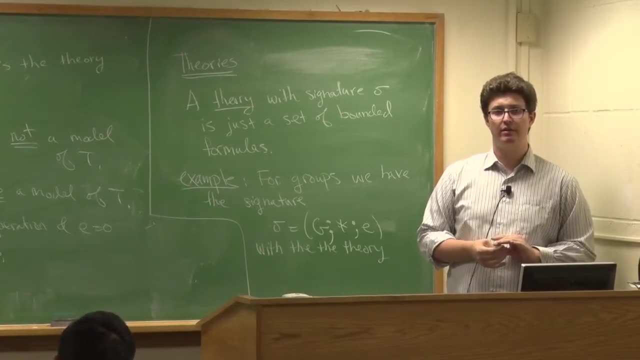 in the model, into the formula, and it'll say, okay, this Like for a bounded formula, right? So this is a proposition. right, It'll return true or false. Yeah, So you can have a structure and a model of something. 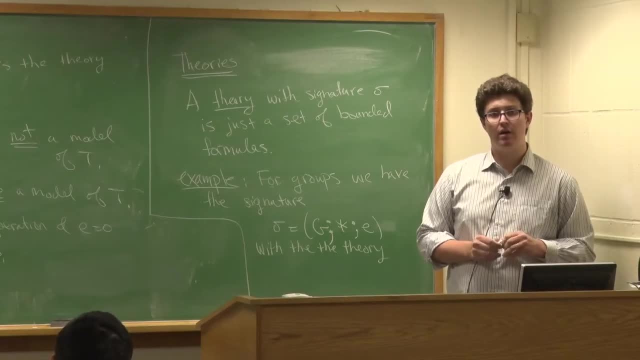 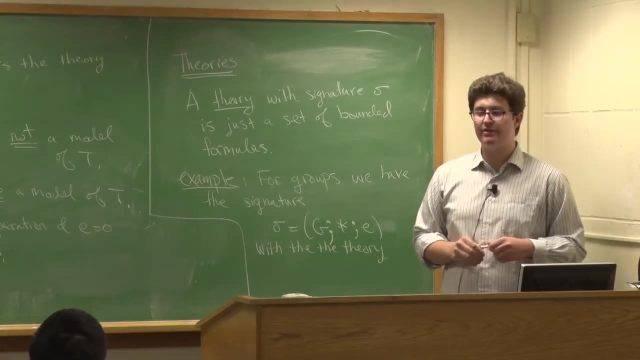 that abides by groups. but until you have, Until you like, imply the theory of groups, it doesn't. I don't want to say it doesn't matter, but Yeah, I mean. so, for example, every model is a structure right. 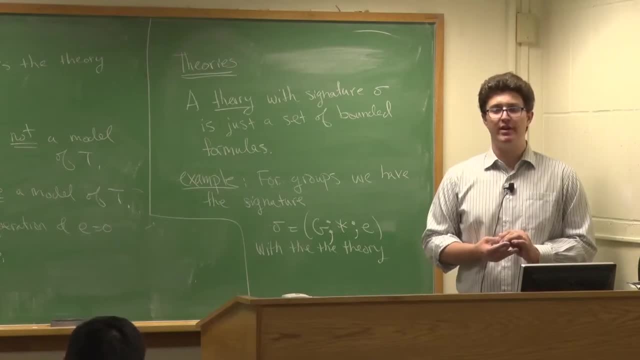 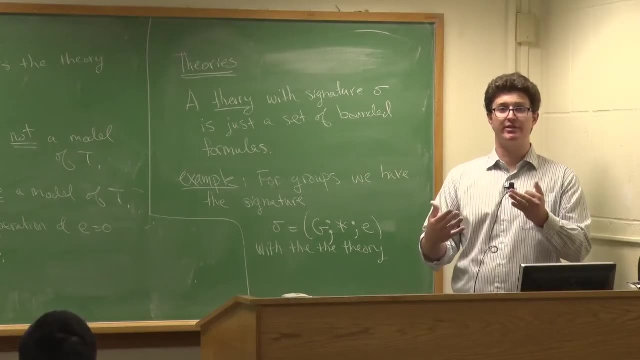 And so there are certain things which I can check the. So if it makes sense for me to check the axioms of groups against this thing, so then that's a structure right for that signature right. It makes sense that I can like: okay, does it even parse? 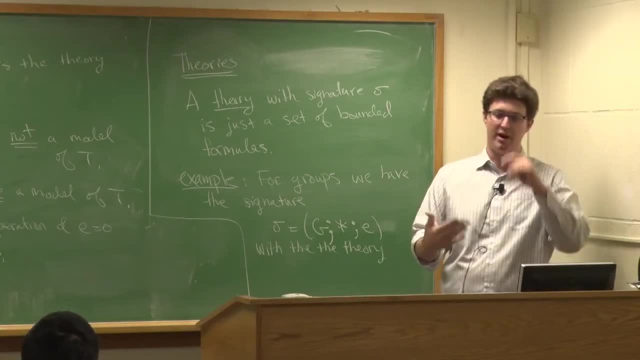 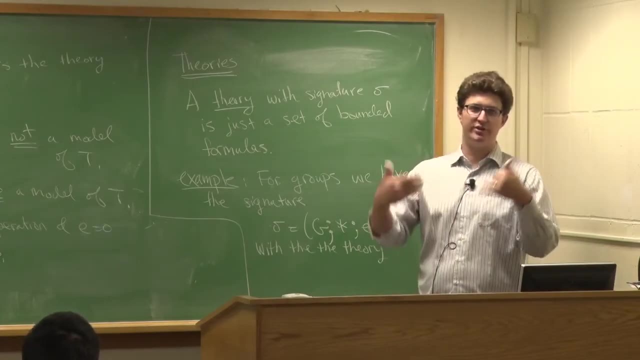 that this thing could be a group right. Does it have a binary operation? Does it have something that you called the identity right? Well, you know, then, that's a structure and you can check it and the axioms will fail right. 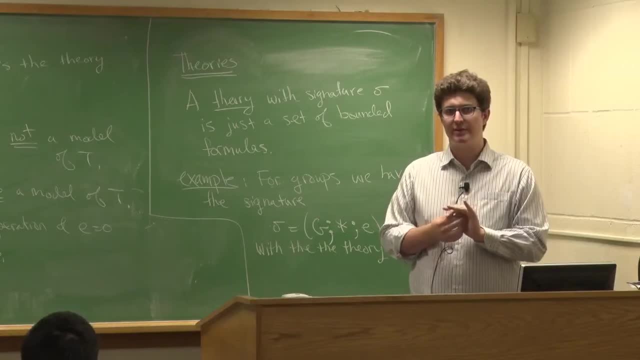 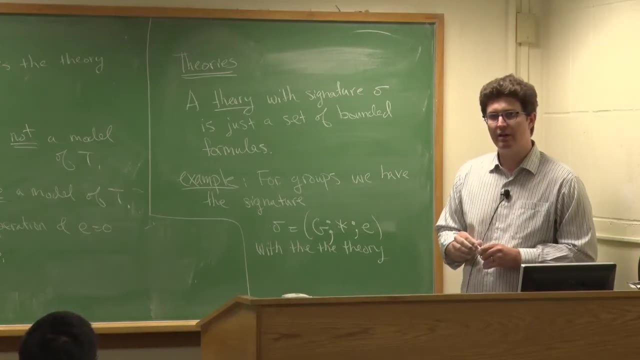 Or if it is a model, then the axioms will be true. Does that make sense? Yeah, Yeah, I don't know if I clarified what you were saying, but yeah, Yeah, Do you think the P-ignition theory and structure? 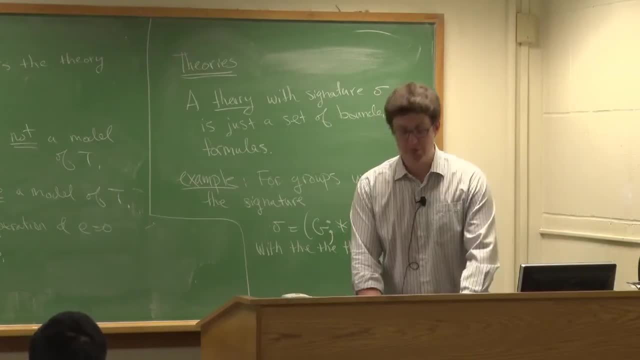 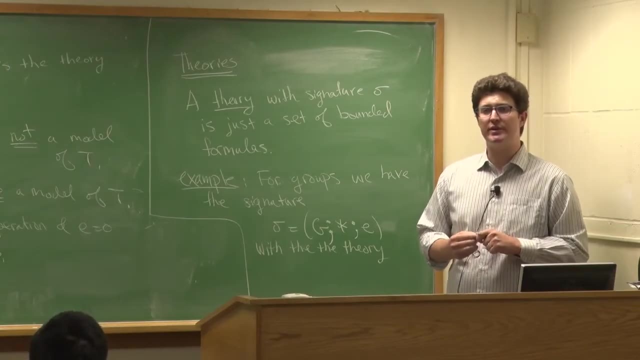 Okay, yeah, so a structure. right. so a theory and a structure are different, right? So a theory is just a collection of formulas that you build, right? The difference between a structure and a model is that, so models. so for a model, for a structure to be a model, 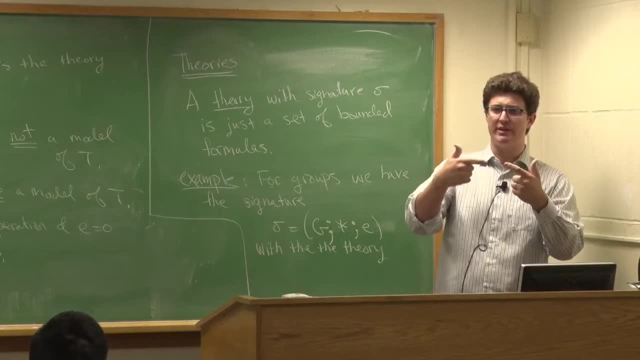 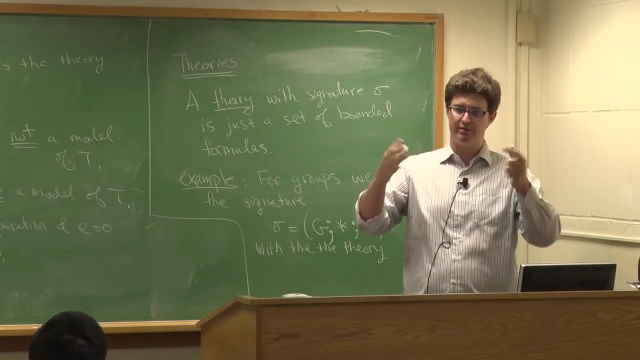 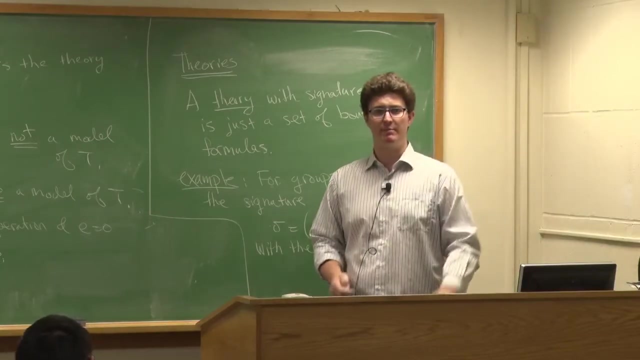 of a theory. you need every single one of the formulas in the theory to be true when you investigate it for that particular structure. So a structure is promoted to the rank of model if it verifies the axioms. So once you verify the axioms then it becomes a model, right. 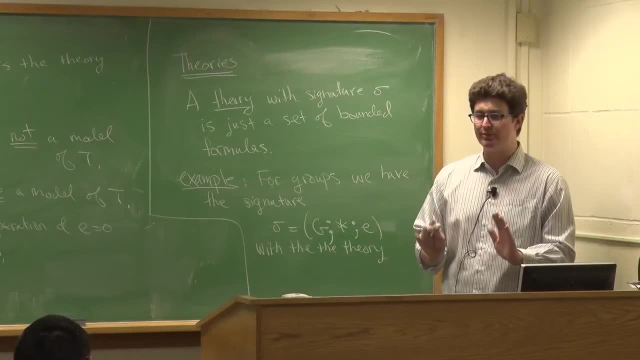 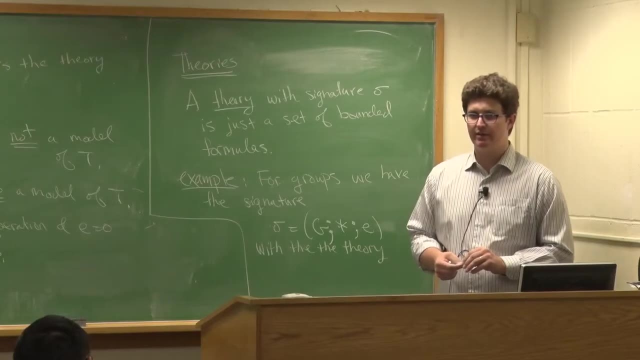 So, for example, in the theory of groups, if you have an actual group, that's a model for the theory of groups, right? So it's true, like if you have a structure and then you check your formulas and it turns out to be true, right? 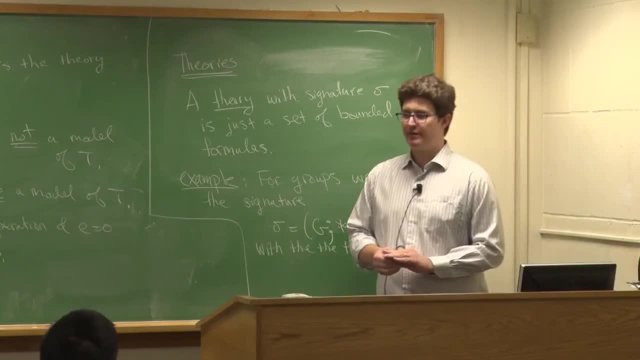 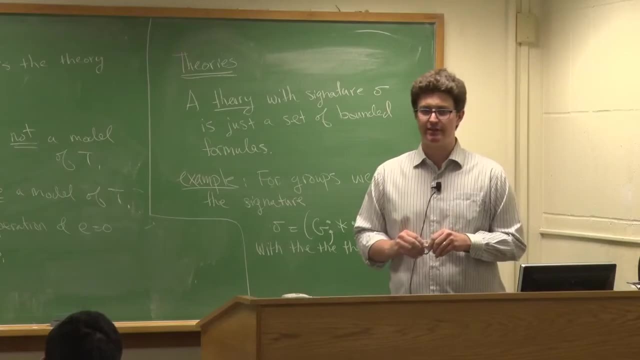 If it turns out to be true, then it becomes a model. yeah, It you know passes and it you know you need to call it a model. So it's just a lot of words, right, But these words allow me to say things more succinctly. 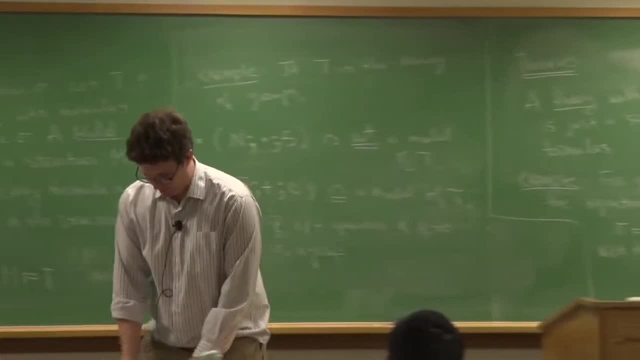 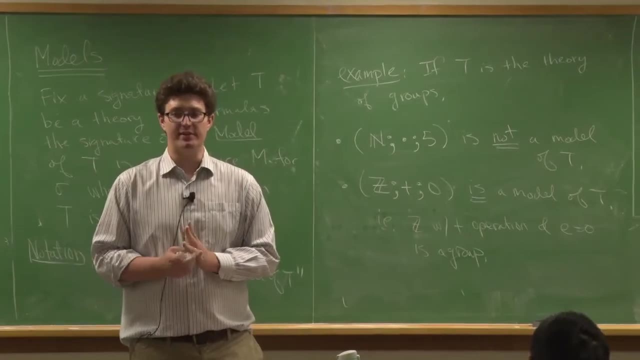 like okay, like the reason why I introduced all these words is in order to talk about the difference between the Dedeckin, piano axioms and piano arithmetic, And the key difference is the signature. okay, And some people and the way that you can formulate. 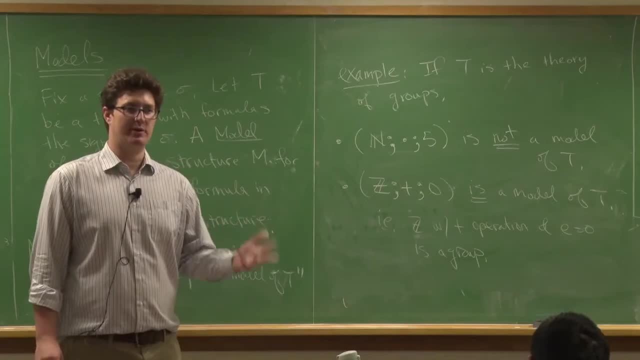 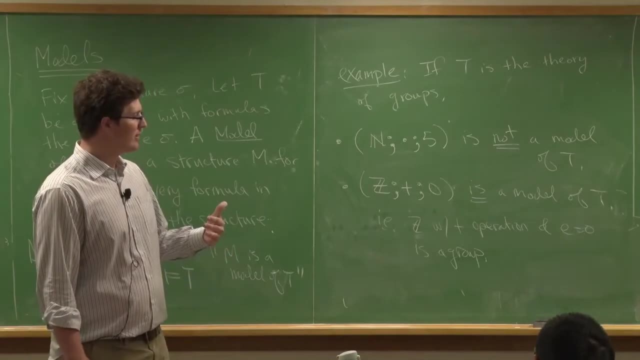 the axiom of induction. okay, Piano arithmetic is the famous one, the famous set of axioms that, you know, the incompleteness theorem are about. okay, And so, in order to talk about that precisely, I wanted to introduce some of this terminology. okay. 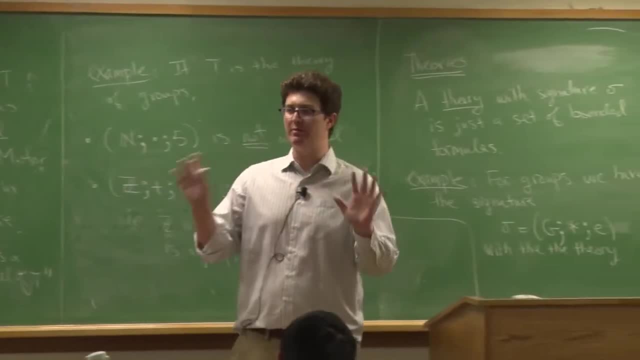 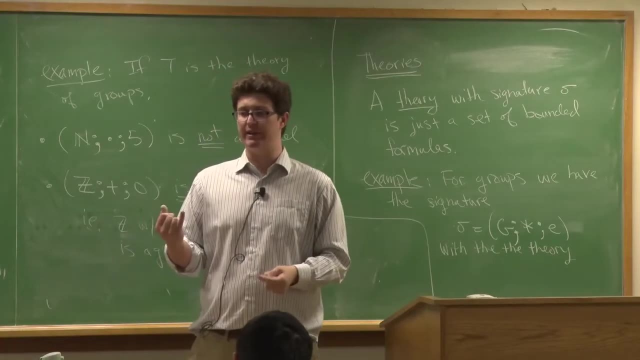 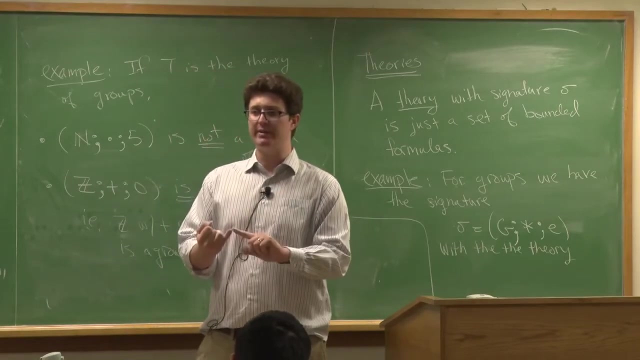 And so, and in the background of piano arithmetic, which are these axioms for the natural numbers which have a larger signature? so, originally, our signature for the Dedeckin piano axioms just had the successor function and a constant element right. and now for piano arithmetic. 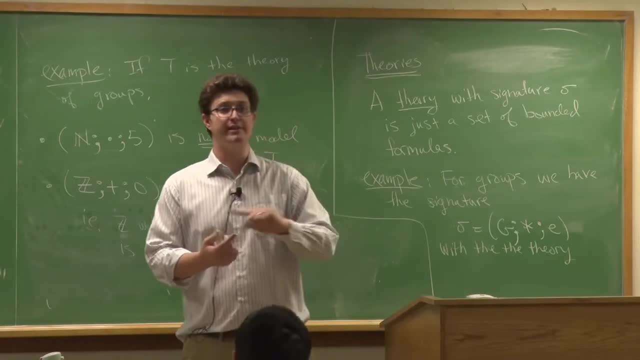 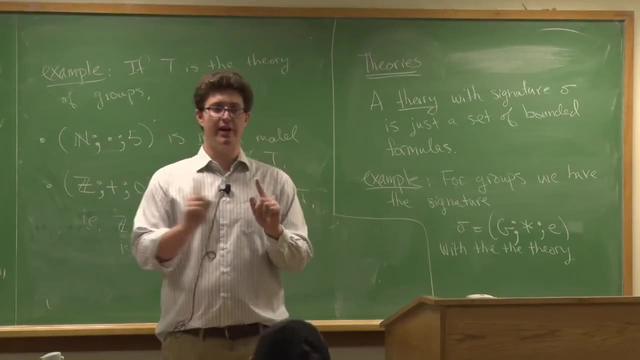 we're gonna have a successor function, a constant element, but we're also gonna have plus and times. okay, And so plus and times allow us to say more. in particular, talk about the ordering of the natural numbers that we needed to in order to say that strong induction. 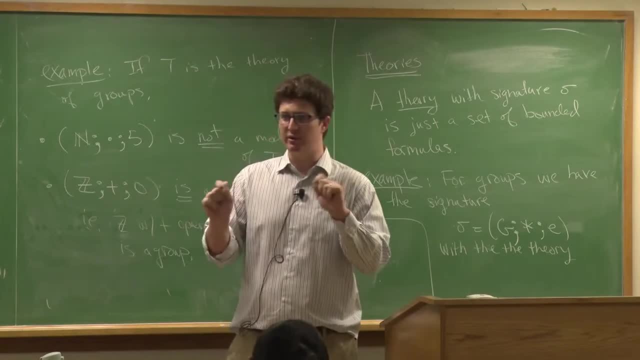 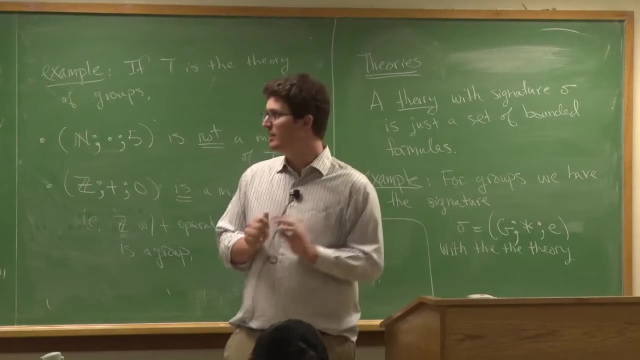 and weak induction were the same Because, remember, I was using the less than or equal to sign everywhere. but I didn't, you know. I told you I was cheating right And that cheating was because I was using something that wasn't in the signature of the theory. 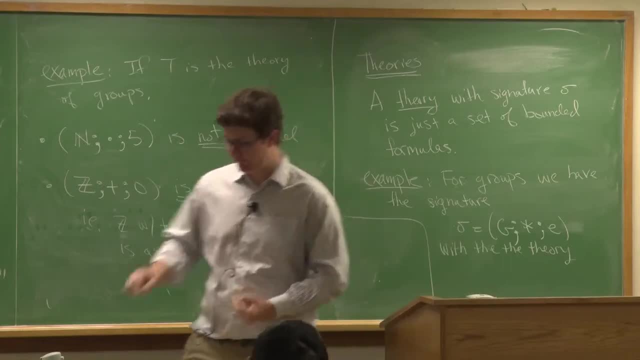 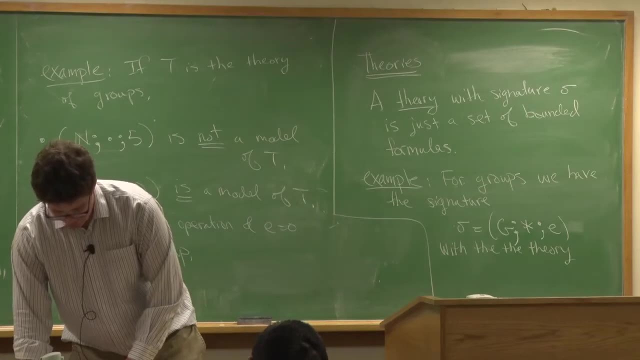 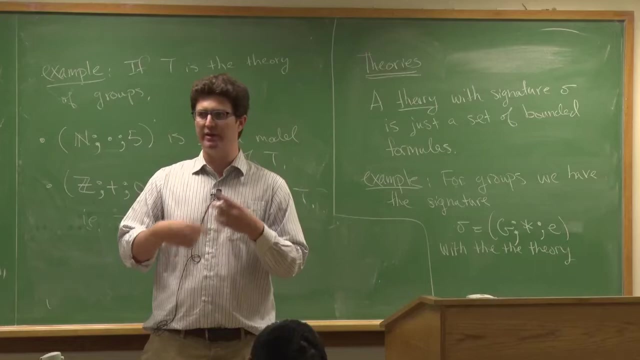 Okay, So technically that's what was going on. So, so what time does this end? Seven minutes, okay, So let me. so what I'm gonna do is I'm gonna write down the axioms for piano arithmetic and then next time I'm gonna explain. 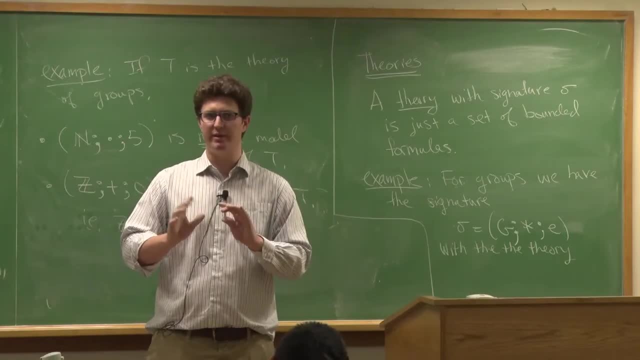 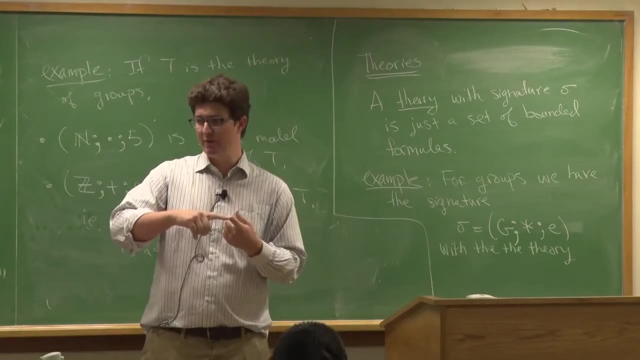 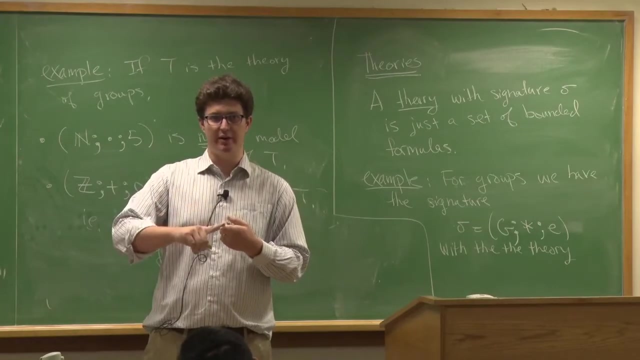 how the Dedeckin piano axioms and piano arithmetic are different, And so I guess next time will mean you know the generalized next time, because we have review right And then on. so we have review next class and then on Monday you don't have class. 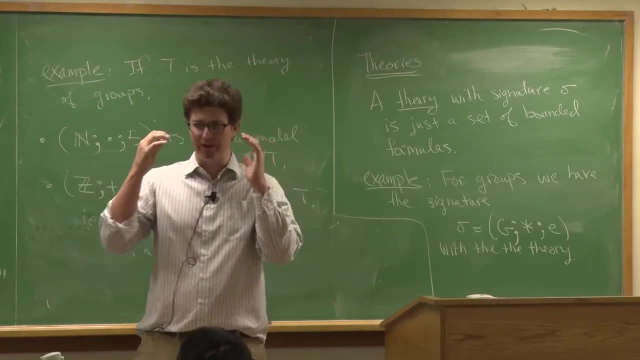 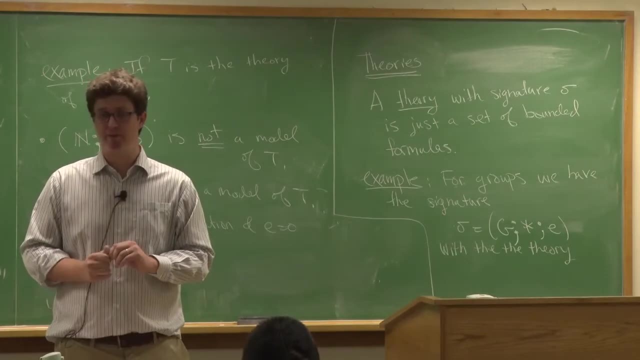 and then on Wednesday we have the test, okay, So you'll have to, like, hold on to this kind of hard for next time, and I'll do a little recap before. so I guess it'll be next Friday, right? So it'll be like a little while. 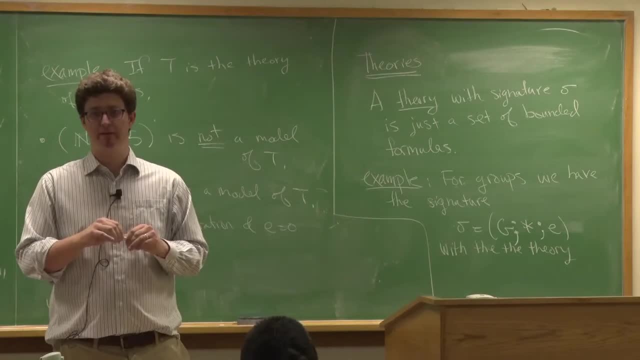 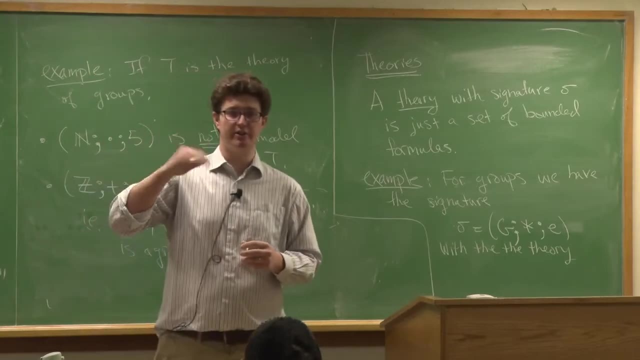 before we actually get into this. Yeah, Evie, Oh, So for the exam it has like what chapters We're going over? just non-induction. so up to chapter two. Oh Yeah, yeah, yeah, yeah. 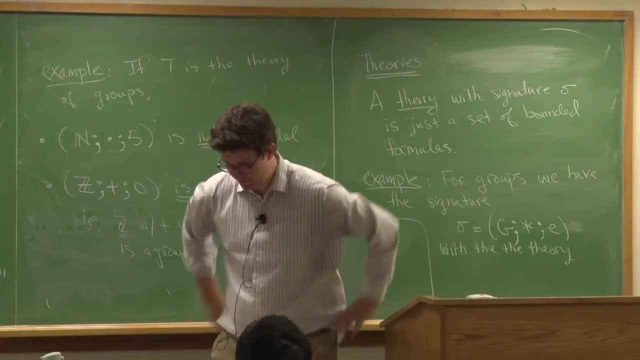 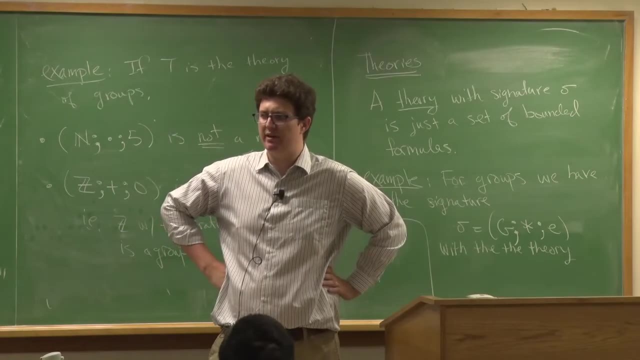 And so, yeah, before I write these things down- so I'm gonna, so I started writing the test, right, I need to throw out some questions, and so I'll make those- the ones that I throw out- available to you guys, right. 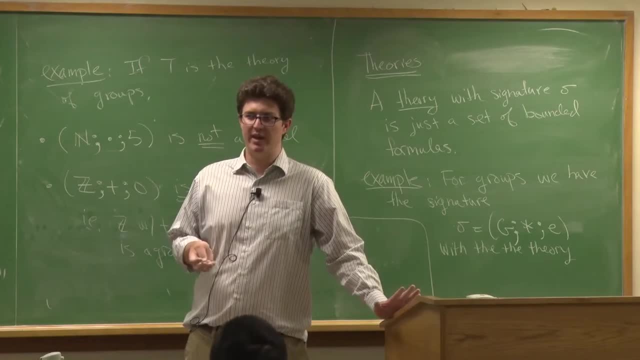 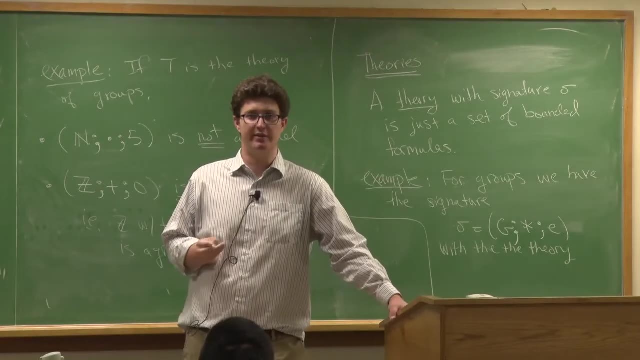 You know. so you can kind of see what type of things I was thinking about. And then I found some practice exams from another old Math 52 class that I'll make available to you guys. okay, Yeah, How group-centered is this exam going to be? 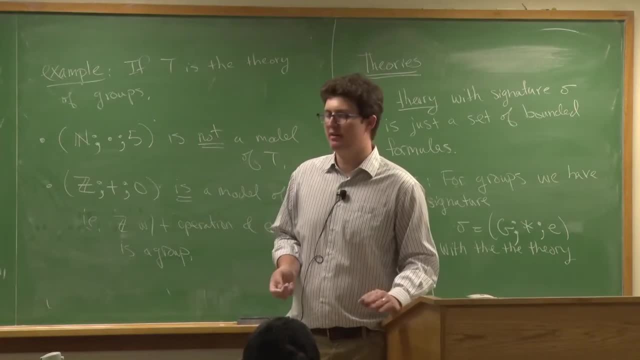 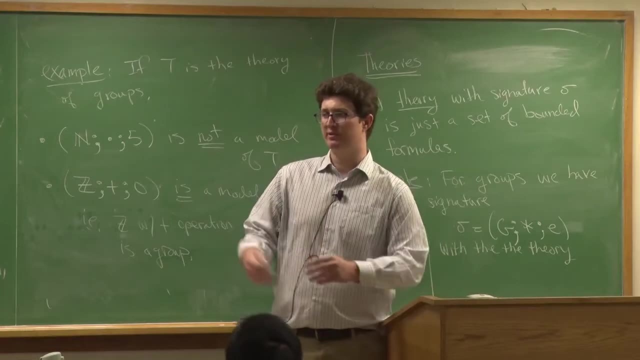 I mean not very, you know, Like it's part of the class, right? And the reason I gave you guys multiple group questions because, like on the homework- is because you guys didn't do so well the first time, so I wanted to make sure that you did it. 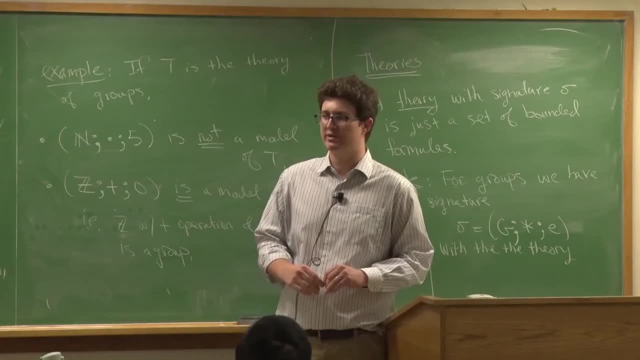 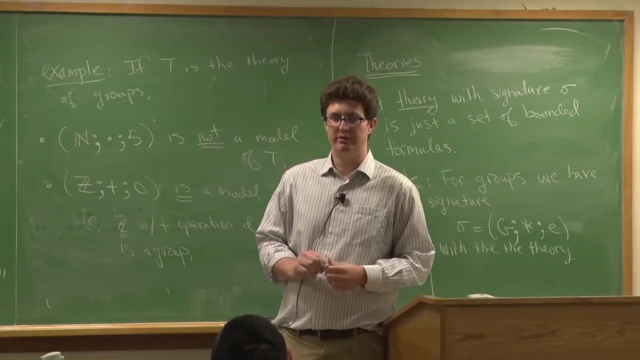 So I mean, if you go do the handouts and the homeworks, they should be sufficient, you know, Yeah, Is there a difference in the capitals in any of those chapters? One and two? One and two? Yeah, yeah, chapter one and two. 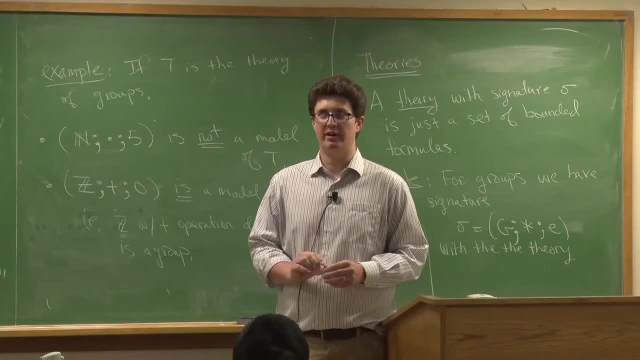 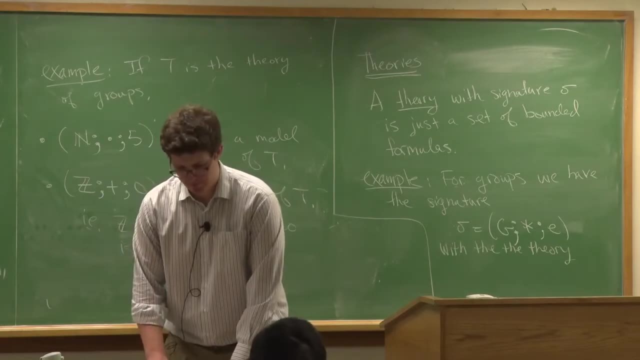 Is that for any of your multiple pages? The book is Laken's, so it was the one on the course description or the syllabus. Yeah, we can talk about this after, if you want. Okay, so let me write down these axioms. 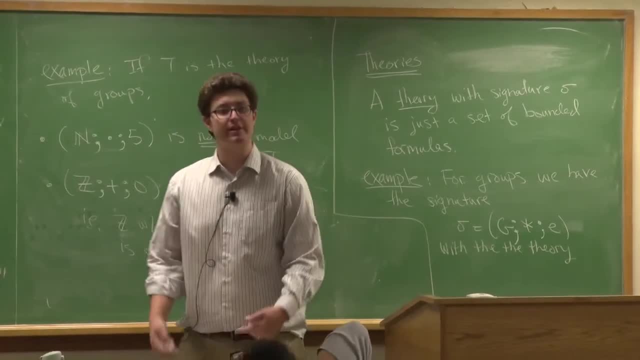 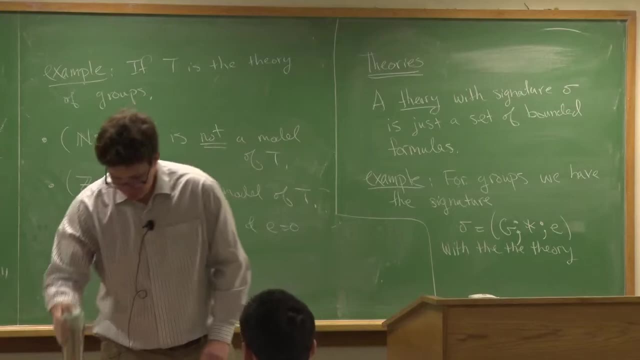 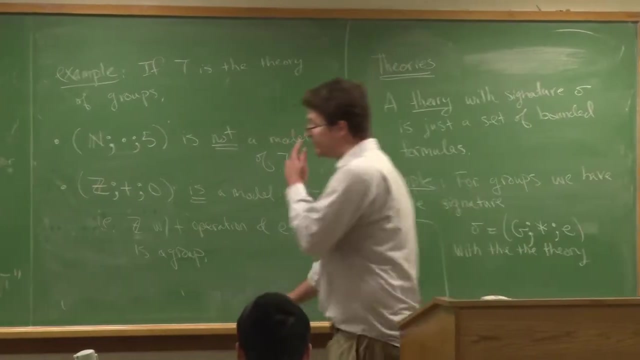 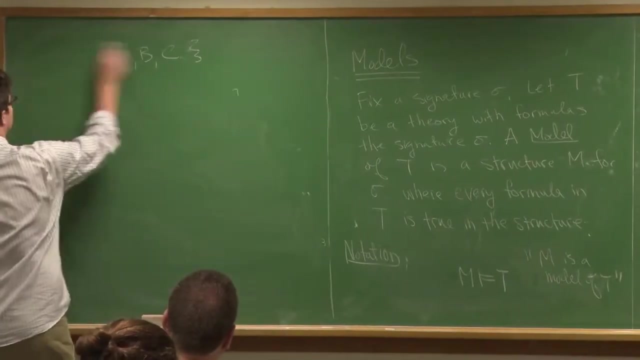 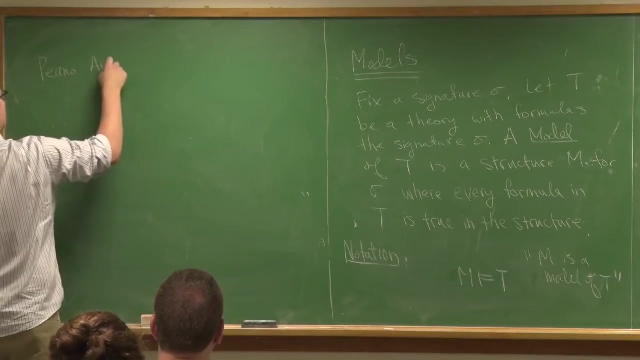 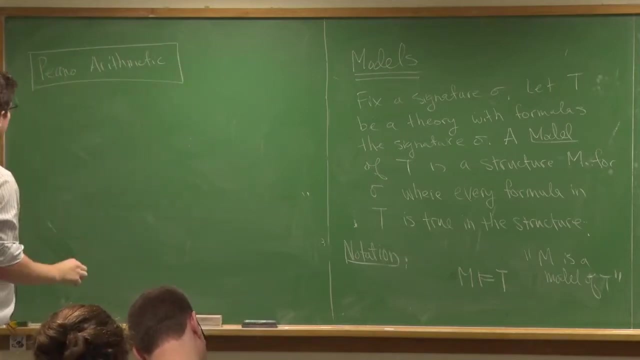 for piano arithmetic, and then, if you have more questions about the test, you can come ask me after class. okay, All right, Okay. so for piano arithmetic you have to use the axioms, right, Okay, Okay. so here are the axioms. 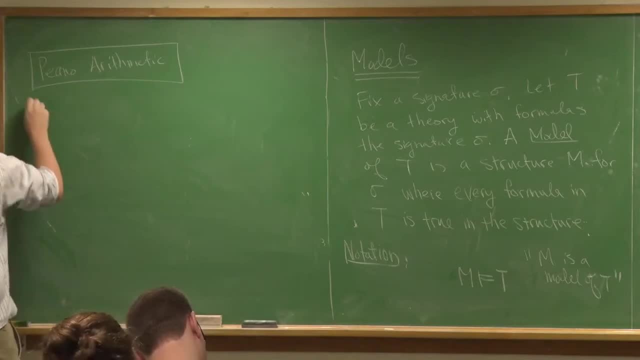 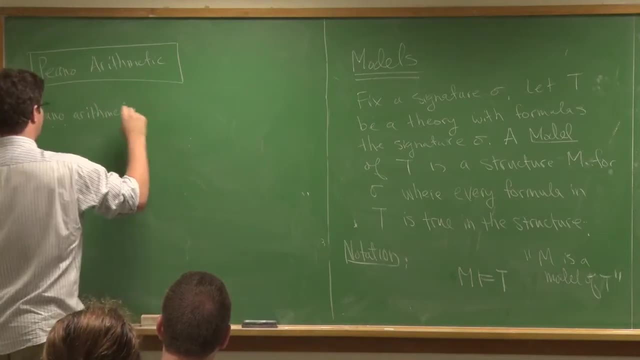 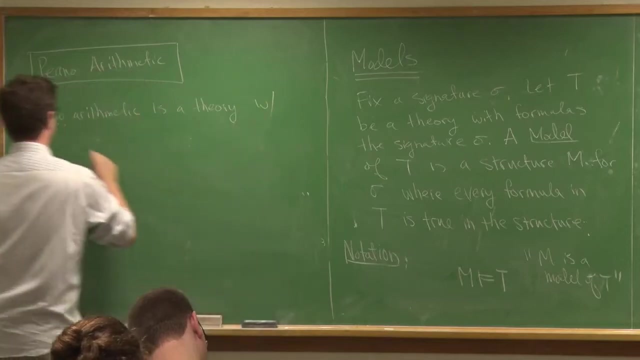 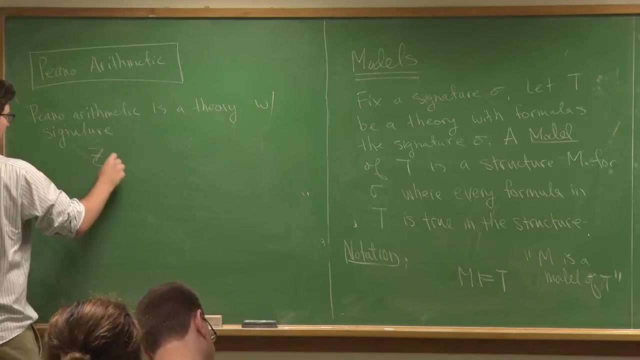 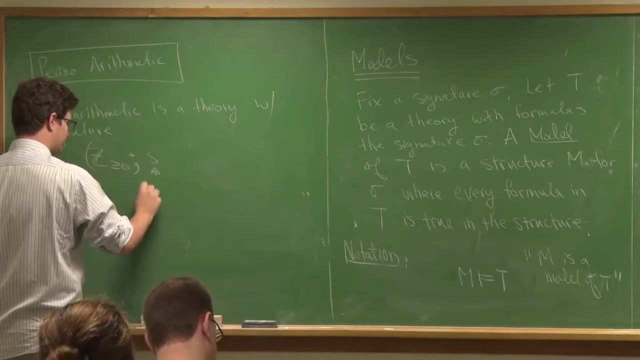 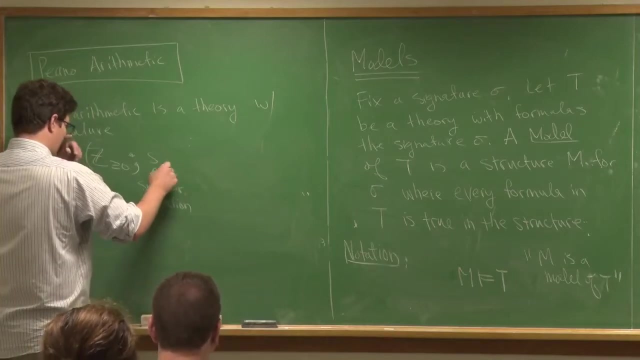 So the So piano arithmetic is a theory with the signature, okay, so we have, so I'm gonna, so I'm going to do this, so I'm going to include zero, okay, and then we have this guy. so this is the successor function function, right, and then we're gonna have two new function. 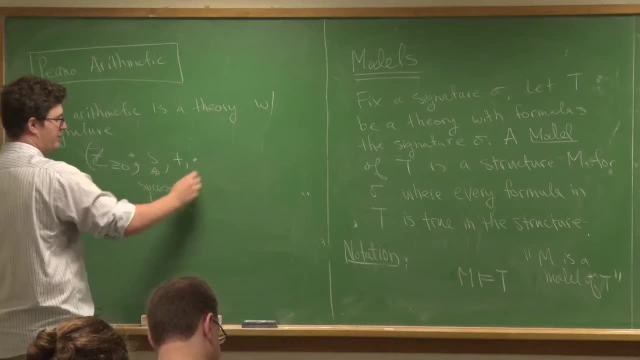 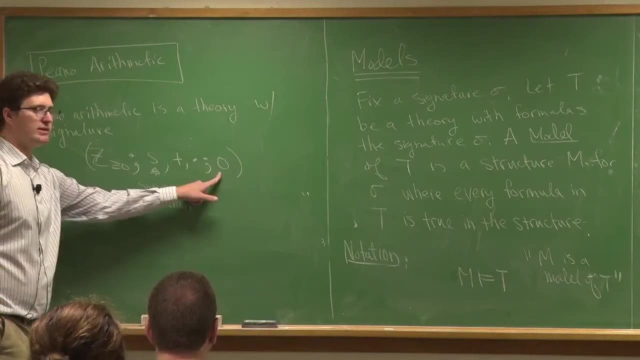 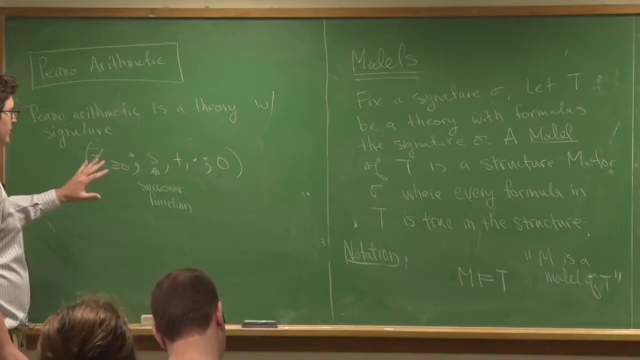 new, two new operations: right plus and times, and then we also have two constant symbols, or no one constant symbol. we're just going to use zero. so this will be the starting point and it'll it'll serve the purpose of the, the, the identity for addition. okay, so it has this signature and and it's 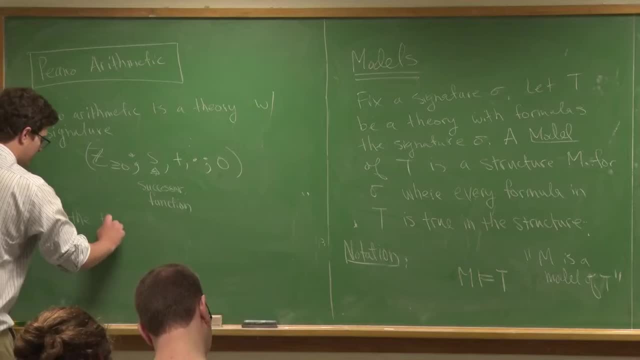 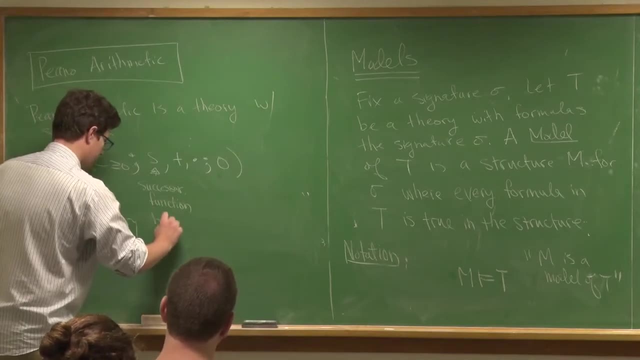 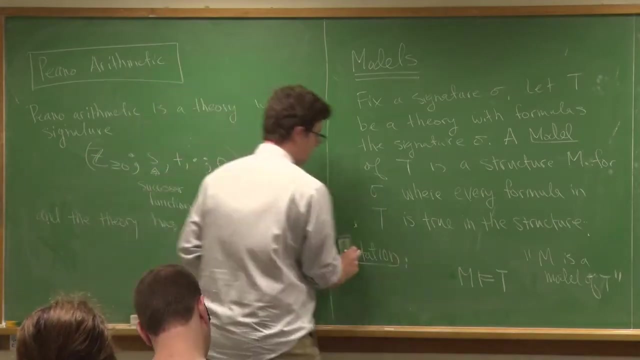 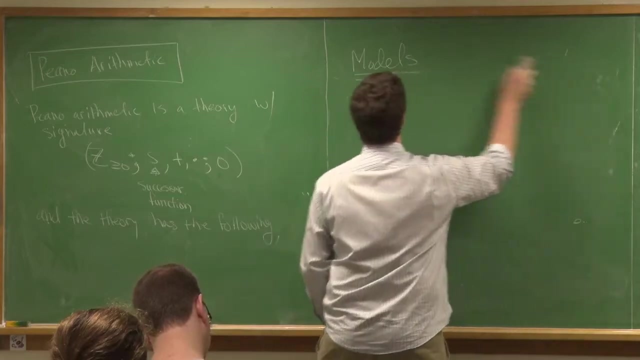 satisfying wise theory contains the following formulas: okay, and I'm going to list some of them that are actually contained in the signature. so, as you guys might remember that, I wrote down three axioms for groups right in this in today, right, but you had to check for right, the really the fourth axiom. 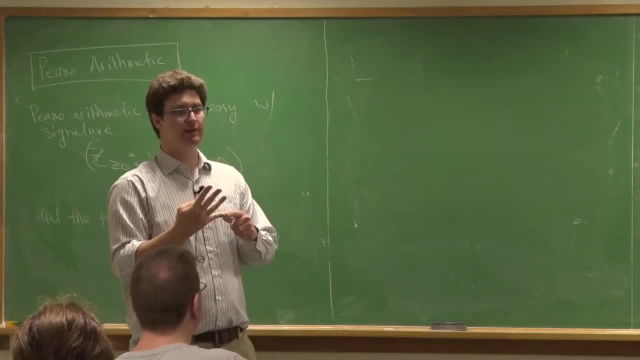 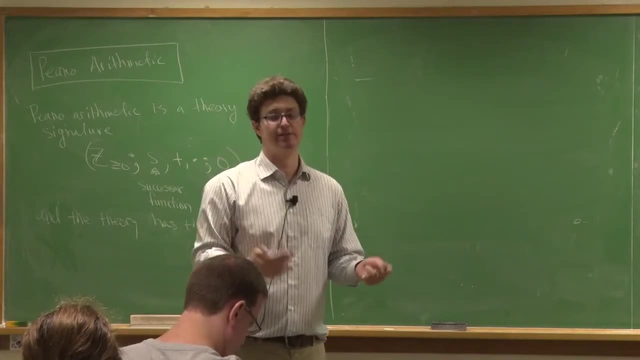 is part of the structure. okay. so the fourth axioms, that the thing about the closure- right, that's why I didn't include it the first time, because it's actually part of the structure. okay, but it is something that you need to check. so so you get. so some people can call it an axiom if you want, but technically, 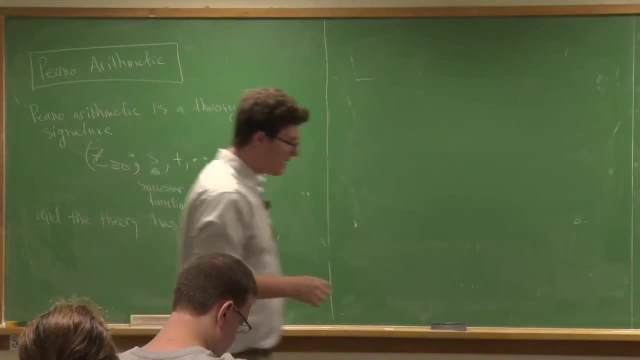 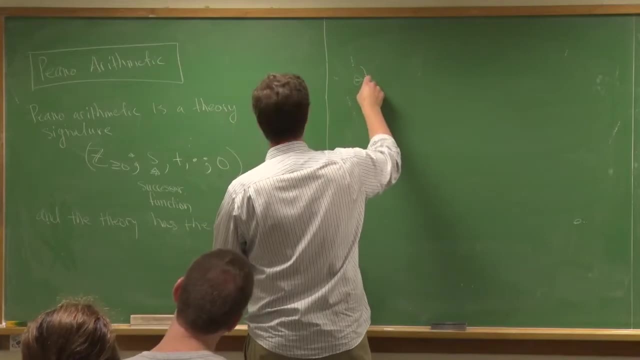 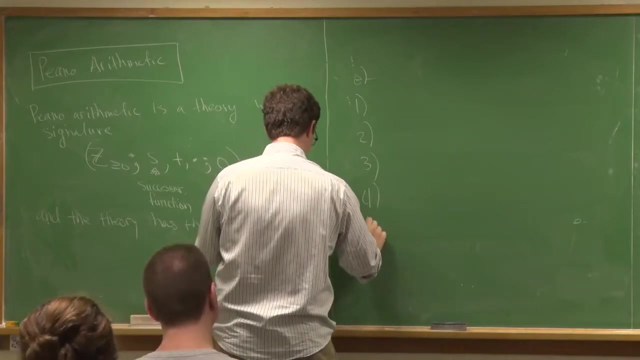 it's part of the structure, okay, anyway, I'm going to write down what they are so here. so here's: there's going to be eight axioms: zero, 123, 143, 126, 5, estás, 128, four, five, six, seven, okay. and then there's this induction axiom which will 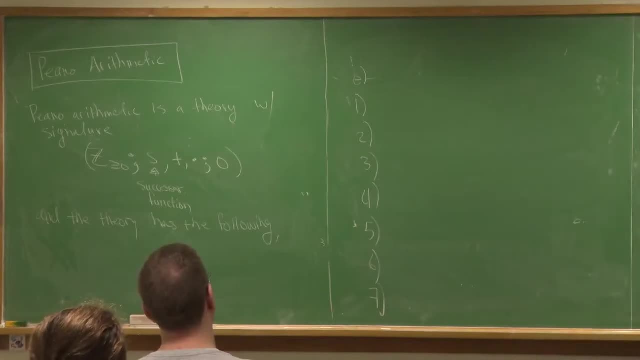 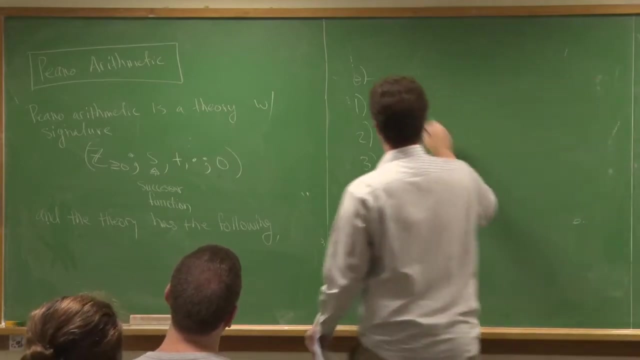 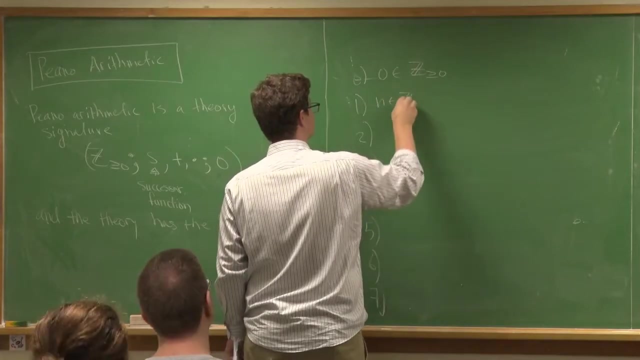 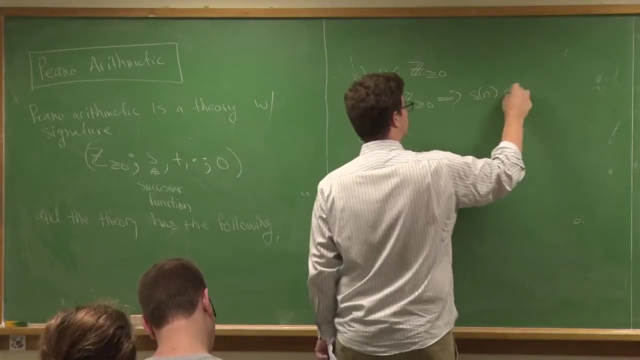 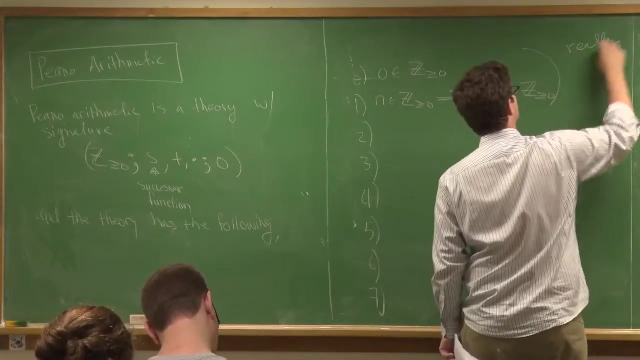 be over here. eight and okay, so the zero, that. so these two axioms are not really axioms, but they're part of the signature. so if n is in here, this implies sn is an element of here. so these things are really part, part of the structure, so you could omit them. 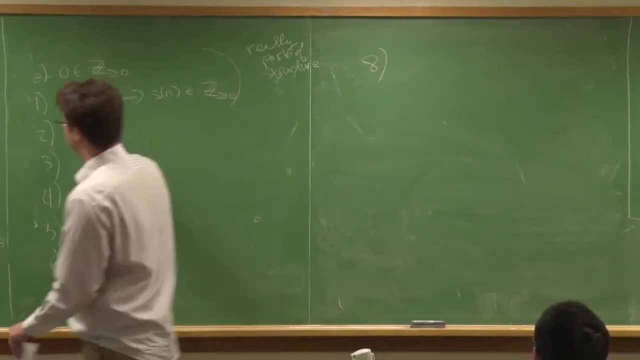 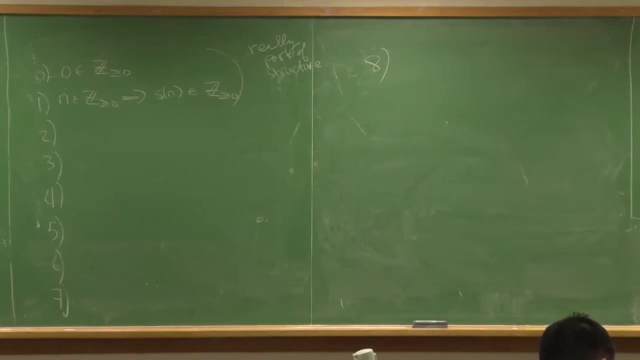 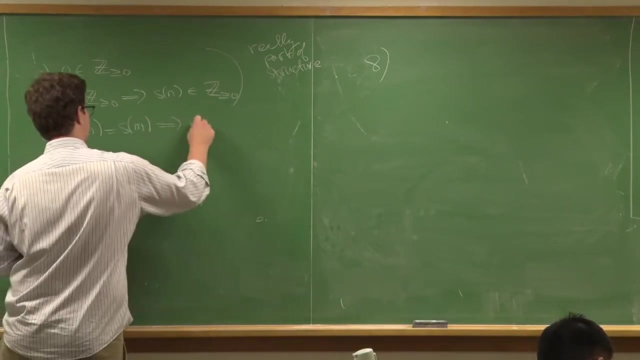 once I once I specified the signature. technically, you don't have to write those down. okay, now that we have this language of signatures, okay, the verbiage here, but we do have to write down these. if this is true, then n is equal to M. right, we already. 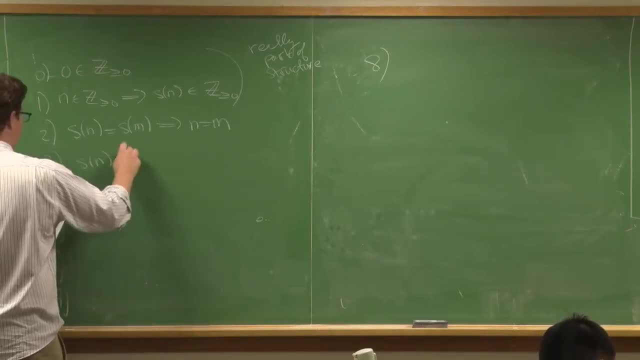 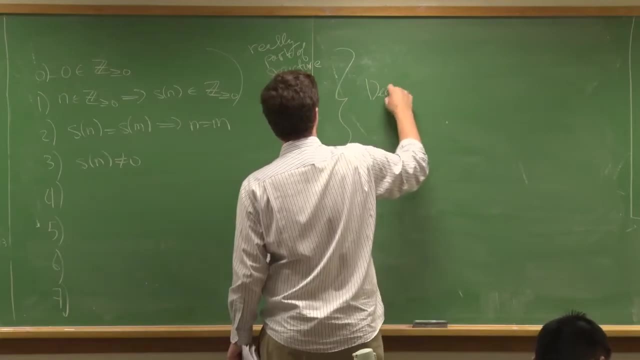 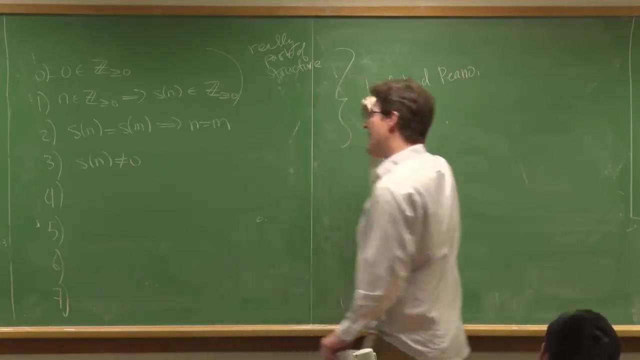 wrote that one down and then we had that for all. n sn is not equal to zero. so these ones here, let me. let me just say this here: so these were the Dedekind piano things, Dedekind piano, and now we're add these new axioms here which allow us to talk about multiplication. 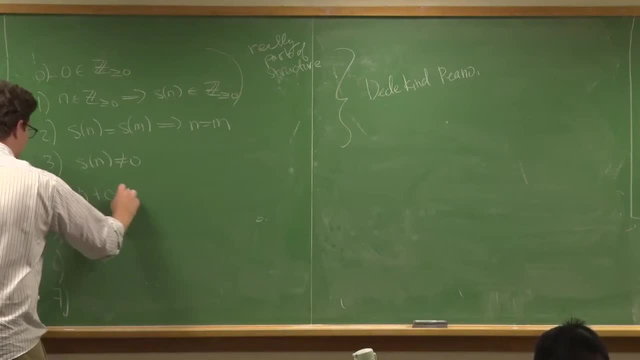 and they're pretty innocuous, right? n plus zero is n for all n, right? the other one says that if you add n and the successor of M, that's the successor of n plus M, so it tells you how successor behaves with respect to addition. and n times zero is equal to zero, so that's. 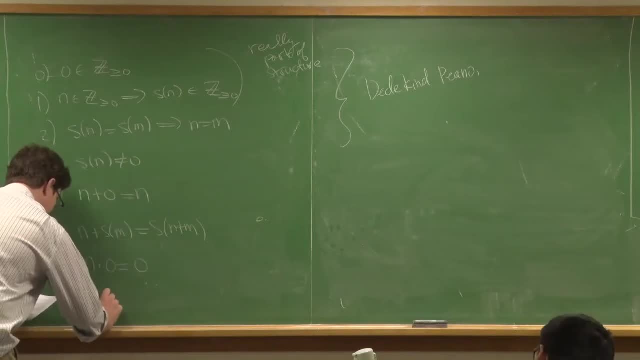 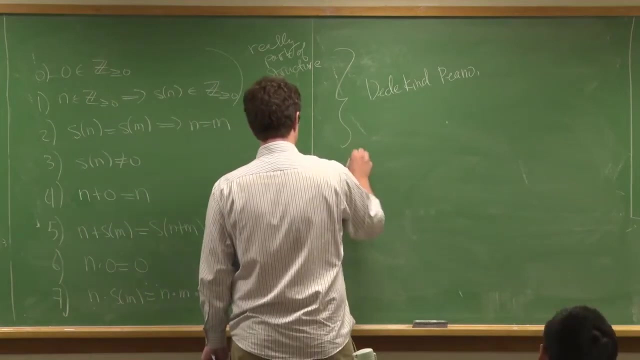 the subordinate rule of n, and that n times the successor of m is equal to n to zero. and that n times the successor of M is equal to n times m times n. okay, and that's like the distributive rule, okay. so these are the axioms here, and then plus the eighth axiom. 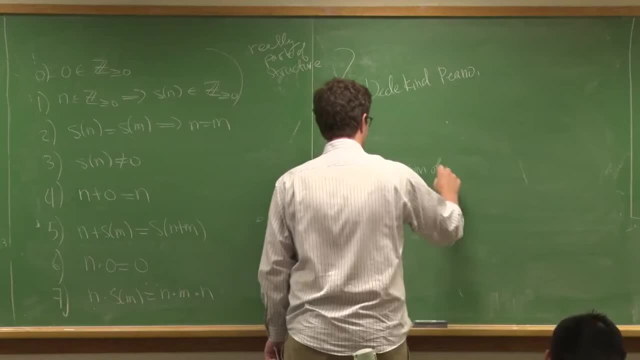 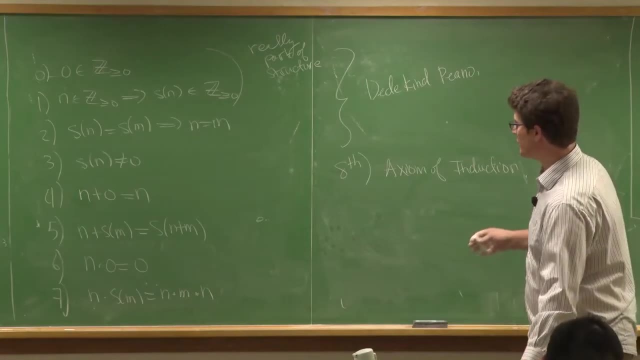 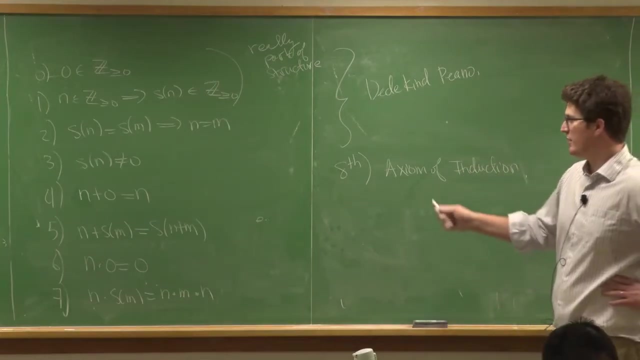 is an axiom of induction, then there's two ways to do this right. there's a first order way and there's a second order way. the first order way is that you could actually add an infinite number of axioms right, instead of adding predicates, and you add, you add it for all formulas with one. 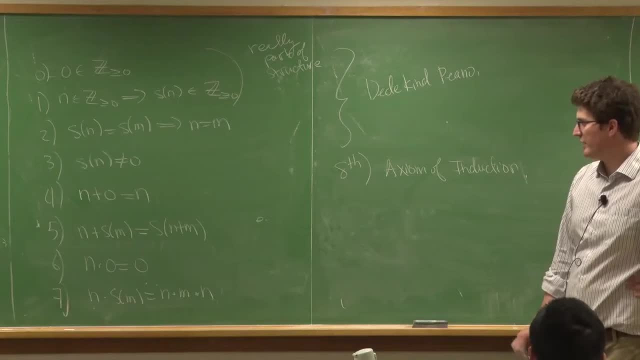 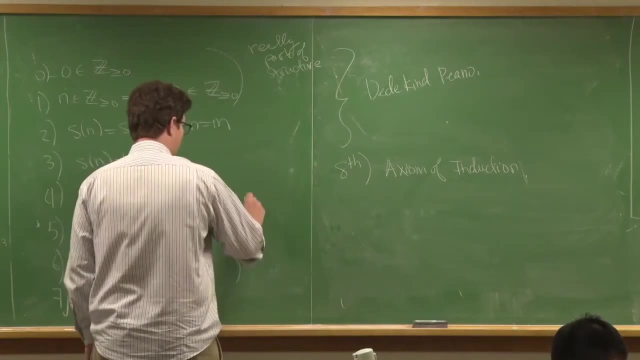 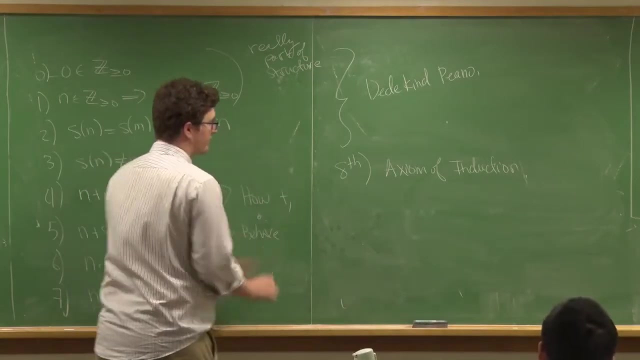 single free variable, right I'm. and the other way to do it is with predicates. so these things here, we just say this here. so this is for how, how, plus in times, behave, and I'm not gonna specify this here. maybe we can talk about this. we want to be more precise. 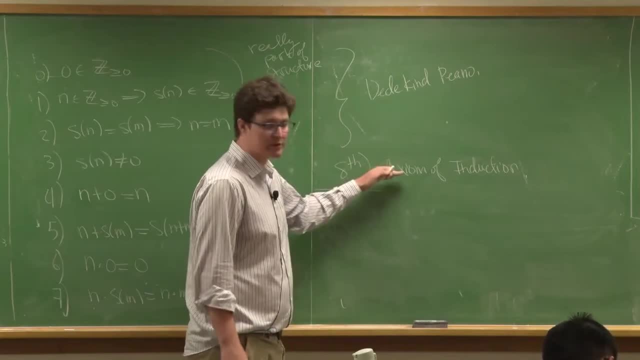 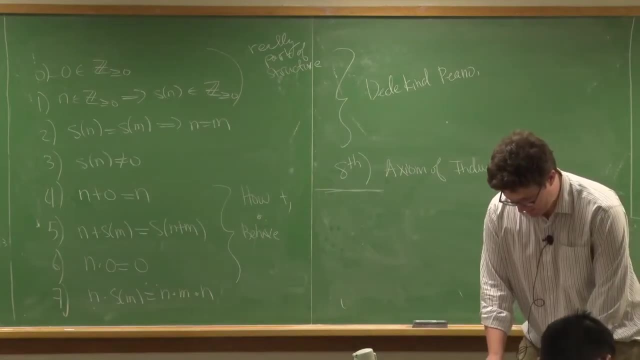 I'm just gonna say there's an axiom of induction that there's a first order way of doing this and the second order way of doing this. it's your, your choice, kinda okay, I'm finally a. the point of this is that using so what's one of the big points is that 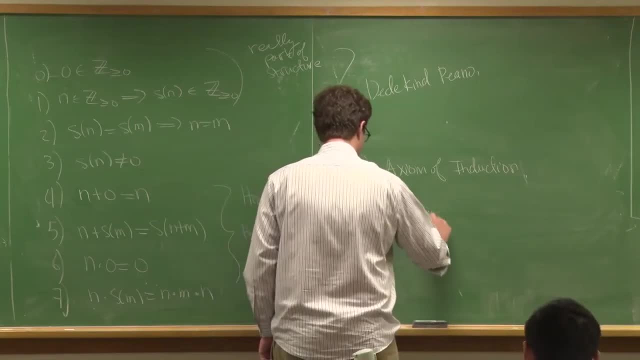 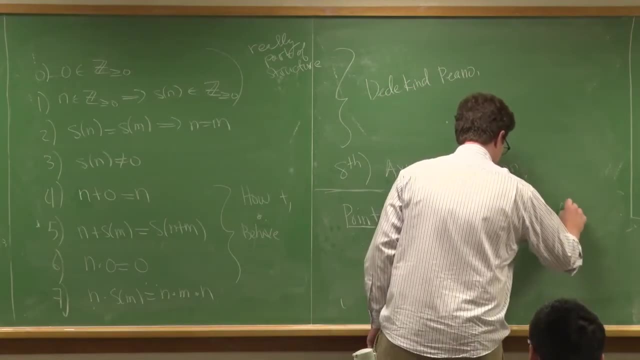 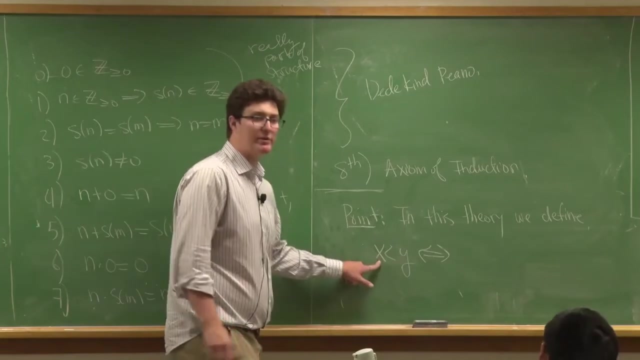 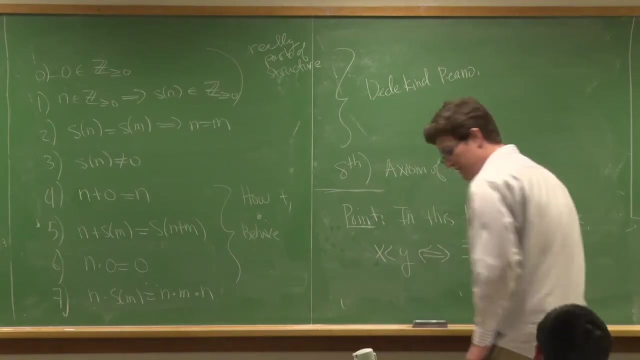 so in this theory we can define the following: X is less than Y. okay, so this is what we really wanted to get at, right, if, and only if, there exists some Z, such that S of Z plus X is equal to Y. okay, so you define. this is by definition. 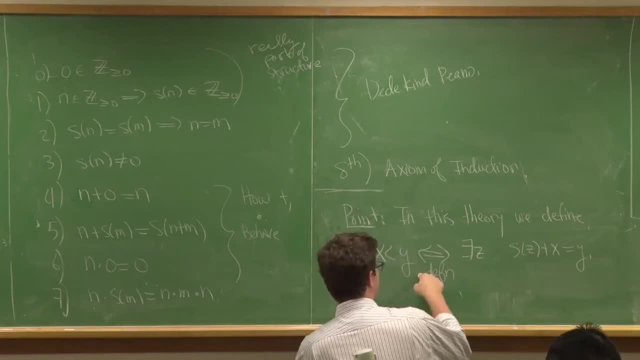 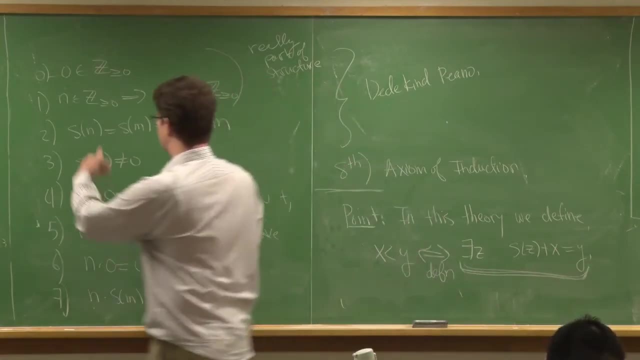 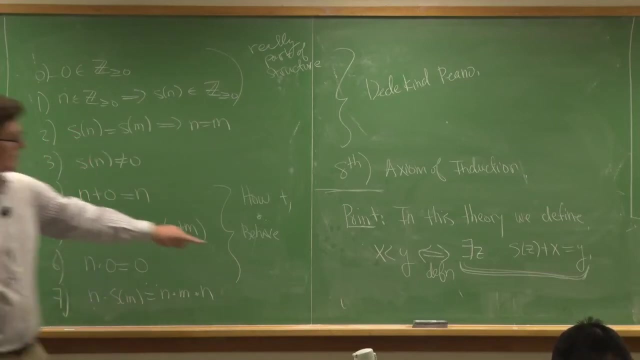 we define the inequality to be this way, and this now is a formula here. right, this is something that we can define using our signature and our, our, our stuff here, okay, so this allows us to define the, the inequality, okay, and so I'll say a little bit more. about this next class.